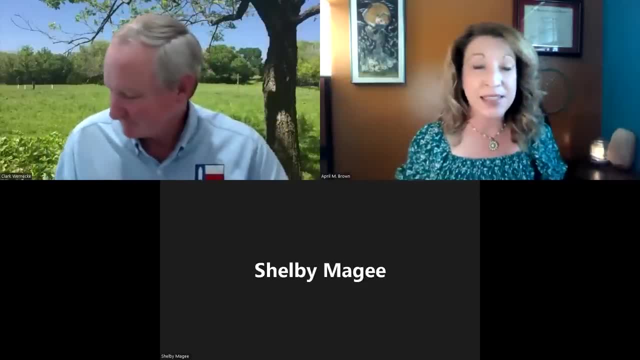 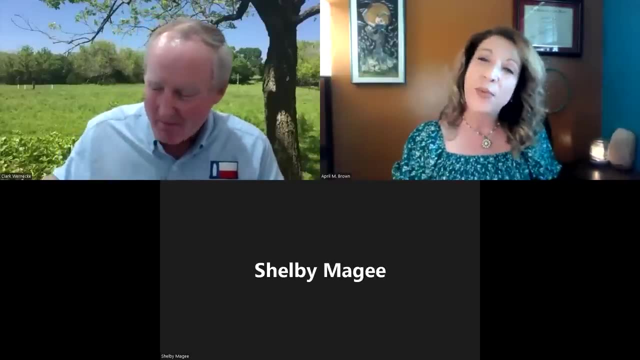 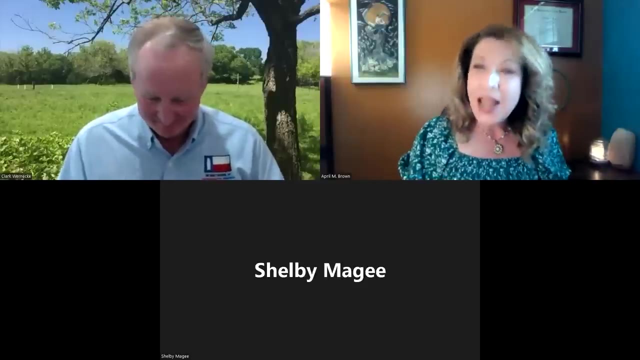 evening is the Executive Director of the Galt School for Archaeological Research, as well as the Project Director for the Prehistory Research Project at the University of Texas Austin, And you probably remember him from his fall lecture The Galt Site and the Peopling of the. 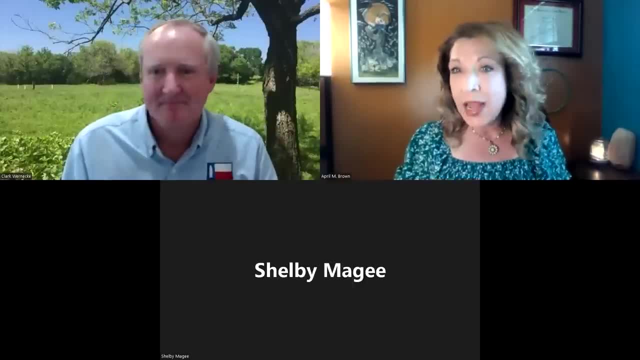 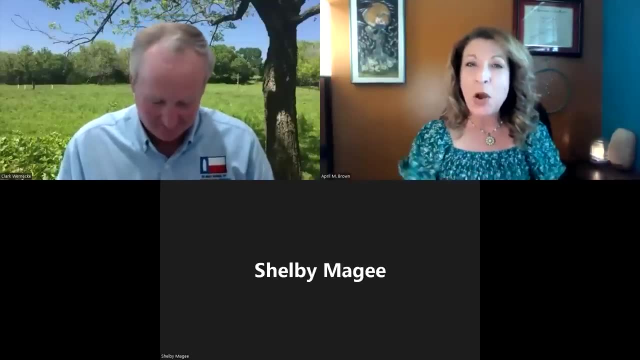 Americas, and he's going to continue on that theme tonight, as he shares an introduction to the American Upper Paleolithic as well as some of the latest research on the topic. So welcome, Dr Wernicke, welcome back. Thank you for coming tonight. Well, thanks for having me again. 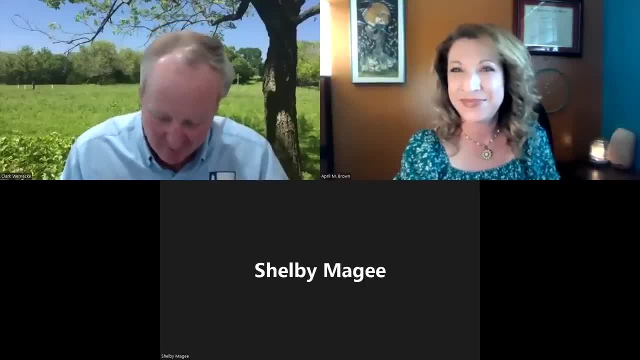 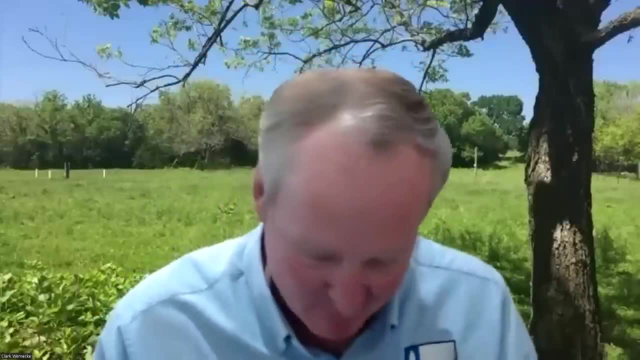 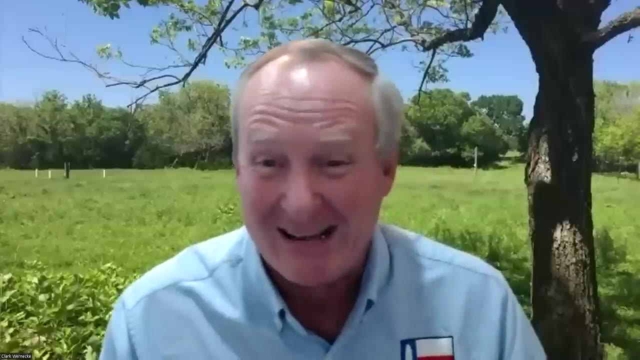 Well, good evening and thanks for all of you for signing in to listen to this talk. Before we get started, I wanted to make one thing really clear: This talk is not a guide for idiots, but rather a guide by an idiot- me. I am a generalist. I have made a career out of organizing 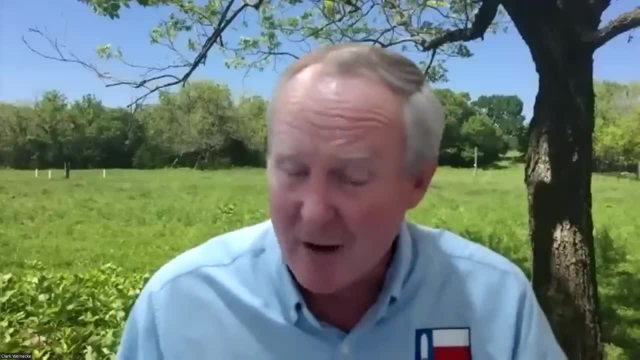 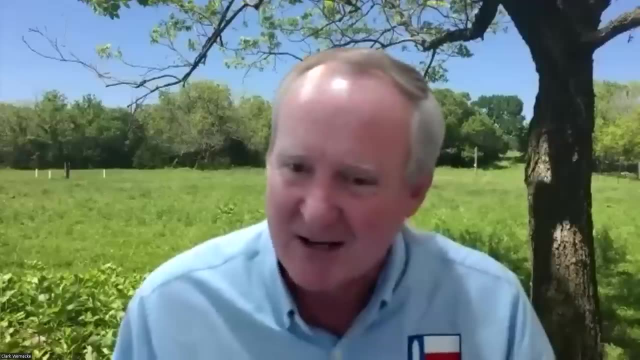 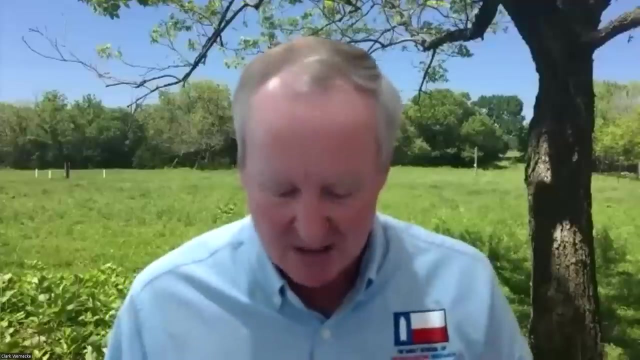 large archaeological projects And while I've helped head up a series of projects looking at archaeology, I'm not a lithic analyst or a geneticist or a linguist or a physical anthropologist. What I'd like to do is give you kind of a layman's overview of the current research into the earliest. 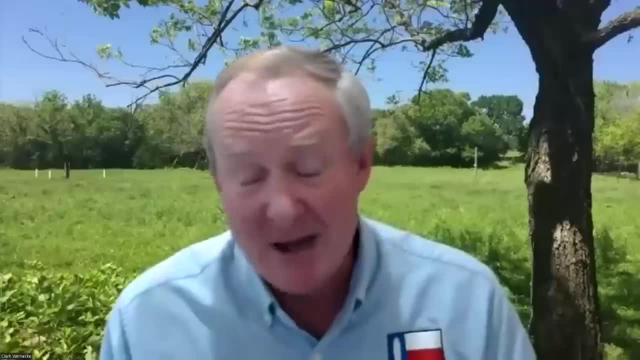 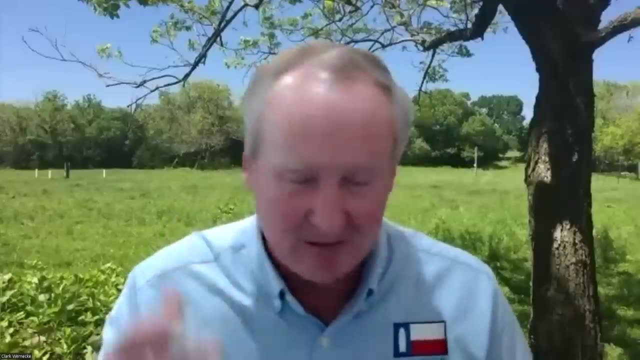 peoples in the Americas. And while I've definitely chosen a side in some of the debates, I'm going to try to present some of the arguments from the critics as well, at least the serious scholarly critiques, To paraphrase Gary Haynes from his book The Early Settlement. 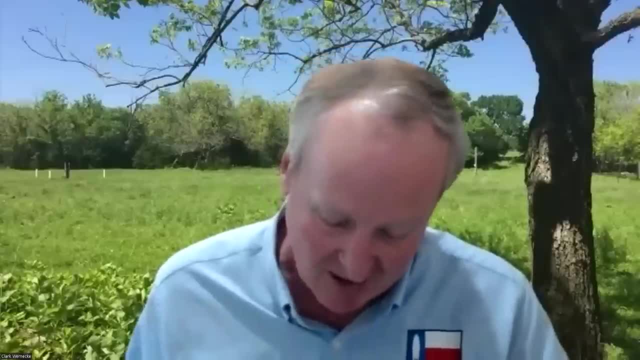 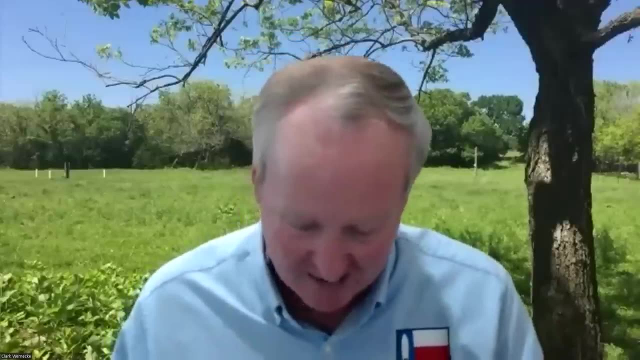 North America. it's impossible to talk about the first settlers in the Americas without offending someone. At the end of my talk I'll be happy to try and answer questions, But keep in mind that I may only have broad answers to some of those questions without technical detail. 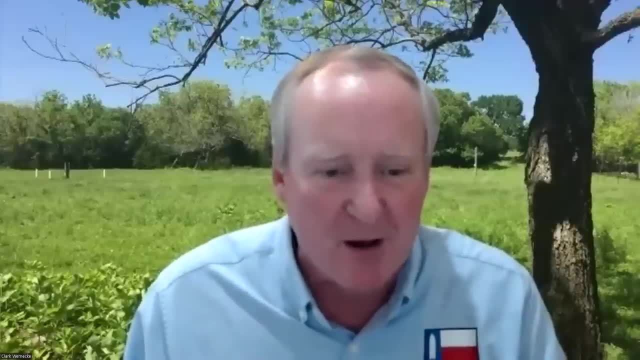 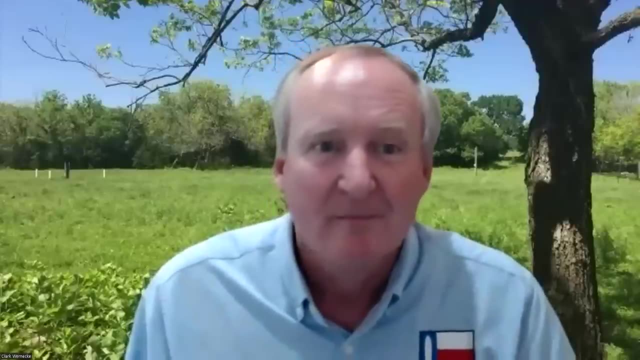 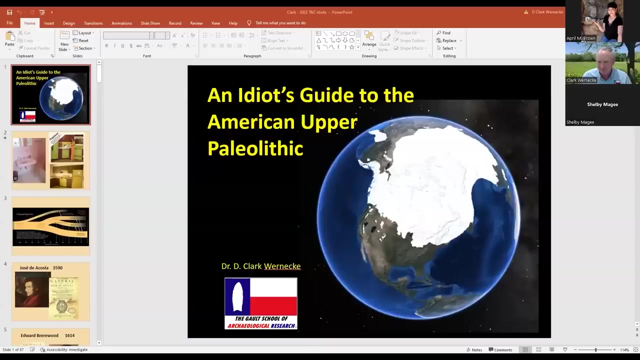 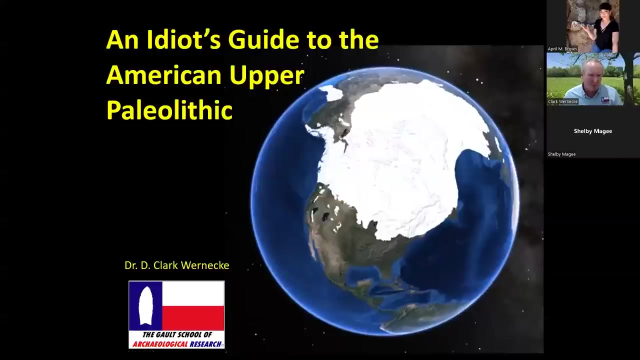 So let me get my PowerPoint up here. There we go. Okay, I want to talk briefly, before I get into the slides, about the term Upper Paleolithic. Upper Paleolithic is a term that's used in the rest of the world regarding the period roughly. 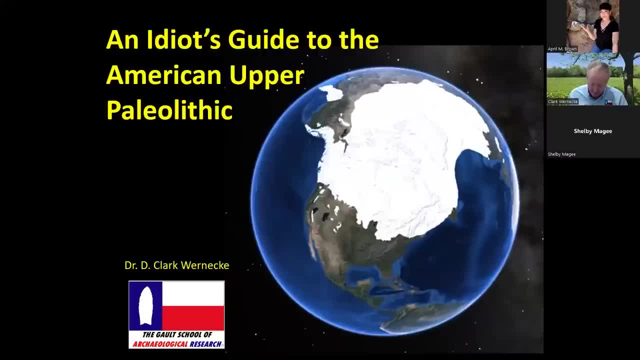 from 50,000 years ago until about 12,000 years ago. American archaeologists, for reasons I've never understood, have resisted bringing our nomenclature in line with the rest of the world. No one's arguing that the first peoples in the 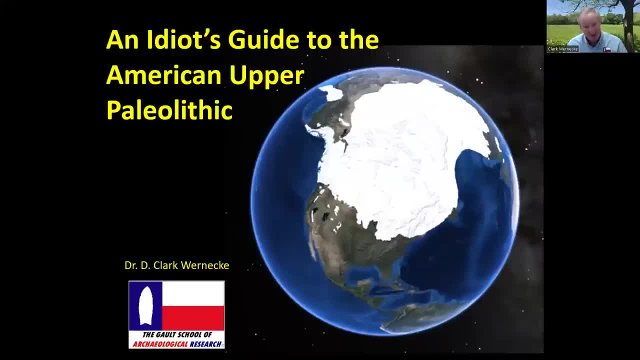 New World didn't come from the Old World during the Upper Paleolithic period, But we've stubbornly stuck to our own terms For a long time. we thought that people arrived in the Americas only about 4,000 years ago. In 1940, Frank Robert first used the term Paleo-Indian, though only in a very 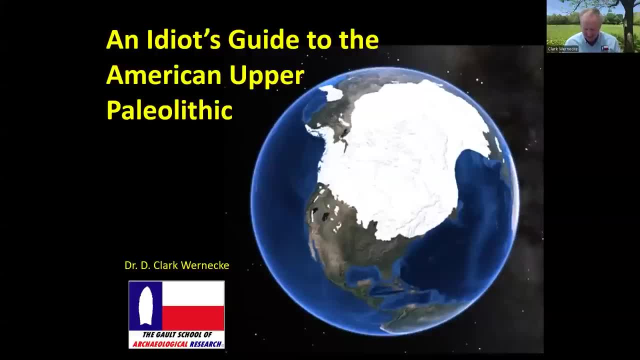 general sense, And by the 1950s, archaeologists were beginning to define a Paleo-Indian time period, usually divided into an early period, including Clovis and Folsom cultures, and a later period, With more and more sites showing evidence of people here prior to the early Paleo-Indian. 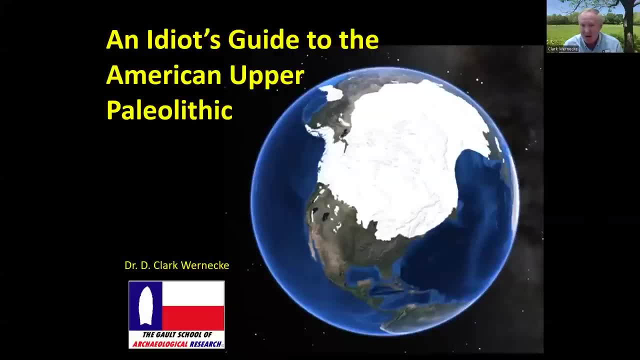 period, we run into a problem. Some speak of pre-Clovis or older than Clovis, But this puts an emphasis on Clovis. that's not justified, as if everything earlier must be measured against Clovis, But if Clovis is not the first recognizable culture in the Americas. 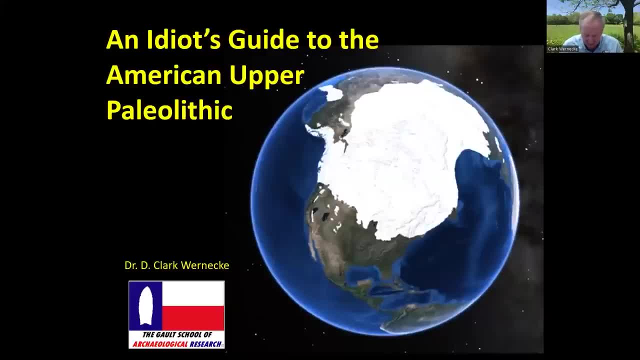 then it is no more important than the cultures that followed it. It's not a gold standard. Since Clovis and Folsom are regarded as early Paleo-Indian — what do you call anything earlier Early, early Paleo-Indian, Pre-early Paleo-Indian? So that's why I'll call this the American Upper. 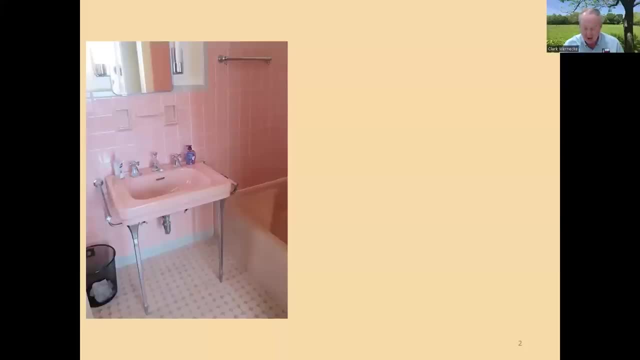 Paleolithic. Jim Collins, Andrew Wilson, Mike Riles, Jim Collins, Jim Collins. talk a little bit about terminology before we wade into this topic. First, I'd like to emphasize that, with rare exceptions, archaeologists are looking at technology things rather than people. 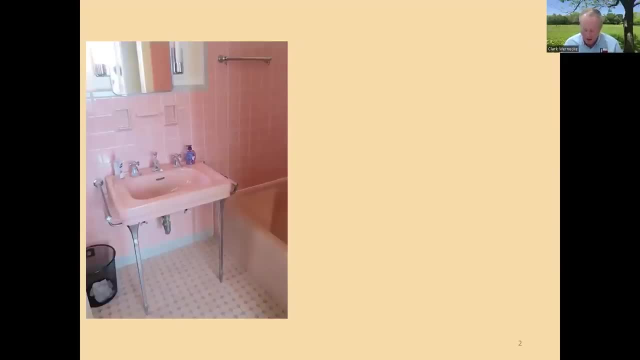 It's what we do. We basically look at garbage to figure out past human behavior. There's not much difference to us, except perhaps smell, between new garbage and old garbage. Now, if you go into a house and the kitchen and baths are black and white and pink, 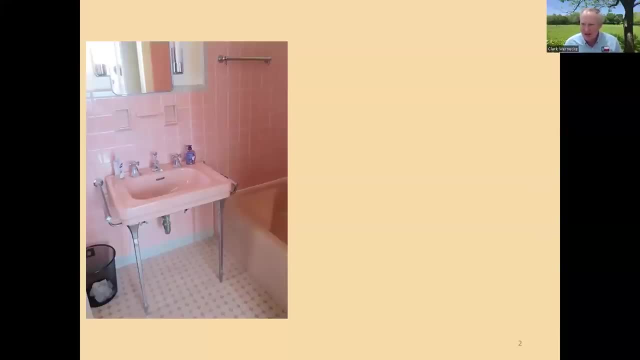 how old is it? Some of you remember it's going to be late 50s, early 60s, And you might remember after that turquoise, avocado, harvest, gold, poppy, red, black, almond, white, stainless steel. 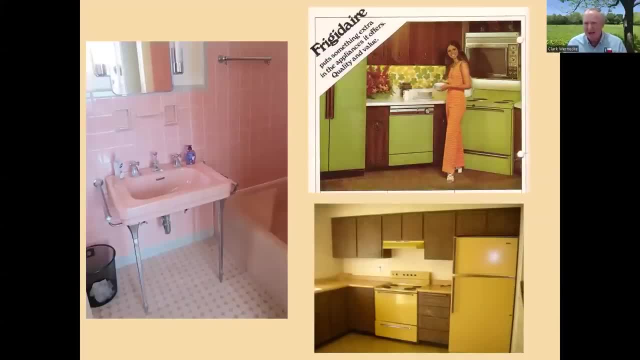 Nobody ever asks me what happened to the avocado people. You know who you are. They became the harvesters gold people for the most part. but we get asked all the time whatever happened to the Clovis people. The short answer is: there is no such thing. There is a Clovis technology, but we have 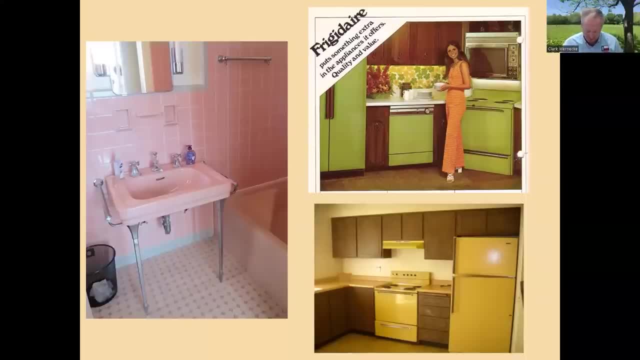 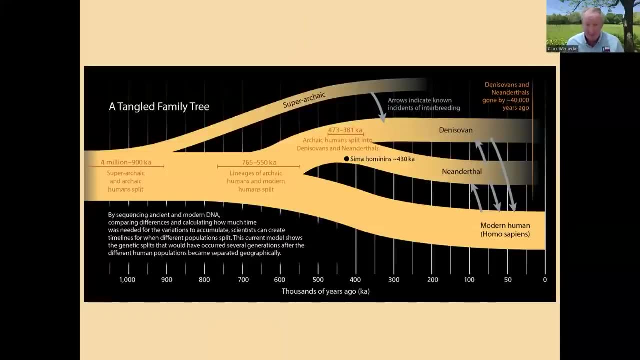 little idea what people or peoples used it. All the people we're going to be talking about tonight, all the people we're talking about in the new world, are modern humans, homo sapiens, just like us. Collectively, they're not any dumber or more primitive than all of us here tonight. 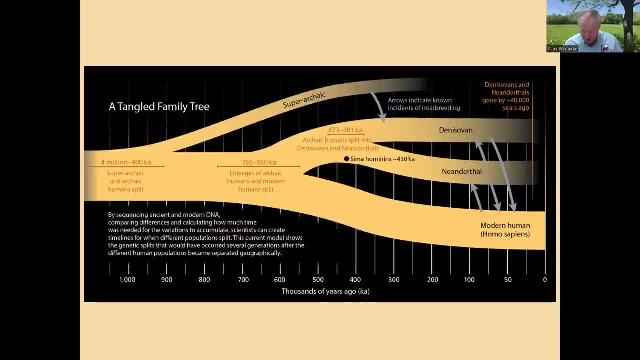 Current scientific data points to modern humans' origin in Africa, followed by out-migration. Humans were thought to have gotten to Europe around 50,000 years ago, for instance. That is, until the publication of data from Apodoma Cave in Greece with the oldest modern. 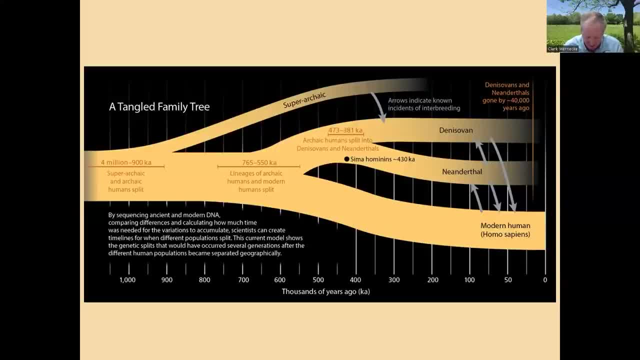 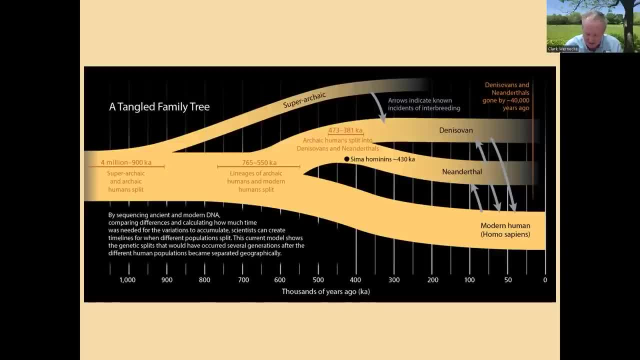 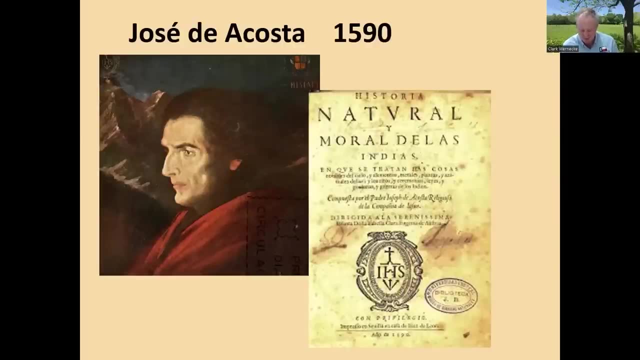 It's based on the best current data and our hypotheses. the ideas of what occurred in the past change as new data is found. Our story of the people of the Americas starts with a Jesuit priest, Jose de Acosta, in 1590.. Jose had spent 15 years in the new world in South and Central. 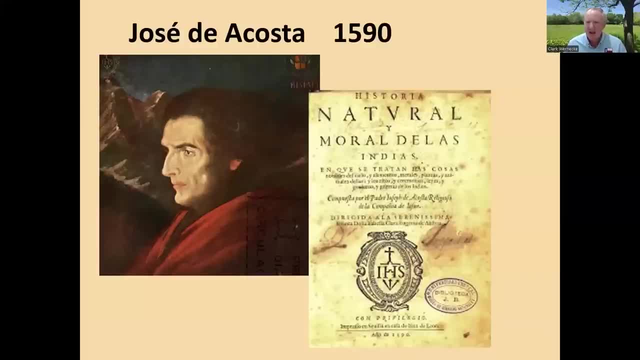 America and he wrote about his experiences in a book, The Natural and Moral History of the Indies. The book became the bestseller of the day. People were very curious about the new world and it was translated and printed widely And in it he speculated on where the people in the 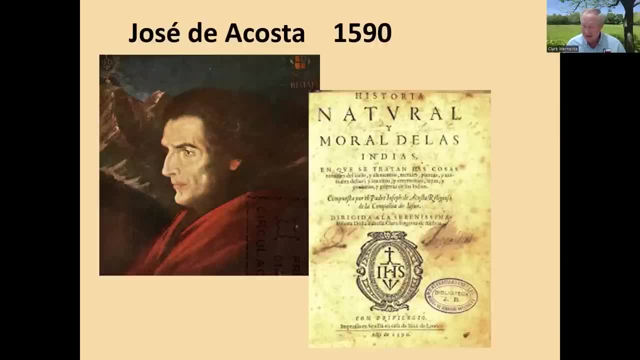 new world had come from. First he knew, as a priest, that all humans were descended from Noah and his family in Central Asia, so they must have come from there. He looked at whether they'd come by land or sea, and he decided that people were too primitive. His major argument was they lacked. 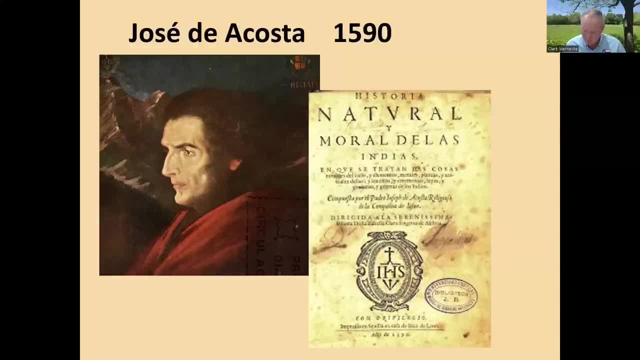 them. He looked at whether they'd come by land or sea and he decided that people were too primitive The compass to have come by boat. He also noted that the new world had some old world animals, especially wolves, that he noted, And since only an idiot would put a wolf in a boat, 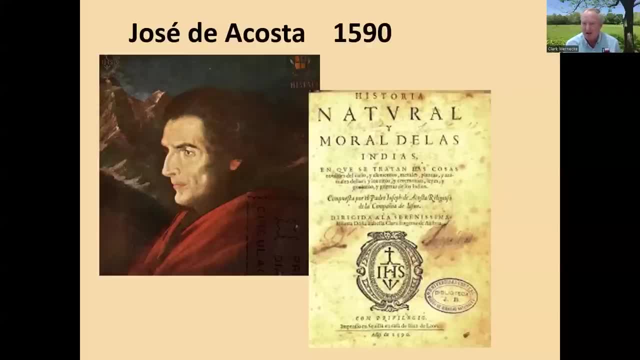 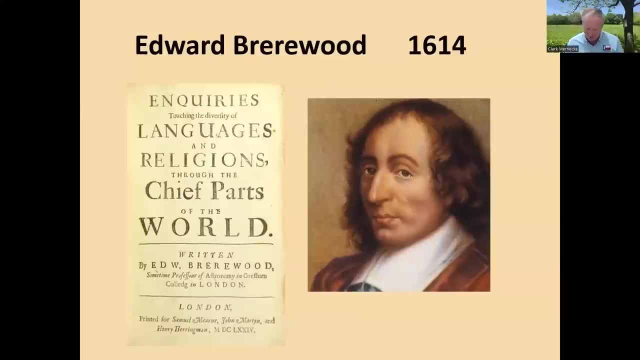 Jose decided that humans and animals must have walked here somehow. In 1614, Edward Brerowicz's work on languages reinforced this idea. His book was actually published posthumously by his son, But it was still being quoted a century later. A number of popular writers at the time had been: 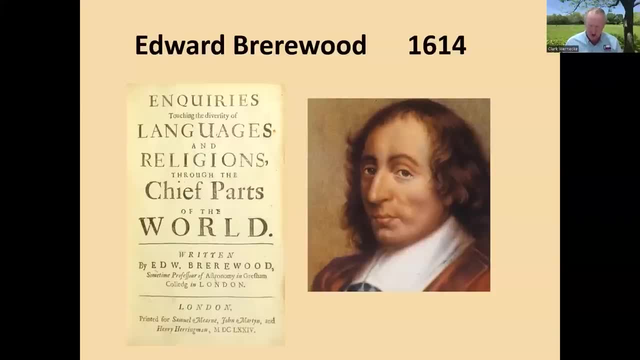 tossing out the idea that Native Americans were descended to the lost tribes of Israel or Phoenicians or they had a lot of theories like that, a lot of hypotheses, And Brerowicz's work discounted this notion. He thought they were more likely related to the Tartars of Crimea. 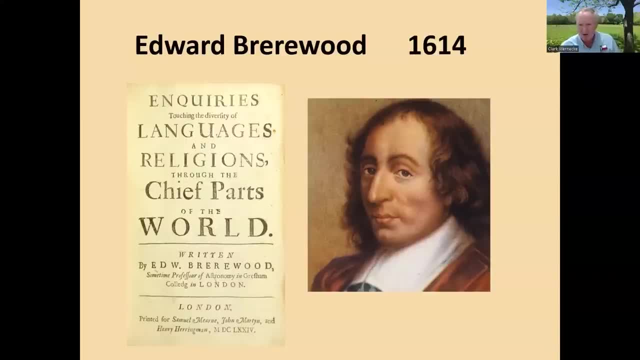 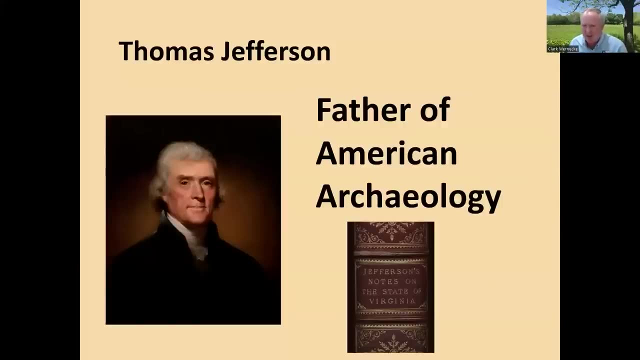 making them of Asian ancestry. So that pretty much takes us up to this guy, Thomas Jefferson. You might recognize him. who we're in regard is the father of American archaeology In the 1780s. in response to a questionnaire from: 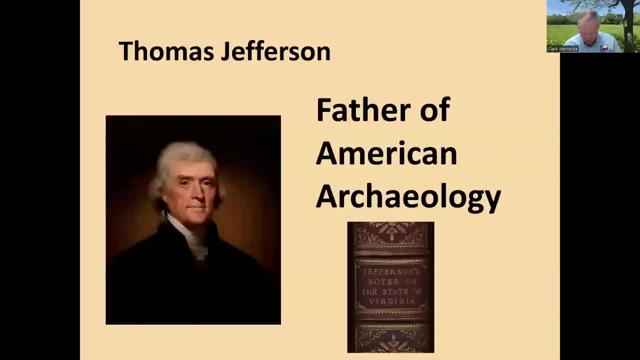 France. he wrote a book, Jefferson's Notes- on the State of Virginia, And one of the things he did was scientifically excavate a burial mound near his home, recording the various strata that he discovered, the various layers of this mound, And in this book he actually speculated on the 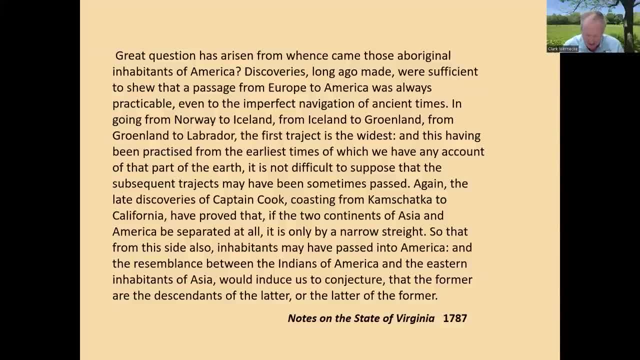 origin of the inhabitants of the Americas. He concluded that, well one, there was really no problem with people getting here by boat. He also concluded there was really no problem with them getting here from Europe. He also thought that there was probably little or no distance between the continents of Asia. 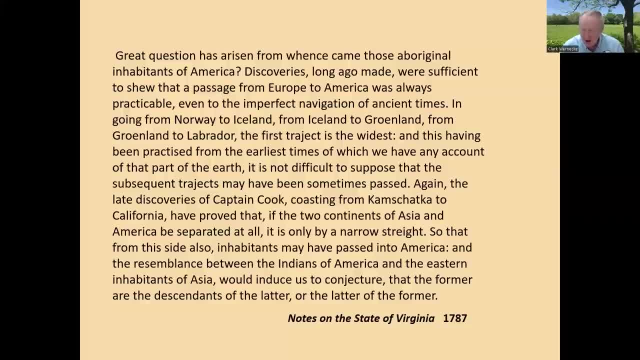 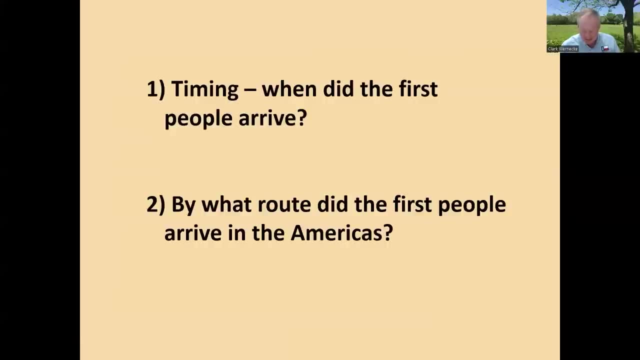 and North America, And he also decided that there seemed to be a resemblance between Native Americans and those in Northeast Asia, which a study of language might clarify, But he's definitely a bit of a connoisseur of the history of the Victorians and the Balkans. 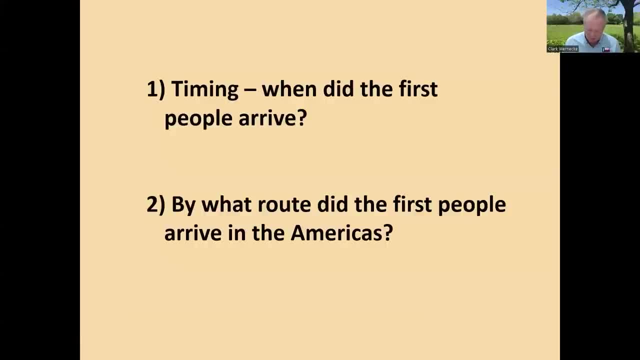 And he also concluded that there seemed to be a resemblance between the continents of Asia and the Balkans, And he also concluded that the continents were not only the regions of the Mediterranean but the regions of the Atlantic Ocean. In other words, there was a lot of. 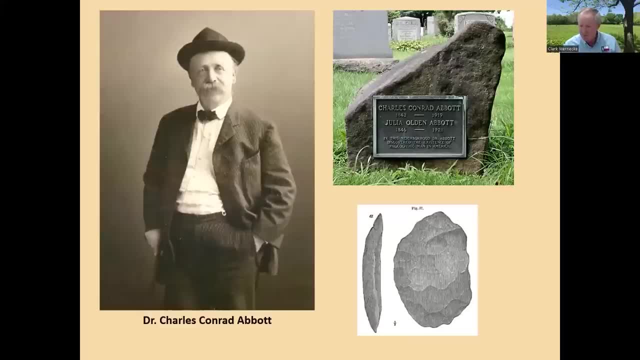 information, but not enough to be found to prove that the continents were made up of the same ancient sources. So he concluded that the continents were the origins of the Atlantic Ocean. So yeah, there's a lot to be said here. I'll put it in the description. 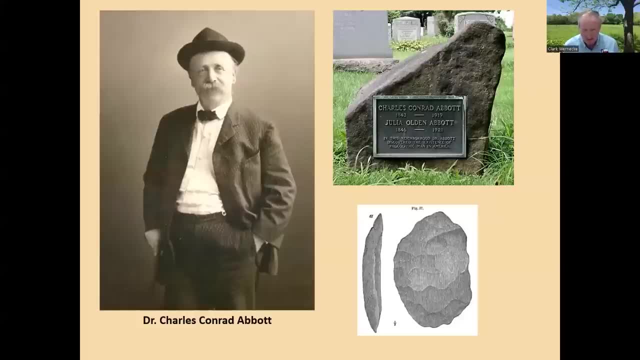 tools coming out of gravels in France and was also filled with a little bit of nationalist zeal and he was convinced he had the same thing in the river gravels of the Delaware Valley. William Henry Holmes of the Smithsonian basically ripped his head off, saying he was equating. 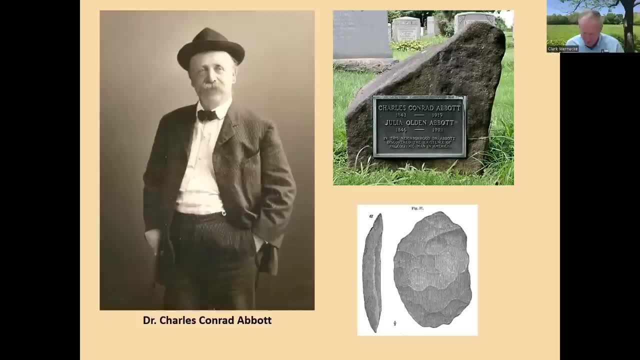 primitive with old. The head of the Peabody Museum at Harvard was intrigued enough to send an archaeologist, Ernest Foulkes, who worked with Abbott for 20 years, also basically concluding that the tools he was finding were not that old. But Holmes wasn't alone in this attitude towards. 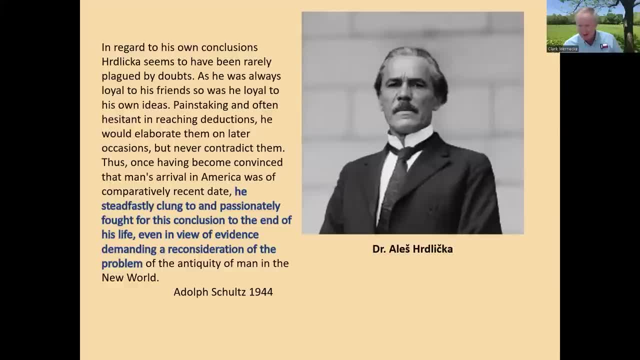 researchers, professional or amateur. His colleague at the Smithsonian, Dr Alice Sherdlitschka, often attacked any idea that man in the New World was older than 4,000 years. This quote is actually from an official biography of Mendes' death by one of his friends. 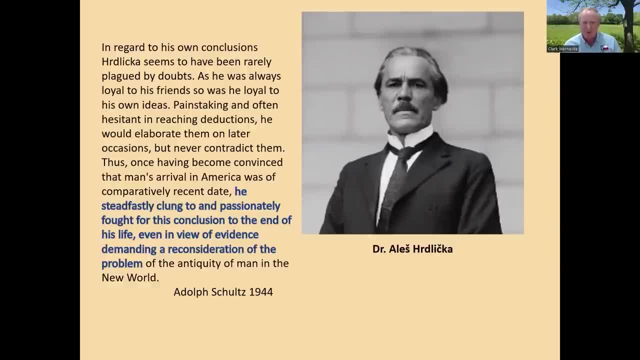 and even his friends say he steadfastly clung to and passionately fought for this conclusion to the end of his life, even in view of evidence demanding a reconsideration of the problem. Sherdlitschka and other conservative researchers were powerful checks on anyone who speculated. 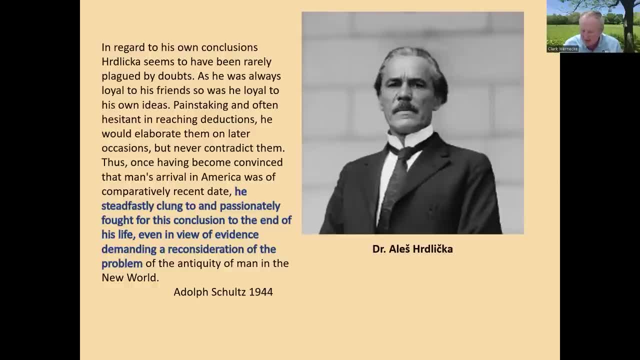 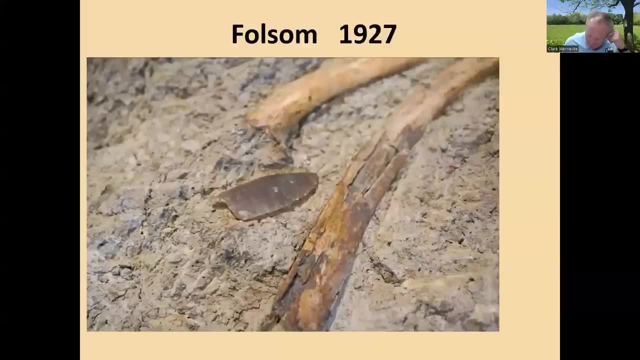 about anything older. They controlled basically the journals and the jobs. In 1927, Frank Hibben from the Denver Museum found stone projectile points in association with bison known to have become extinct by 10,000 years ago near Folsom, New Mexico. He left them in situ. 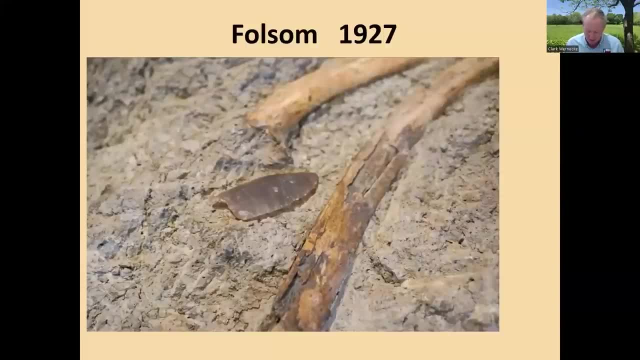 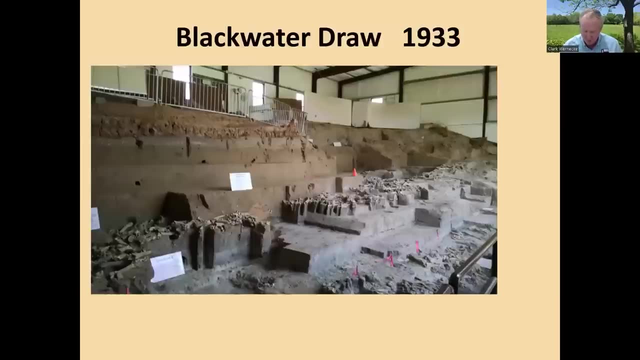 in place and had other researchers come and take a look, And they agreed that the find was scientifically valid. Later, Edgar Howard, working in Blackwater Draw near Clovis, New Mexico, found what he called cruder projectile points, which remains of mammoth, horse and bison. 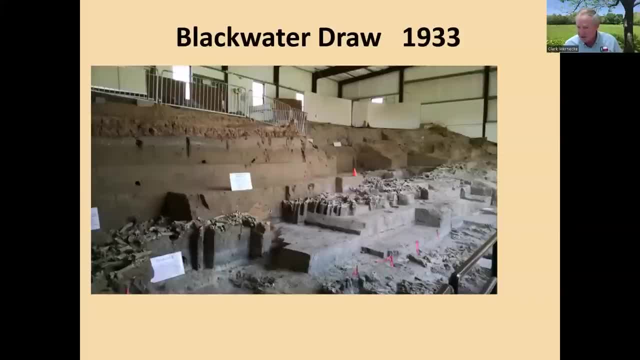 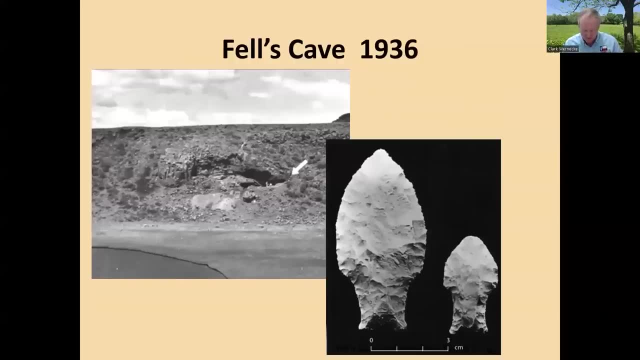 Blackwater Draw is the type site for the Clovis culture, which was later determined to be older than Folsom. And in 1936,- whoops, skip ahead here a little. and in 1936, Junius Byrd. 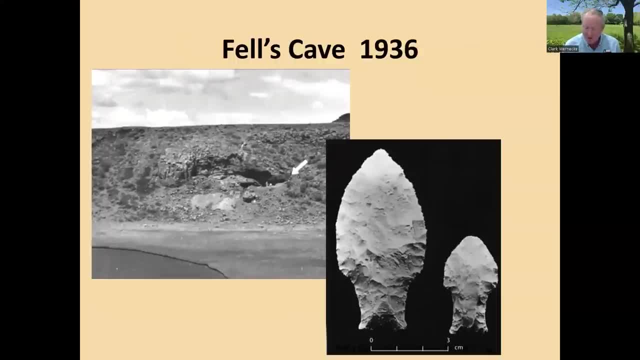 working in Southern Chile found what are now called fishtail points in association with extinct horse. I want to emphasize that these fishtail points are similar in age to the Clovis culture in the North. We'll come back to that later. There was now no doubt that people were in the 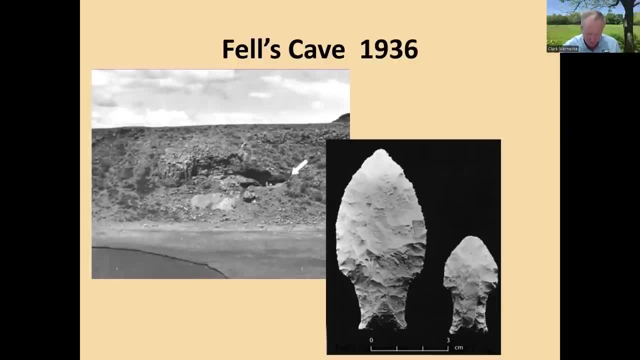 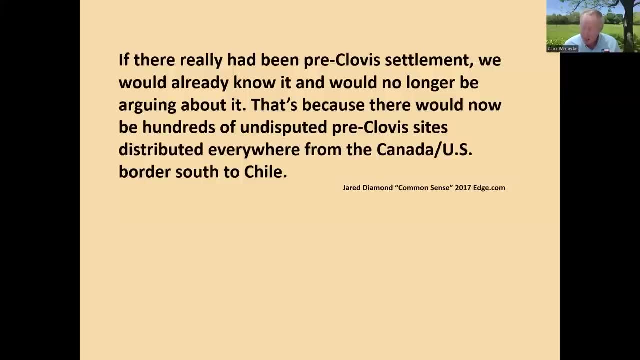 New World prior to 10,000 years. In recent years, very vocal critics have taken up Alisher Glitchka's crusade to block further scientific inquiry. In this case, a Pulitzer Prize-winning author who apparently understands neither the incremental nature of science nor archaeology, thought it worthwhile to comment on. 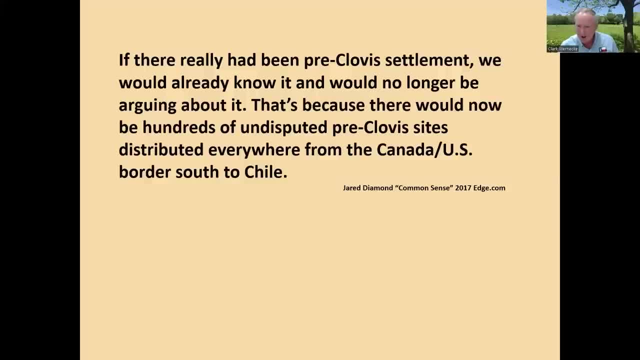 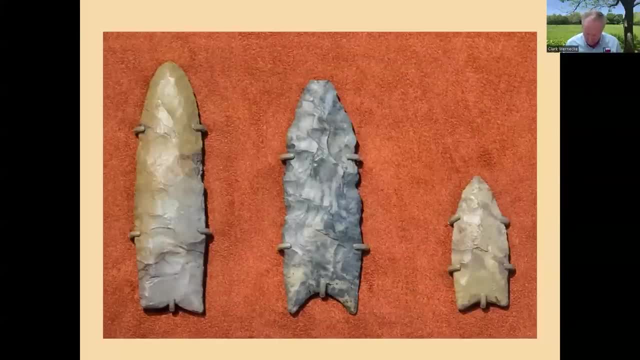 Not only is this statement a logical fallacy, but it also ignores the data. In 1806,, Meriwether Lewis and William Clark- you might have heard of Lewis and Clark vaguely- found these Clovis points at Big Bone Lick, Kentucky. The Clovis culture was not defined until nearly 150 years later because they didn't. 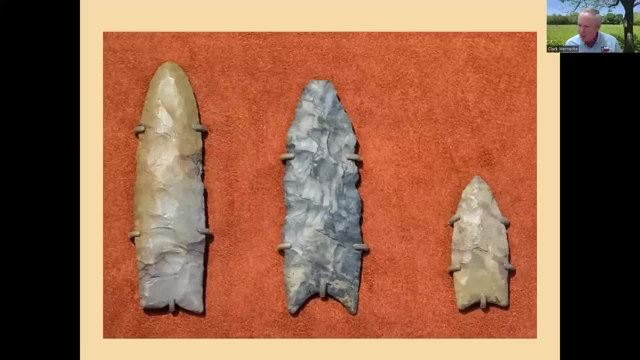 have good context for the points and they had no way to properly date material at the time. Context is everything. Clovis materials were found for hundreds of years prior to the definition of Clovis, just like older materials, Clovis materials were found for hundreds of years prior to the. 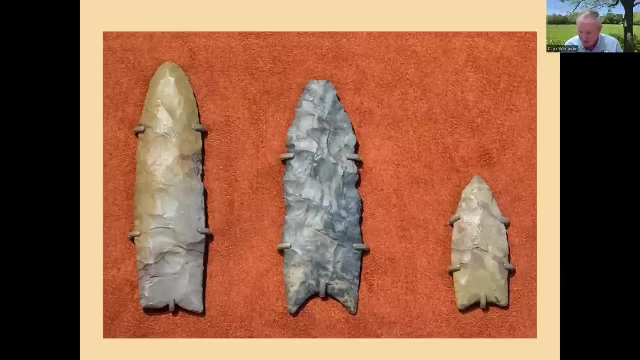 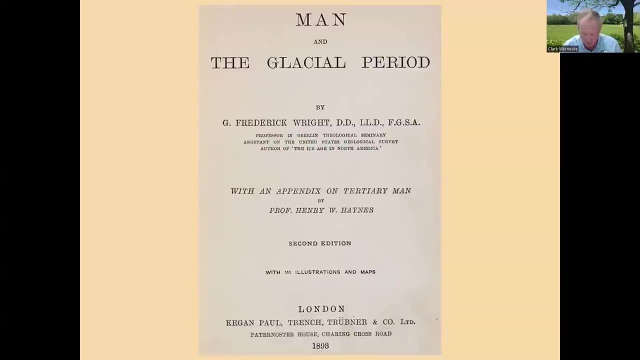 definition of Clovis. Clovis materials have undoubtedly been found for those same years, without context, Not that there wasn't early dissent. Frederick Wright published Man in the Glacial Period in 1892, speculating about earlier dates. Alex Krieger, in 1964, published lists of 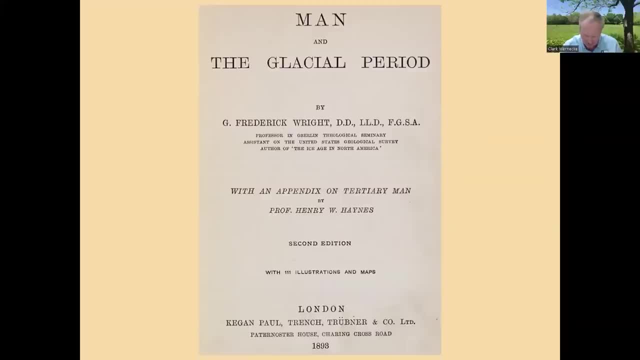 sites in both North and South America. he thought might be older, in a book, Prehistoric Man in the New World. There was scant evidence at the time, but the data in hand seemed to point, however, toward an earlier process. but we needed a lot more work on it. 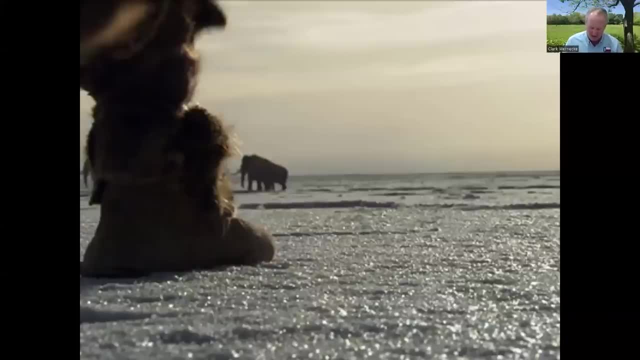 After the finds at Clovis Folsom and Fells Cave, the story of the peopling of the Americas changed from that of people coming here 4,000 years ago to people coming 13,500 years ago. And this story, like the one before it, became institutionalized for all purposes, set in stone. 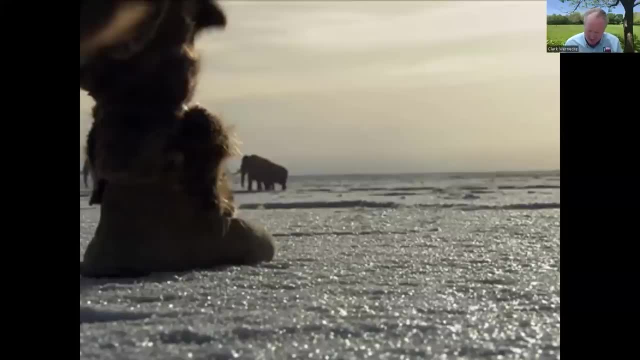 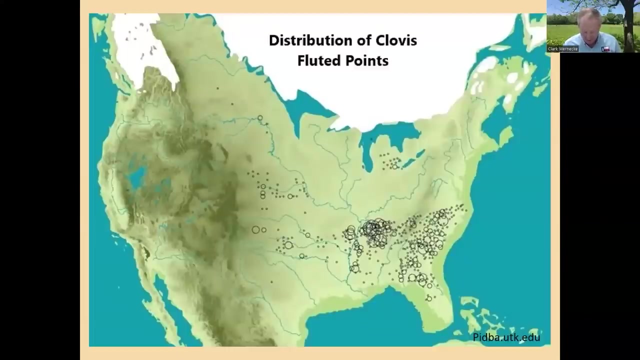 and we taught it to our elementary school children and we still it to our elementary school children. Clovis represented the first people in the New World, But there's always been a problem with that hypothesis. This is by far not a complete map of the current data, but even so it shows some tendencies. 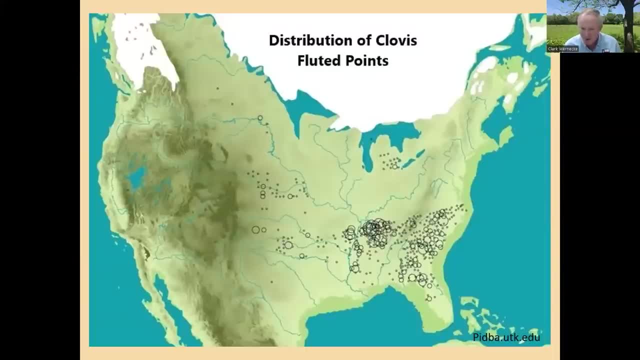 This is a find of Clovis fluted points in the United States, And it certainly looks like Clovis, rather than starting in the Northeast and making its way to the Southeast, spread into in the opposite direction. Coupled with that is that researchers have been unable to find anything. 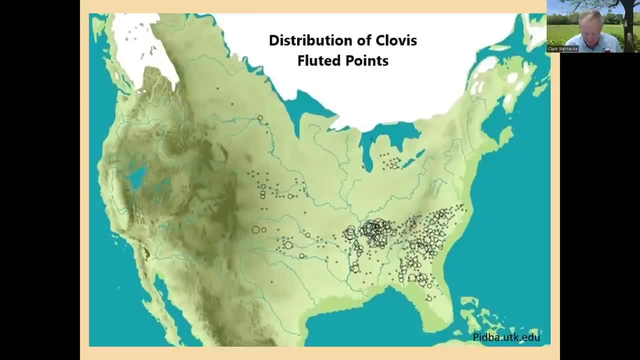 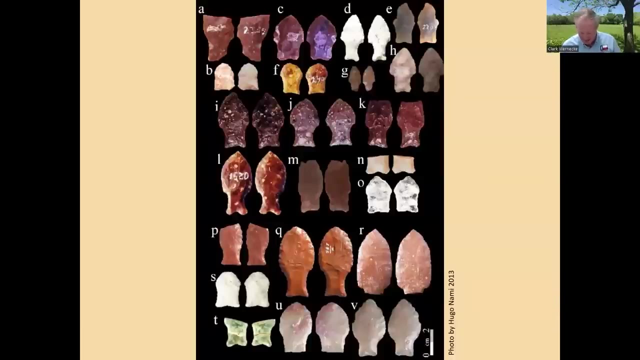 like Clovis technology in Siberia. In fact, it looks as if fluted-point technologies made it back that way from the Americas to Siberia about 12,000 years ago, going the other direction. There was also a propensity in North America to ignore any data from South America. Those pesky fishtail points first found by Junius Byrd seem to have dates comparable to Clovis. If you have cultures in South America and cultures in North America with the same dating, neither of those are likely to be first. There's probably a precursor to both of them. 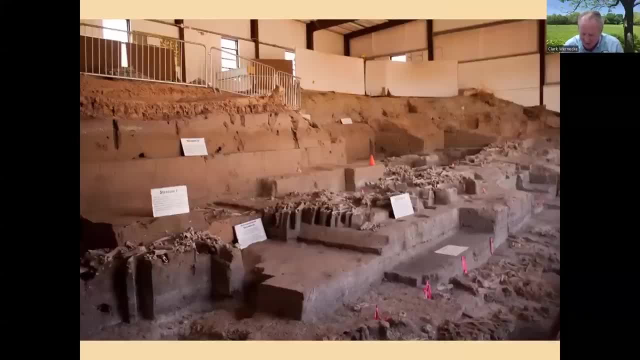 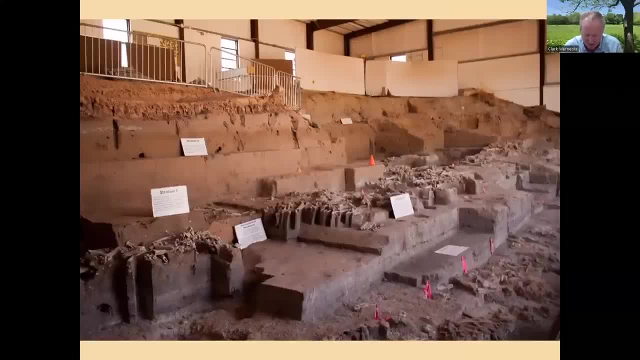 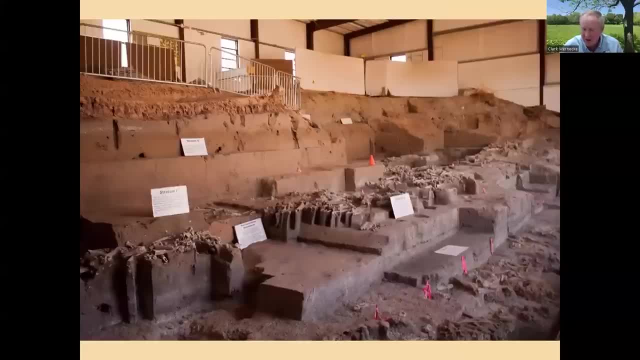 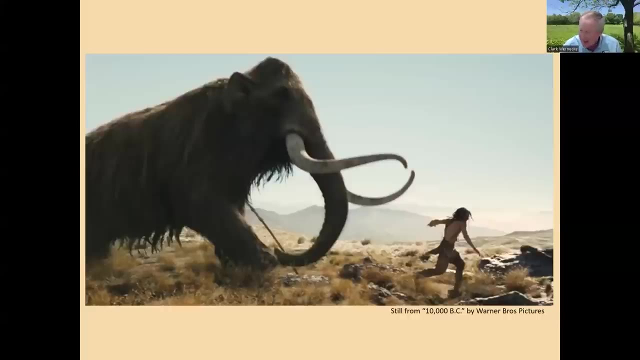 became the type specimens for what was initially called the Lano Complex. Finally, there was some context to Lewis and Clark's find from 1806.. The definitive find of human-made artifacts with extinct animals at Folsom in 1926 and later at Blackwater Draw. 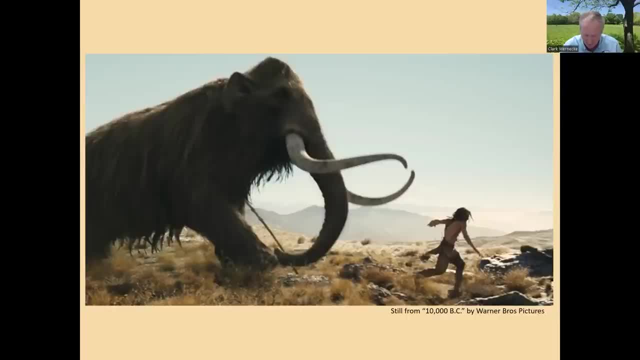 proved that humans were in the New World prior to 10,000 years ago. Even though there were researchers who thought that people had been here much earlier, there was a lack of definitive proof. The story taught to most of you as children, and still taught to many, was that Clovis technology. 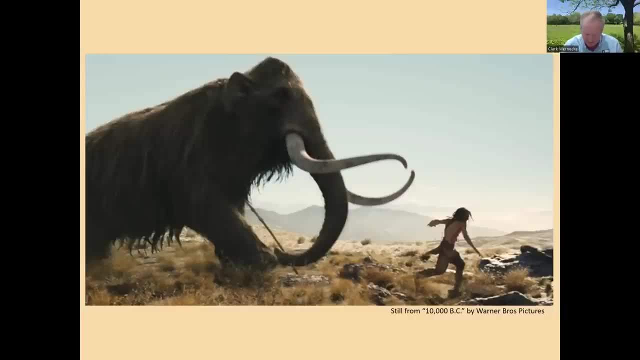 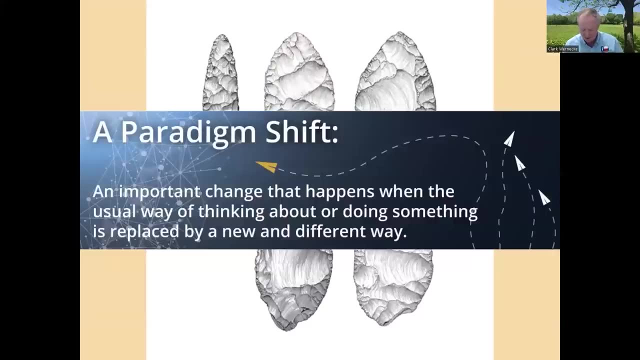 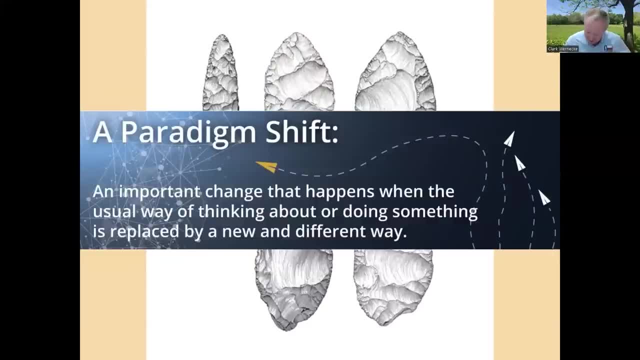 We may or may not be in another paradigm shift, just like the one that happened when we decided the 4,000-year-old date didn't fit the data. That shift wasn't instantaneous. Herdlitschka and others went to their graves arguing against it. Science, however, advances through consensus, as even 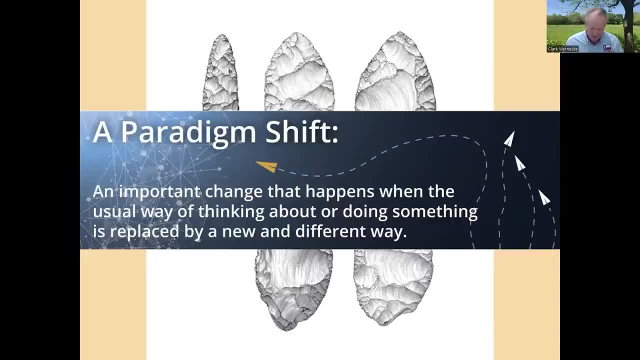 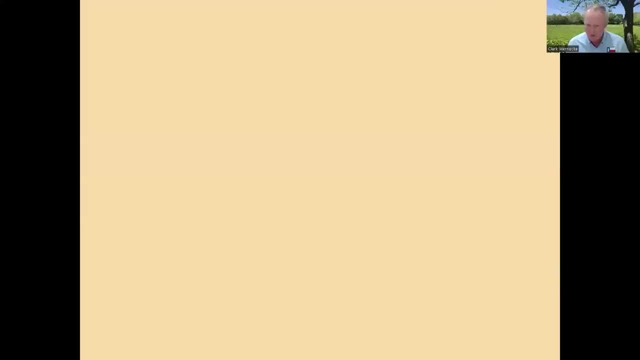 Herdlitschka's friend Schultz recognized in his obituary: When enough data exists for consensus, science changes with it. So what kind of data currently exists? Well, okay, If we're going to look at some archaeological sites, then we're going to. 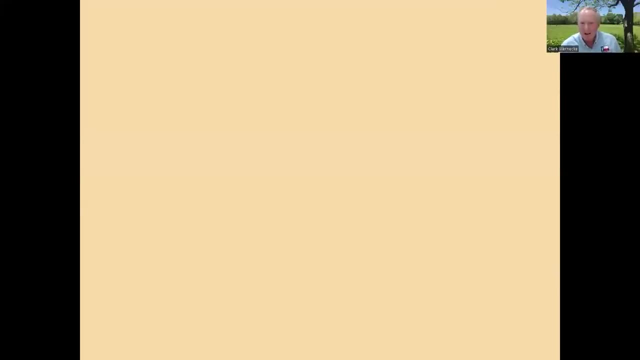 need to discuss something really important: The rules of evidence. What constitutes proof to other scientists that you have what you claim to have: Human-made artifacts, ideally ones that no one can doubt or quibble about? Good geology and stratigraphy Demonstrating that the archaeological materials are where they are for good reason? 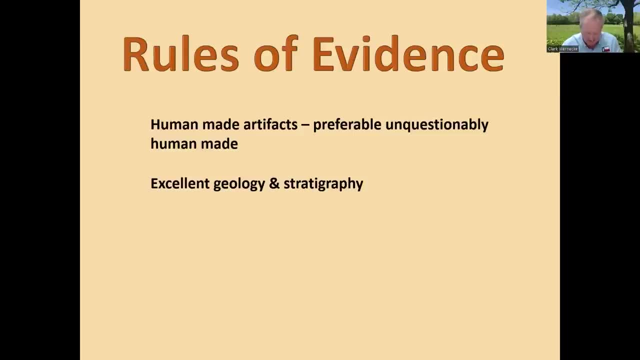 and where they should be for the rest of the evidence to make sense. Good context, Not just the place, but from what soil, what strata found? with what else? Context is everything. Think of archaeologists as CSI, prehistoric. We all know removing or missing one artifact from a murder scene can change everything. 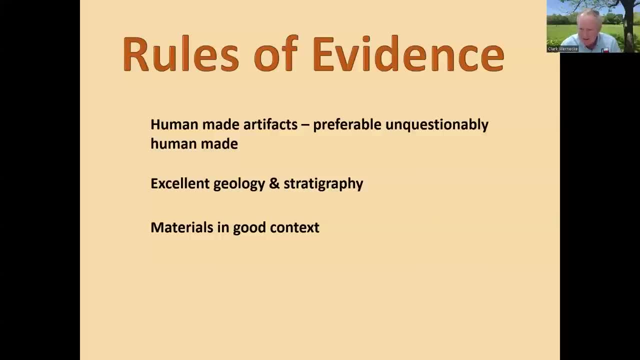 The same is true in archaeology. You need everything, exactly with everything else in good context. And lastly, we need good scientific dates. Generally, when we're talking about this, we mean absolute calendar dates and not relative dates, Preferably a large number. 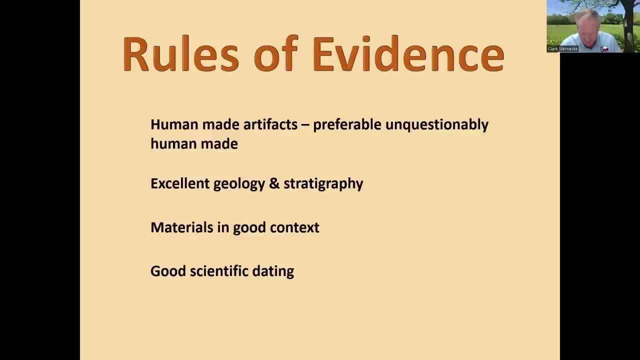 and, if possible, from a variety of techniques and labs. The best case is that calendar dates and the relative dates of materials from the surface down coincide to show a well-dated site. Okay, so that brings us to some data, And in this case we're going to start with Monteverde. 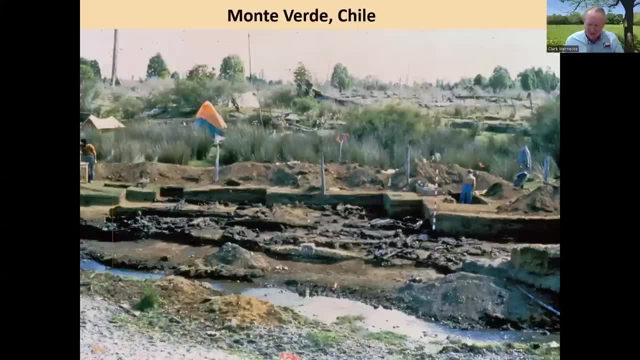 It wasn't the first find of older material but it was the first to get a consensus. Monteverde is near Puerto Montchile, near the south end of the western hemisphere, way down near the pointy bit. The site itself was found in 1975, and excavations led by Dr 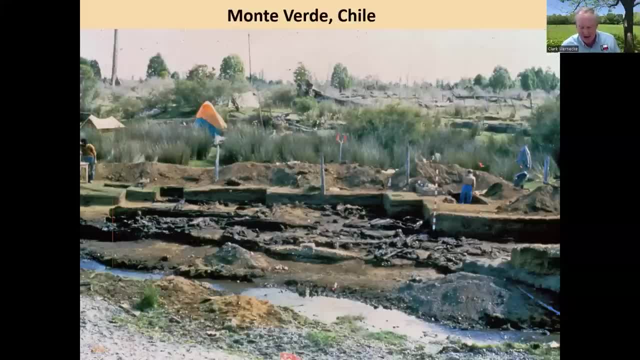 Tom Dillehay of Vanderbilt University began at the site in 1977.. Prior to publication of the archaeology, Dillehay arranged a site visit by nine researchers with, as we say here in Texas, a dog in the hunt- Three researchers from South. 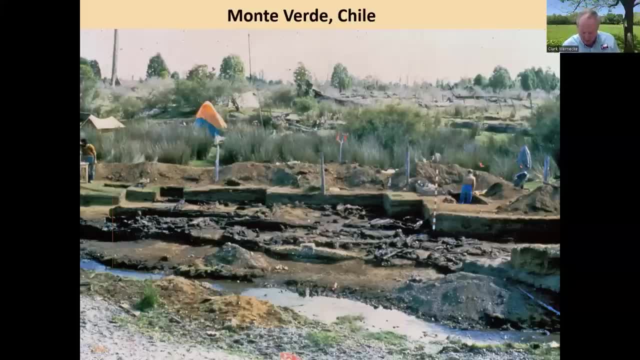 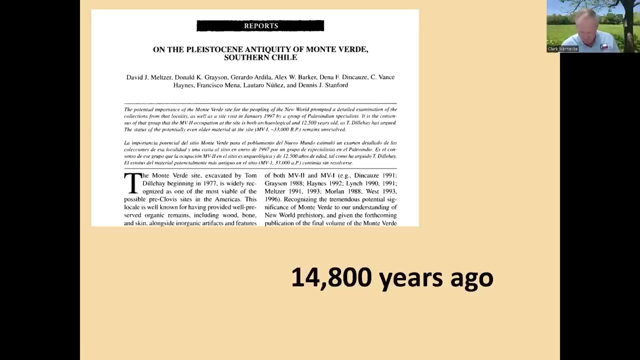 America and six from North America with disparate ideas about the peopling of the Americas. Later that year they published an article about the site, accepting it as a site with dates older than the early Paleo-Indian dates in North America. Now Monteverde has at least two occupations and perhaps three. The youngest dates to 14,800 years. 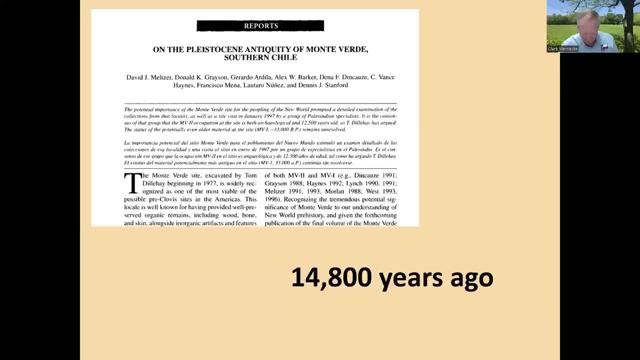 ago and is what everyone agreed on when they went down there. There are some indications- harsh and a few tools, of an occupation 18,300 years ago not everyone believes in and an even more ephemeral indication of something around 33,000 years ago that no one likes to talk. 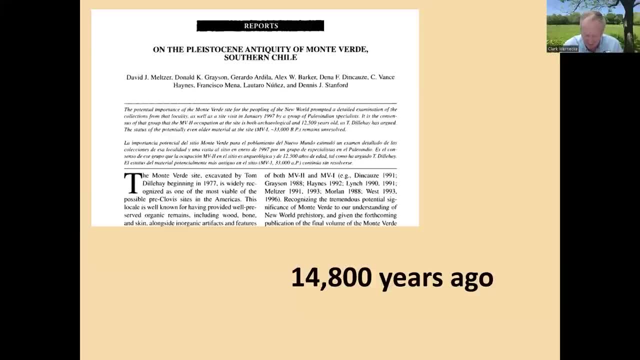 about. The summary of the consensus article might confuse some because they state the date in radiocarbon years about 12,500.. When you calibrate the date, you get around 14,800.. Despite this group of prestigious scientists agreeing, not everyone jumped on board. 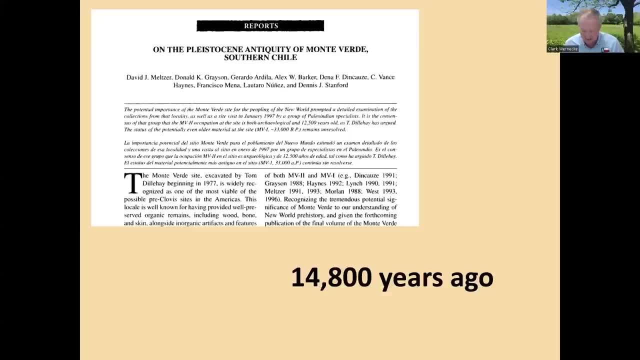 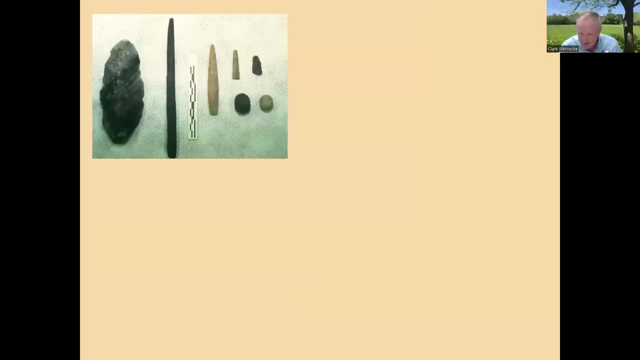 There have been many critiques. A recent article dismisses it because they say there are only about six tools that people agree are artifacts. I would argue that Highly respected lithic analysts disagree with that. But when did quantity become a rule of evidence? I was telling someone the other day if I find a Coke can on the surface of the moon, 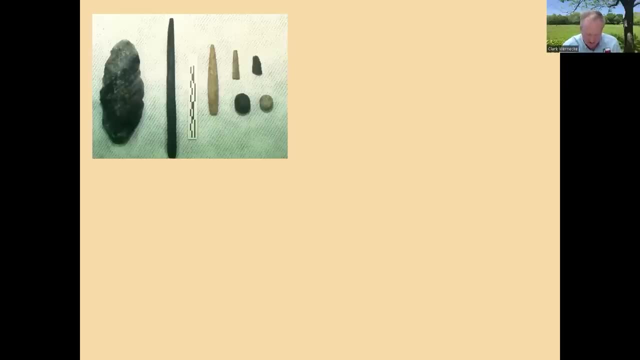 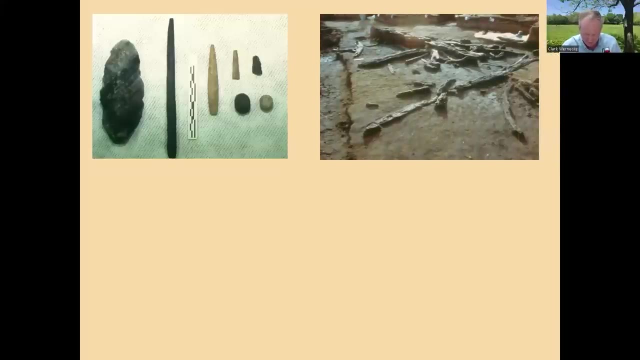 I can pretty much guess that people brought it there. And even if you didn't like or understand the stone tools, what about the structures that were found there? The foundation of a tent-like structure, 60 feet long, and a small horseshoe-shaped structure? 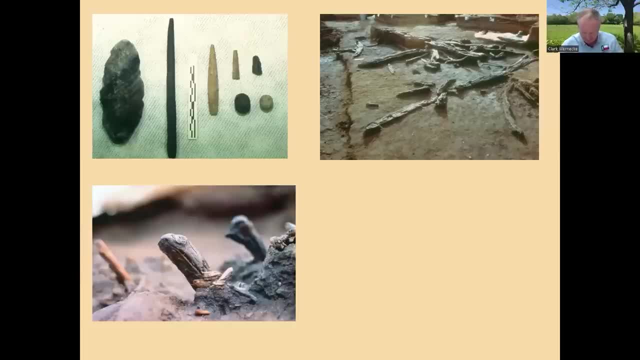 What do you make of the small sharpened poles of those structures, having vegetal matter tied to them? You can see a knot in this picture: The remains of hide clothing, edible seaweeds that came from a coastline that was 55 miles away to the west at the time. 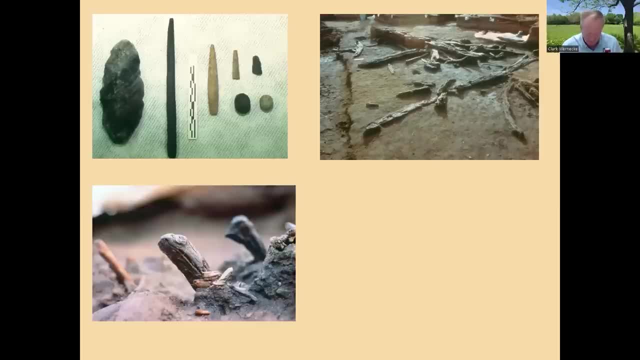 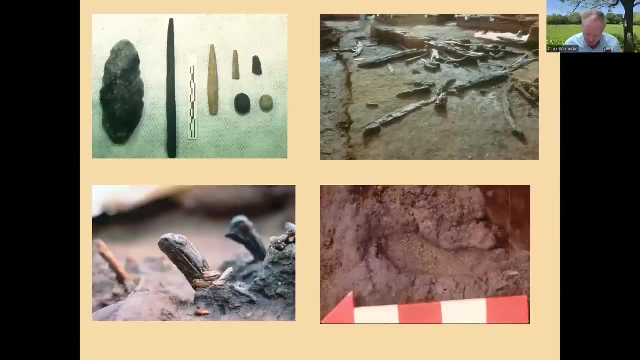 from a preserved piece of agampothere? How do you explain the human footprint found in the sediments? When we examine archaeological sites, we can't pick and choose our rules of evidence. We must examine them all together. Monteverde has 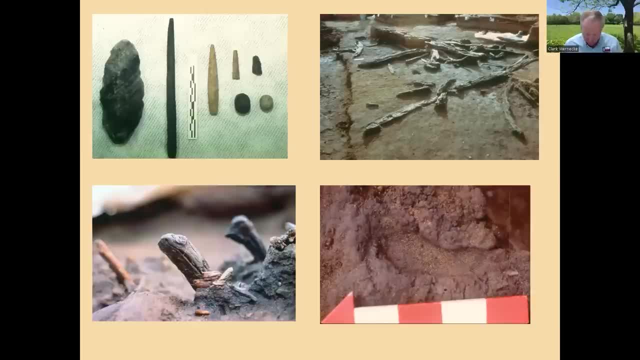 undoubtable signs of human occupation, with good stratigraphy, in good context and with accepted scientific dates. About 80 miles north of Monteverde, near Osorono, Chile, the site of Palauco Bajo also has lithics and megafauna with similar dates Prior to work at Monteverde. 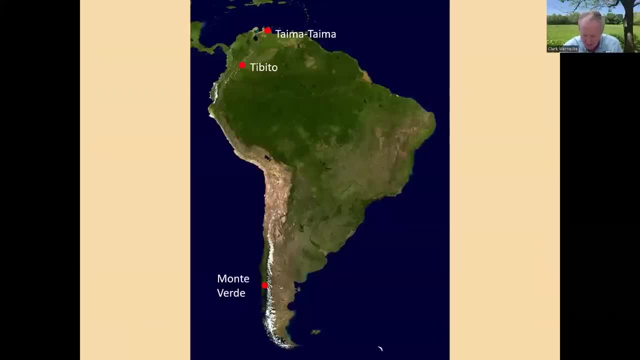 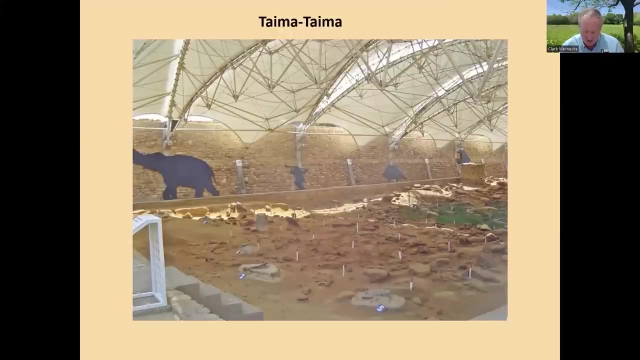 there was the site of both of these appear to be mastodon butchering sites. Tima Tima was excavated- well, it was found in 1962 and excavated over a number of years- and it's located around an artesian spring-fed waterhole where there was a juvenile mastodon. 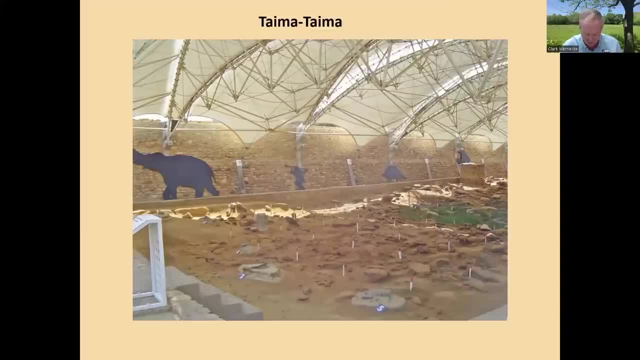 found with stone tools and a stone projectile point within the pelvis Tima. Tima has been dated to 15,000 to 16,000 years ago. The critique of this site is that it's a very old site and it's a very old site. 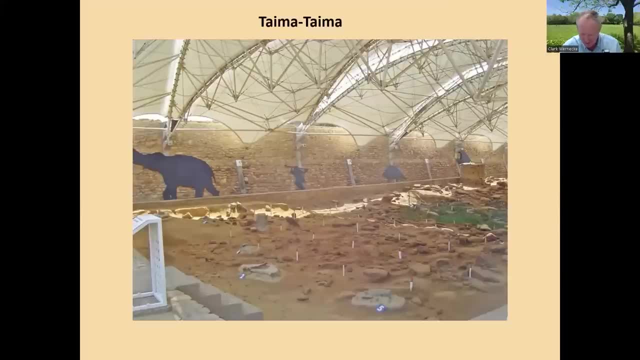 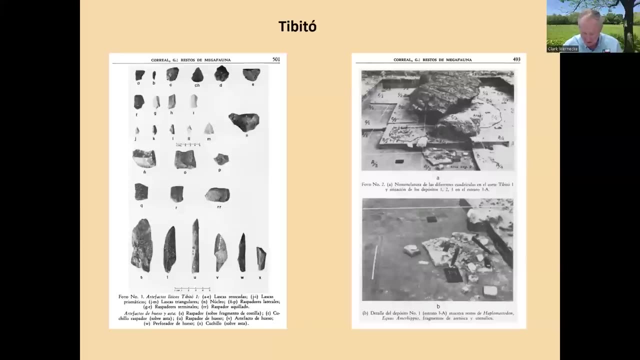 The critique of this site is centered around the provenience of the bone and stone tools, with some claiming they may have been moved around by water or may have moved through the soils. Thibodeau is located on the Bogota Plain in Colombia, over 8,000 feet above sea level. 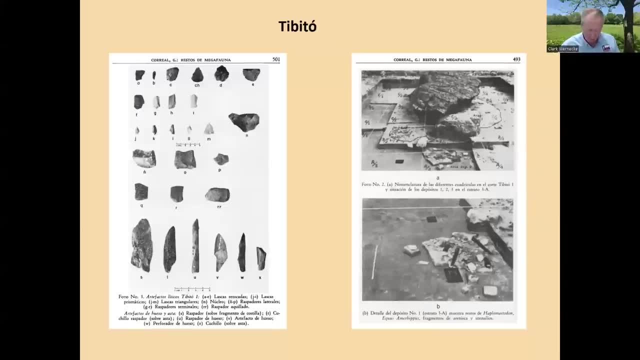 It's an ancient rock shelter with the remains of mastodon horse and a number of other animals in it. There's a large quantity of bone and stone tools and signs of butchering, breaking and burning on many of the bones. 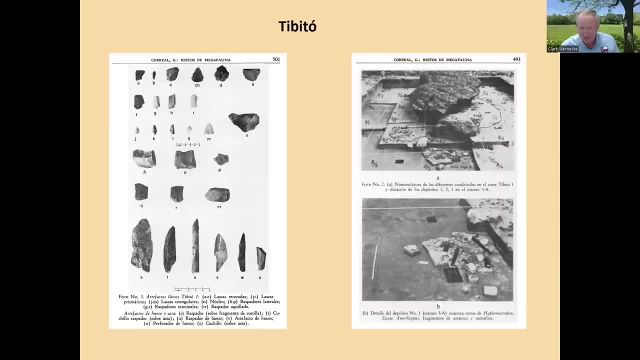 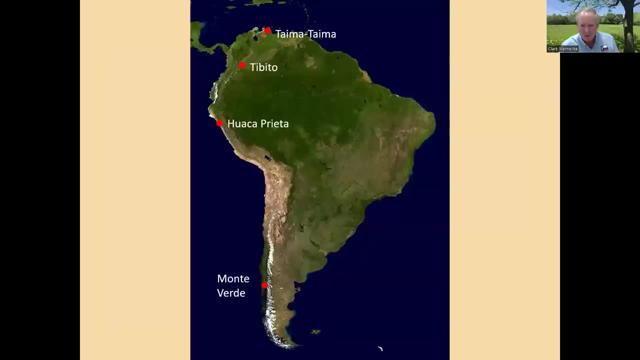 Unfortunately, the site is not known to the public. The site is not known to the public. There is but one radiocarbon date of over 13,000 years, so the site's often rejected as not well dated. Huaca Prieta is located on the coast of Peru and excavations there were conducted by Tom. 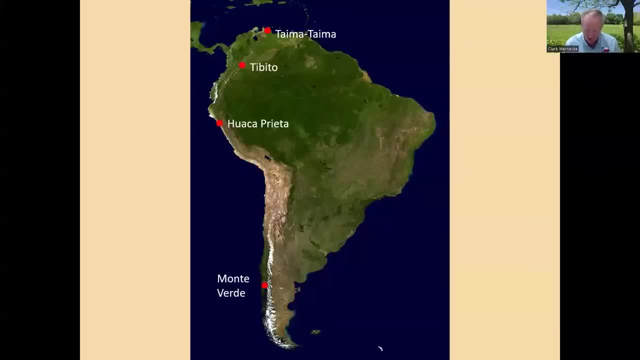 DeLay from 2006 through 2011.. Huaca Prieta means Black Pyramid and is the site of a very large pyramid of the Chavin culture, about 2,200 to 3,000 years old. Full disclosure: the gold and. 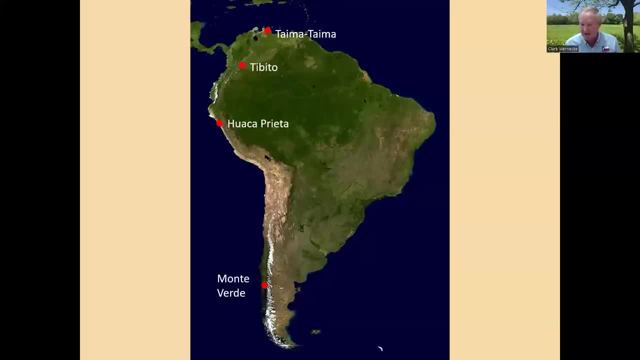 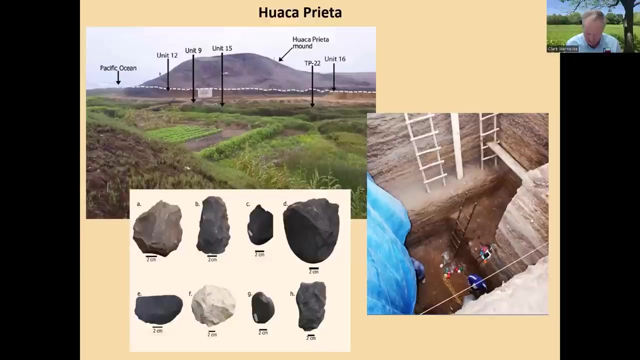 silver meadows You have saltwater, freshwater, swamp, high ground to choose from. That's about 105 feet of later deposits to get to very old river terraces. There they found stone tools and dates to nearly 15,000 years ago. 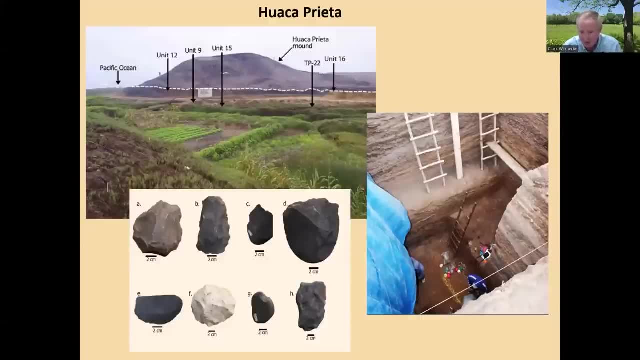 The people who lived on the coast 15,000 years ago were surprise utilizing a lot of marine resources, But they also found evidence of deer from the foothills and the earliest evidence of avocado use in this hemisphere- Ceviche and guacamole anyone. 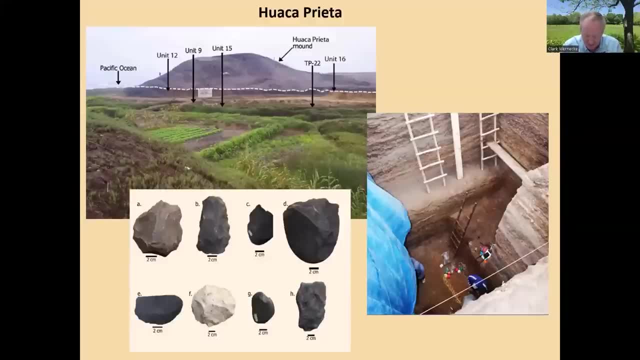 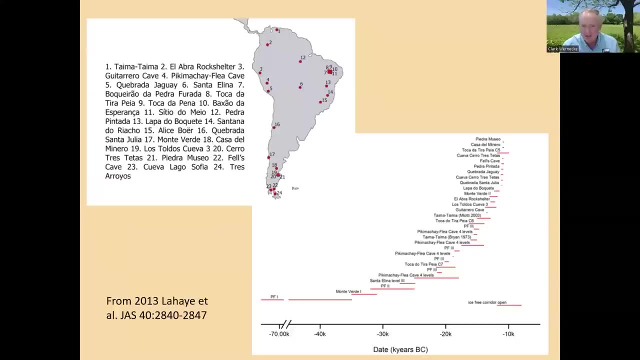 So those are some of the better known sites, Some only better known because they were excavated by North American archaeologists And they're but a drop in the bucket. If this was a semester long class, we might have time to go over all the sites of interest now. 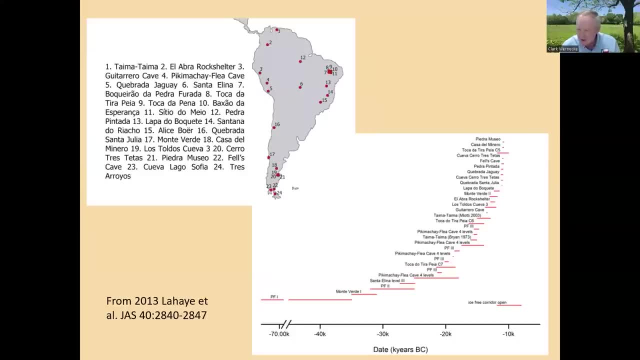 It's quite a long list, And if you look at the range of dates to the lower right there, you'll note that many of them are very early. The authors of this article will help enough to give us some idea of when people could have walked to North America. 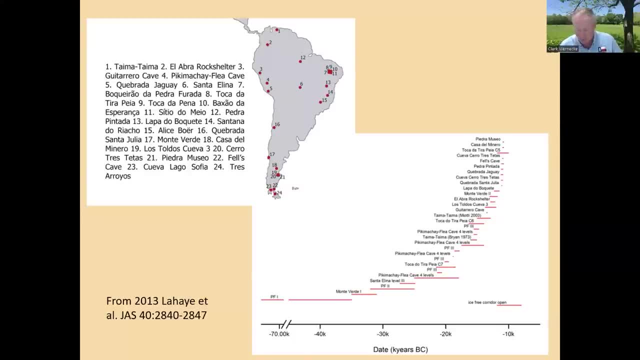 Down in the right corner. there you can see that little line, ice-free corridor open, And these sites predate the possibility of walking here. In addition, most are of Clovis age or older, making it impossible for Clovis to be the predecessor of these technologies. 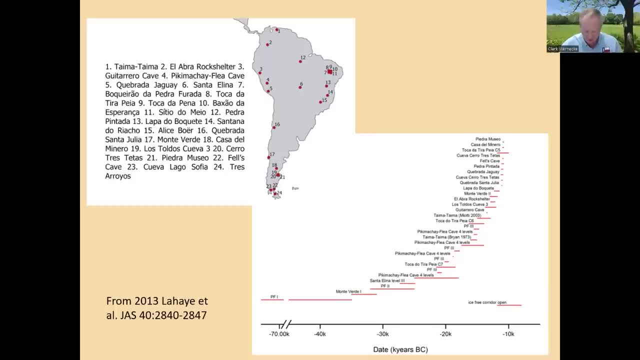 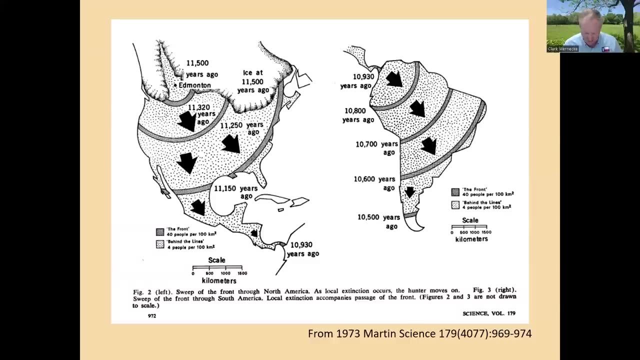 There had to be a technology these and Clovis derived from. For a long time, the idea was promoted that humans moved into a new, pristine world, killing everything before them And, as game became scarce, advancing forward in search of food. The first problem with this idea is that data supports the idea that these people were all broad spectrum hunters and gatherers. 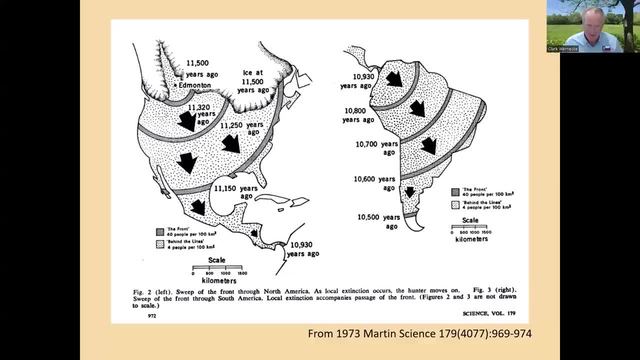 They didn't pass up easy foods or plant foods. If you look on the Internet for information on big game hunting cultures, it refers you to Clovis and Folsom. If you look for proof that Clovis is representative of big game hunting, it refers you to Folsom, and vice versa. 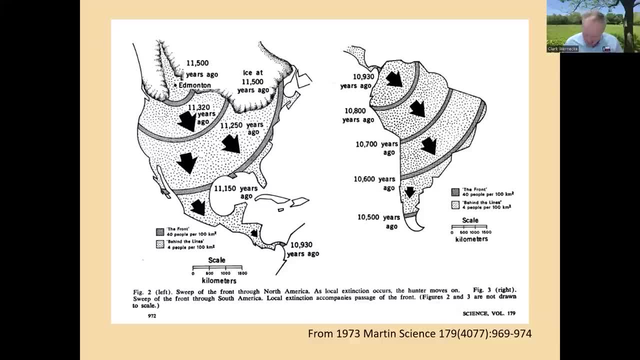 A little circular. It's not really possible for people to live on big game hunting alone. We've never actually seen a culture that exists that way. There's also a lot of data, if only you look for it, that plants and small animals, shellfish, bats, birds, insects. 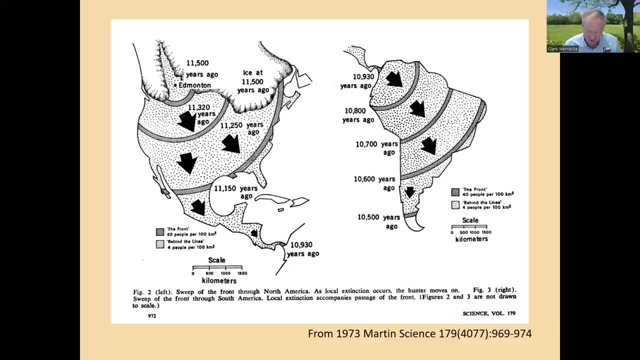 were driven to extinction at the same time, which implies that something larger than bloodlust is involved: A dramatic climate change. People are already living in a world where they can't live on big game hunting. They're living in a world where they can't live on big game hunting. 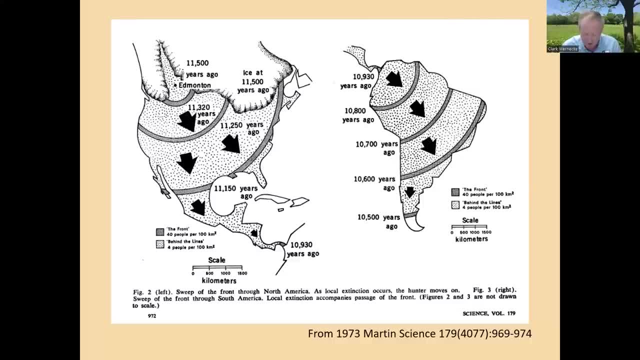 They're living in a world where they can't live on big game hunting. They're living in a world where they can't live on big game hunting. People reached Australia. apparently lived alongside megafauna for 20,000 to 30,000 years. 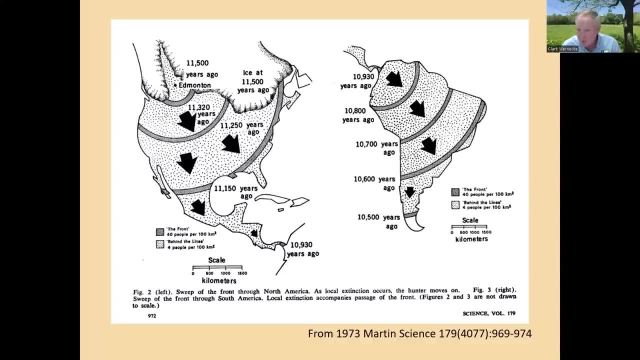 And new data is appearing that some of these animals may have been around a lot longer than we'd previously thought. For instance, a recent publication suggests that there were mammoths in the Yukon until 5,000 years ago. This idea also posits a very small starting population, around 100.. 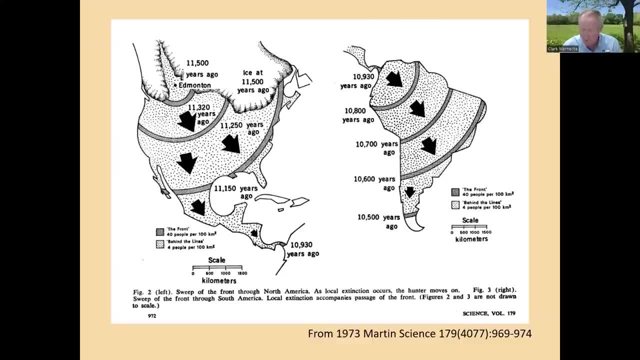 And there are a lot of arguments about how many people you need for a viable population. And there are a lot of arguments about how many people you need for a viable population, With good arguments from 160 to 14,000.. There's no agreement on this at all. 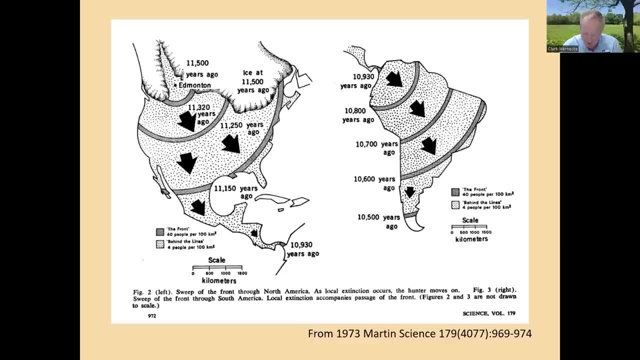 It's a problem that we often treat the peopling of the new world as an event where it's more likely to have been a process. It's not just one people, you know, one group coming over planting a flag and peopling the new world. 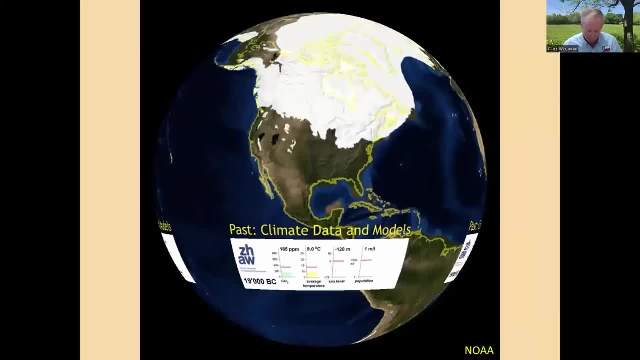 Okay, Let's look at North America. The Wisconsin glacial episode lasted from 75,000 years to about 11,000 years ago, And massive ice sheets covered a great deal of northern North America. At their maximum, the Cordillera ice sheet covered almost a million square miles of the west, from the mountains to the sea. 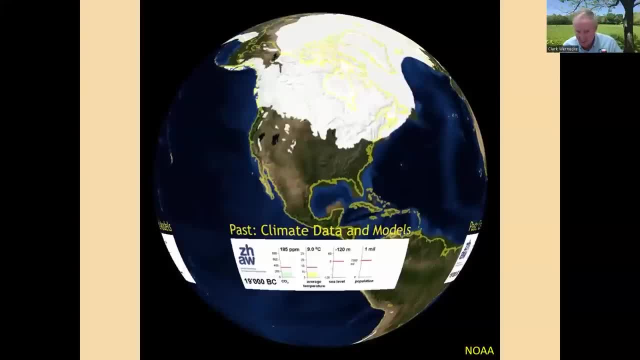 And the Laurentide ice sheet covered another 5 million square miles, up to three miles high Up in the north way. up here We have the McKenzie River Valley, And around 16,000 years ago the ice began to melt, creating a little gap between the two ice sheets. 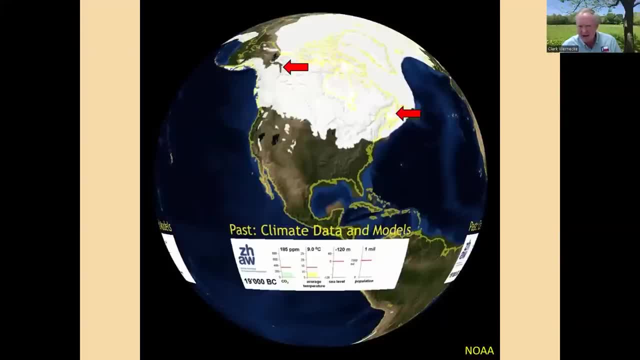 And a similar process started well way down in what's now Alberta. These gaps would have been filled first with freezing water, First rivers, then paraglacial lakes, then swamps, before widening enough to allow dry land. There's no evidence of animals or humans. 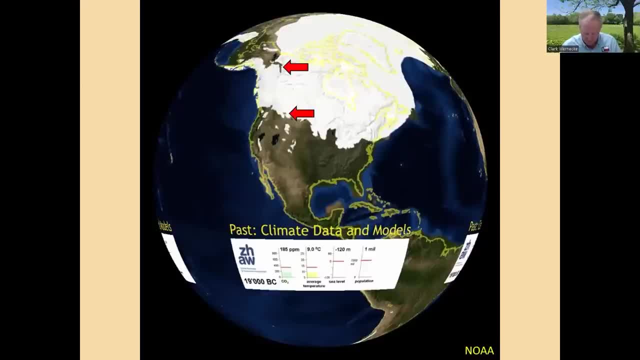 In these gaps until about 12,500 years ago and no evidence that these gaps connected prior to 12,000 to 13,000 years ago. In other words, there was no 1,500 mile long ice free corridor to explain the earliest peoples of the Americas. even if you still believe, Clovis is what they left behind. 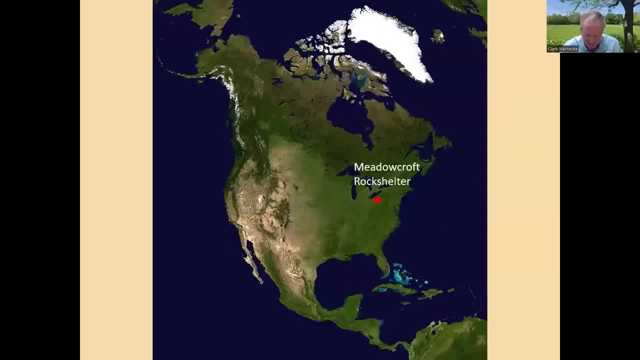 South of the ice. there's a number of sites to consider. The first we'll look at is Meadowcroft Rochester. The first we'll look at is Meadowcroft Rochester. The first we'll look at is Meadowcroft Rochester. It's a shelter in Western Pennsylvania. 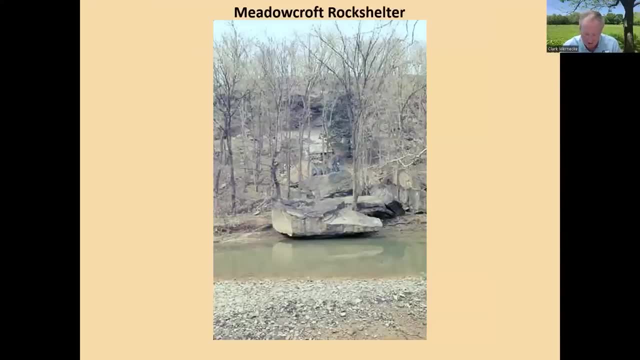 Meadowcroft sits above the bank of Cross Creek, a tributary of the Ohio River, And it was first discovered in 1955 by the landowner Albert Miller, who protected it until 1973 when Dr Jim Adivasio came to excavate there. There were extensive excavations from 1973 to 1978 and sporadic excavations through to 2007.. Basically, 11 years in total. The excavations were painstakingly done, sometimes digging with razor blades, and continued down through materials from a thousand years old to a roof collapse that. 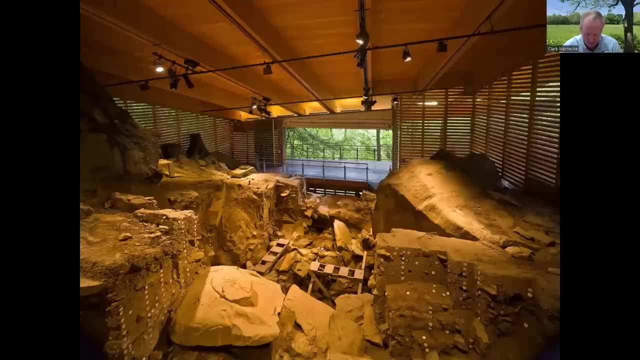 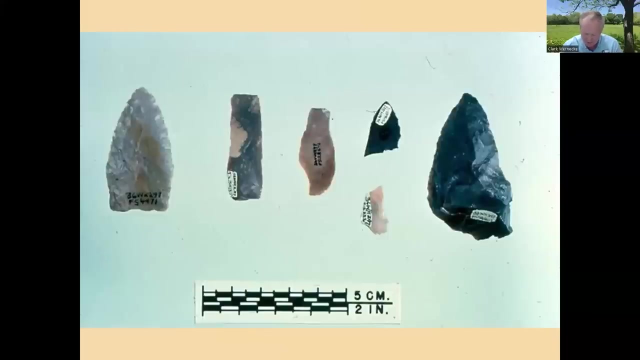 happened somewhere around 13,000-14,000 years ago. The excavations continued down about 16 feet and found materials from human occupation that date between 16,000 and 19,000 years ago. Artifacts included a basket fragment and an in-situ projectile point were found near the. 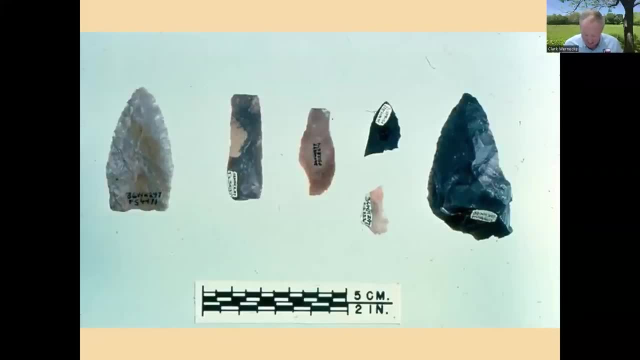 bottom of those units. Dates came from carbon-14 dates on charcoal and the basket fragment and the greatest critique of the site was that these were probably contaminated by coal in the water table. Repeated tests by the excavation group have shown no such contamination. 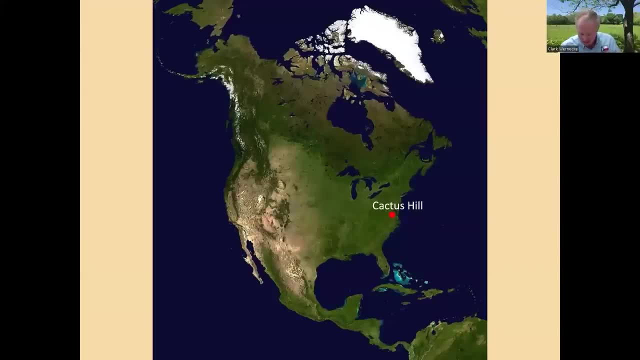 Well, let's take a closer look at Cactus Hill. It's about 37 miles south of Richam Virginia. The site was an open-pit sandbine and was first discovered in the 1980s by an avocational collector, Subsequently Joseph McAvoy of the. 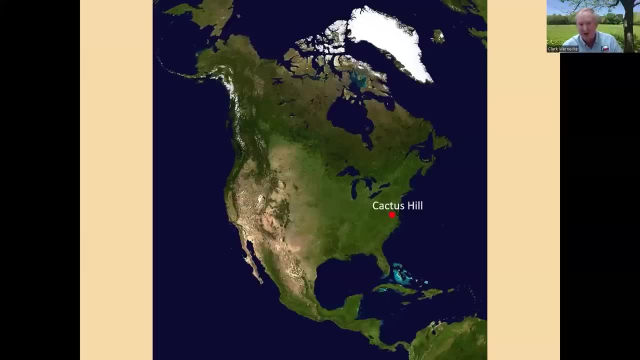 Nottoway River Survey and Mike Johnson, with members of the Archaeological Society of Virginia, excavated here, starting with a test by McAvoy in 1988 and substantial excavations by both groups between 1993 and 2002.. 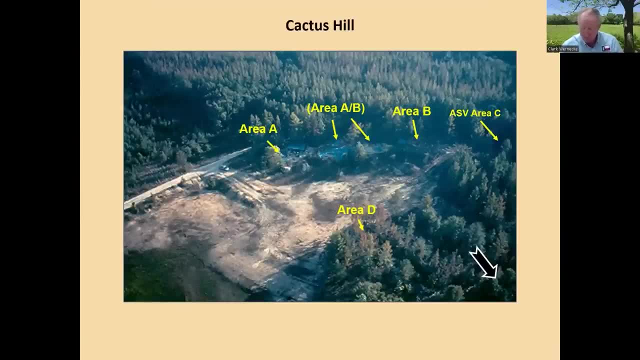 Cactus Hill has a well-dated Clovis component including projectile points and, in areas A and B, artifacts below the Clovis strata with dates of 18,000 to 20,000 years ago. The Clovis component is discrete and undisturbed Below a 7 to 20 centimeter sterile zone. 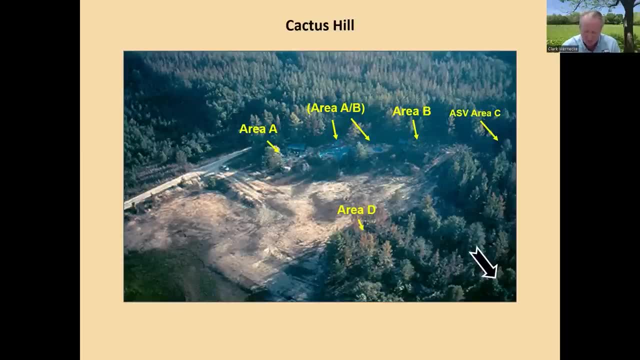 the researchers at Cactus Hill found more stone tools, but they're quite different from the Clovis occupation. above them, Phosphate, an indicator of human presence, was found in the soil. Even better, the carbon-14 and luminescent soil dates are in agreement. 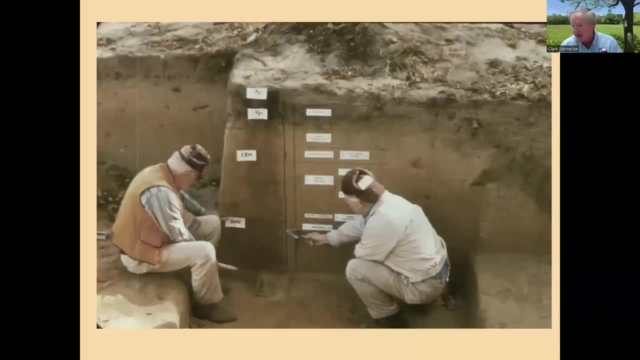 Critiques have often been based on the fact that the soil is sandy, so artifacts may have moved down through the soils. Micromorphological analysis showed that Cactus Hill had multiple buried surface horizons that are spatially and temporally discrete. Oh yeah, and there's no sign of mixing or downward movement above it. 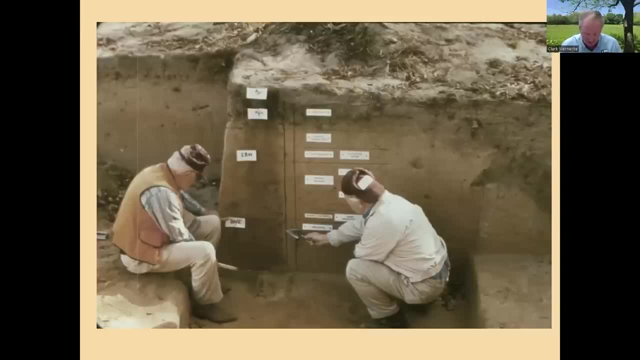 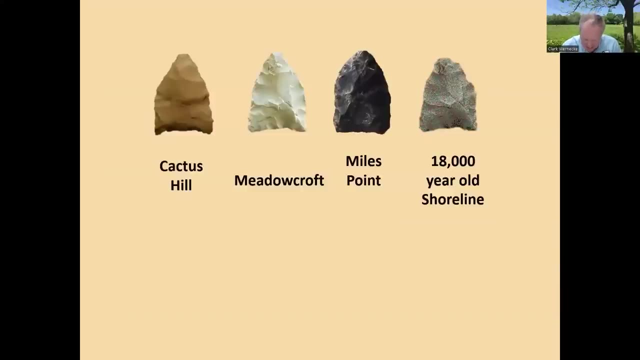 and the assemblage below Clovis is not Clovis technology, Well not even close to definitive. it is intriguing that we're beginning to see some artifacts that, at least morphologically, look alike. I actually don't know of an in-depth. 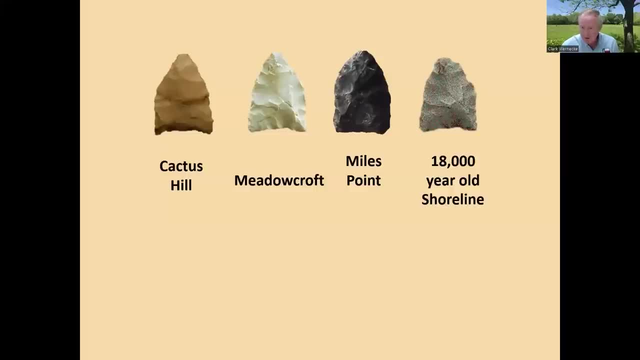 technological analysis. yet The Miller point was found at Meadowcroft and some similar artifacts at a site downstream. The early deposits at Cactus Hill have a similar looking point and others have come from along the Nottoway, the river nearby. The artifacts from old deposits at Miles Point on Chesapeake Bay. 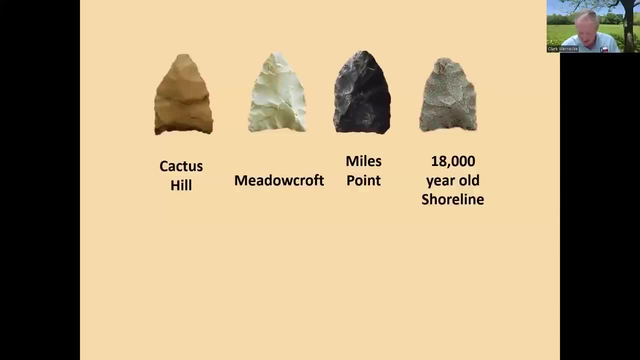 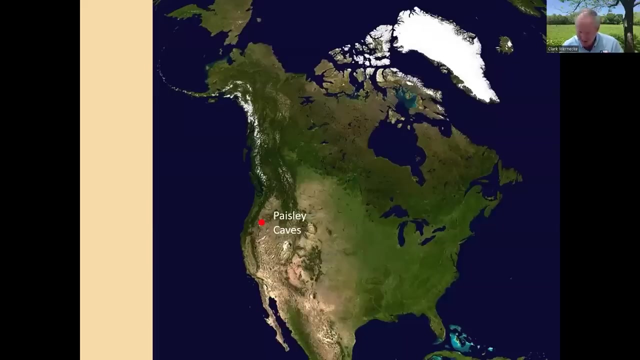 also look similar to one found on the 18,000 year old Delmarva shoreline. underwater in the Atlantic, Archaeologists looked for patterns of human behavior and perhaps we're starting to see some. Let's jump all the way to the West Coast to look at Paisley Caves in Western Oregon. This site was first discovered by the fathers of the Chesapeake Bay. This is a site that was first discovered by the fathers of the Chesapeake Bay. This site was first discovered by the fathers of the Chesapeake Bay. This site was first discovered by the fathers of the Chesapeake Bay. 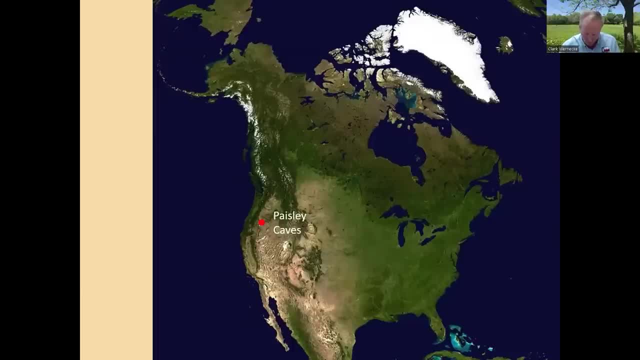 This site was first discovered by the fathers of the Chesapeake Bay of Oregon archaeology Luther Cressman, who worked there in 1939 and found extinct animals- horses and camels- with stone tools. His colleagues at the time cast doubt on his. 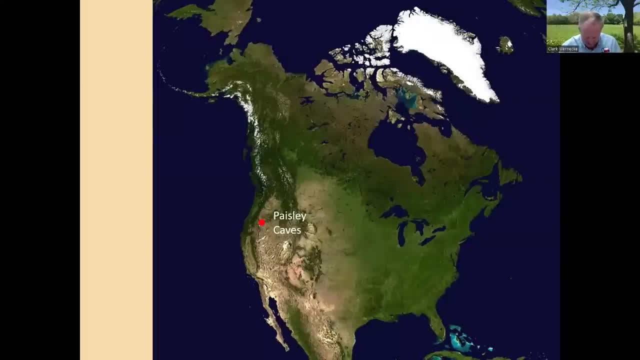 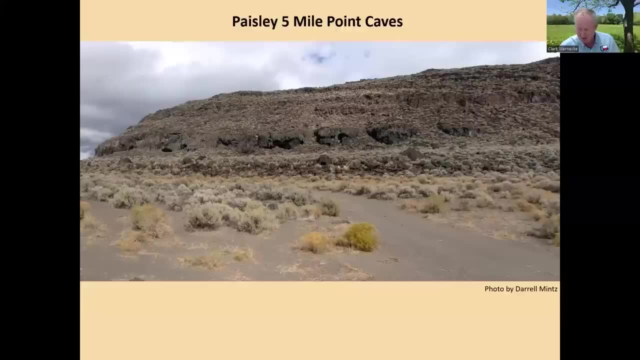 finds because, of course, people had only been here for 4,000 years. The site is a series of caves just above an ancient lake bed, And in 2002, Dr Dennis Jenkins from the University of Oregon went back to the caves to test Cressman's idea that early humans 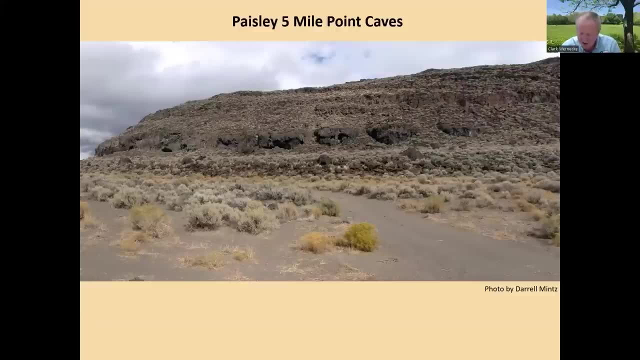 were living alongside and hunting now extinct horses, camels and bison. Several of the caves were painstakingly excavated and news reports proliferated when the team found coprolites. We have to have a different word for everything so human turds that dated back to 14,300 years old. 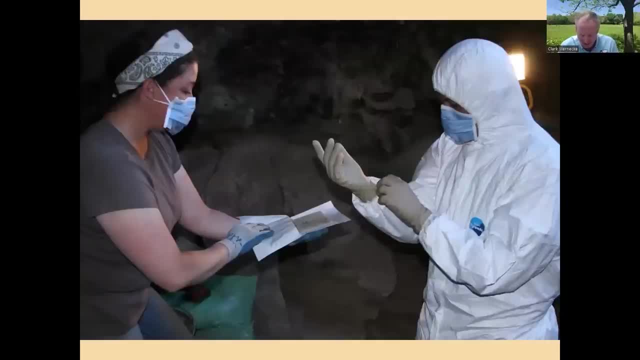 Now critiques of the site are primarily focused on those coprolites- that perhaps they were younger than the sediments they were in, or maybe not even human. The first test of the studies looked for human DNA and dated the organics in them. The researchers went back. 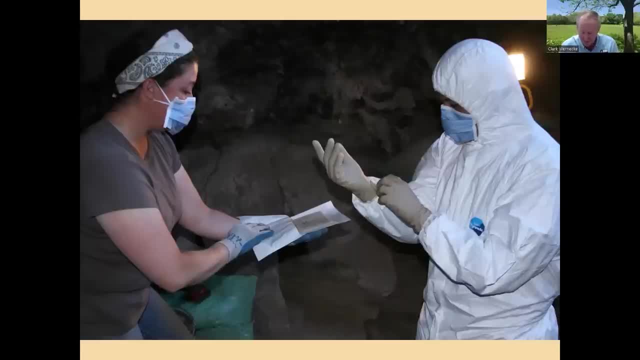 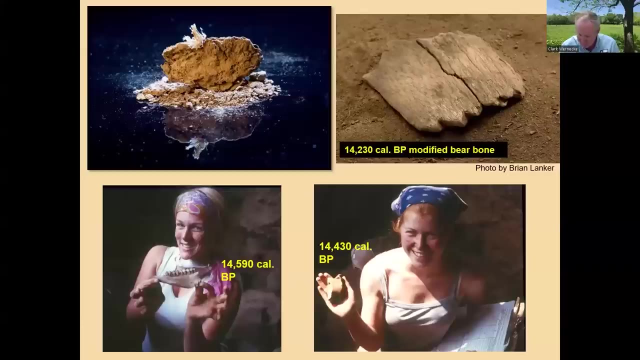 to look at lipids, fatty acids in the samples that are less likely to move around in the soil and conveniently can also be directly dated, and got similar results. Even so, they found modified bone and fauna with butchering with similar ages and stone tools with proteins on. 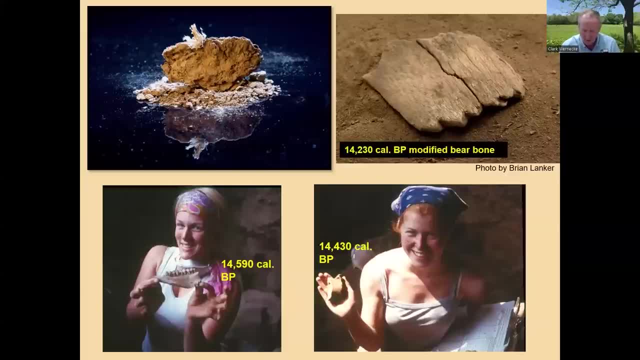 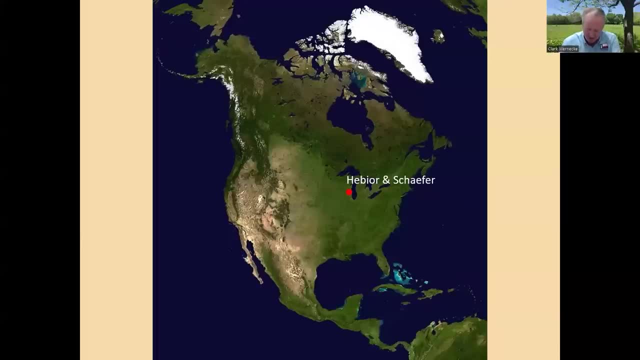 them for mammoths and horses. We've looked at east and west, so now let's look at the midwest, at the Schaefer and Hebbier mammoth sites. Schaefer was found in 1964 by a backhoe driver putting in drain tile. 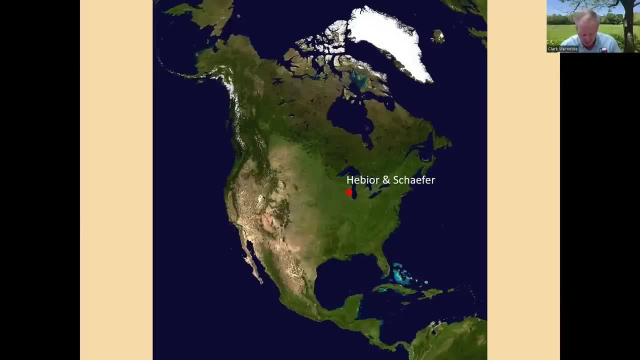 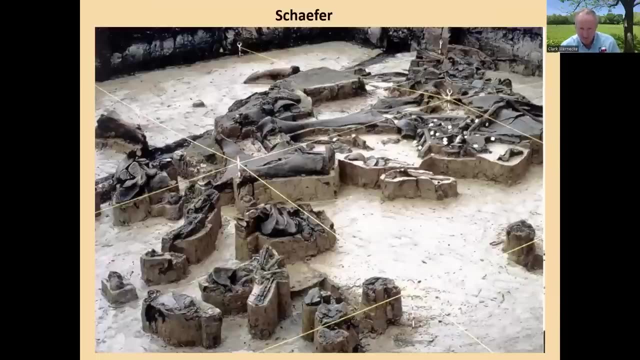 and Hebbier was found in 1994 just a quarter mile away. Dan Joyce of the Kenosha Public Museum excavated there in 1992 and 93 and found 80% of a woolly mammoth, disarticulated and piled. 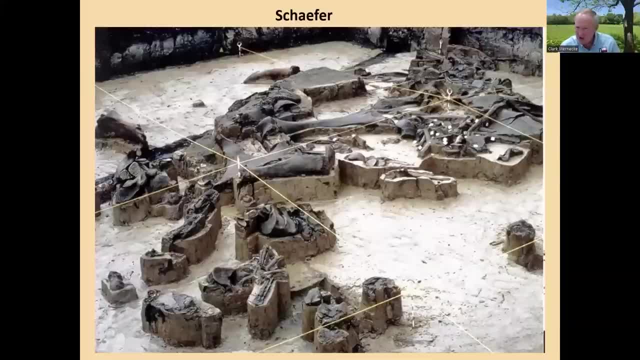 Two of the mammoths were found in the midwest and two of the mammoths were found in the south. Two small chertules were found and the skeleton had numerous cut and wedge marks on it. It had definitely been butchered. Imagine their surprise when they got dates back of 14,500 years ago. 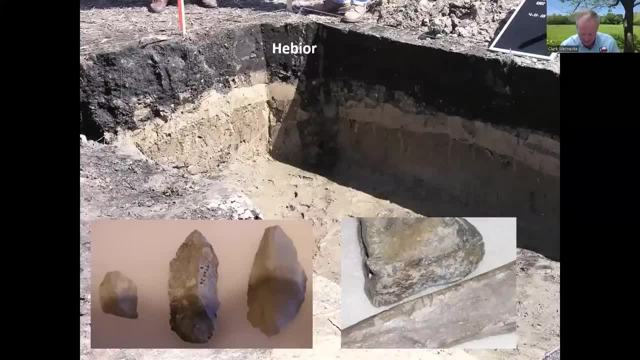 Just down the road, literally within sight of Schaefer, another mammoth was found, and this time it was 95% complete David Overstreet, excavated in 1994 and found not only tools but once again very clearly. 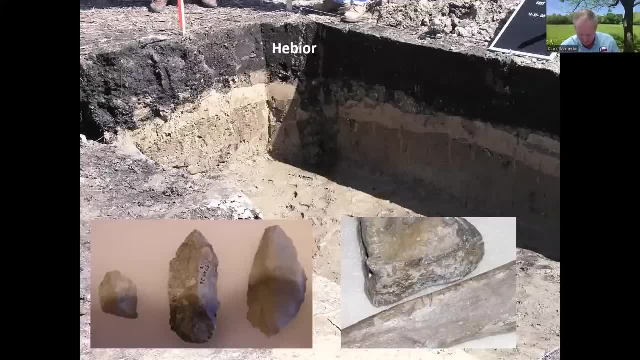 Hebbier cut marks on the bones. You can see some of those in the lower left picture. Hebbier dated 150 to 200 years older than Schaefer. Well, we've done east, west, north, so we'll head south to look a bit at the Galt and Deborah. 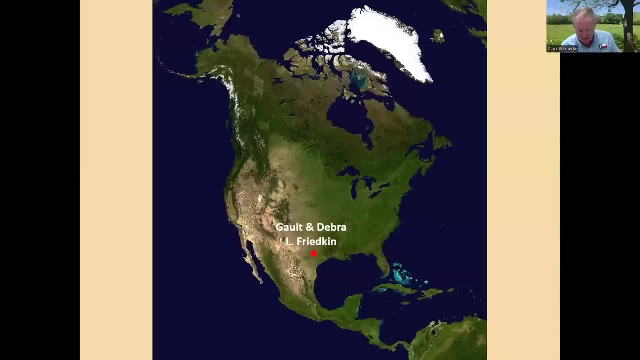 Friedkin sites in central Texas. Now I'm 100% biased here, as I have worked at Galt since 1999 and head up our non-profit as well as the research in the lab. I can tell you we did not. 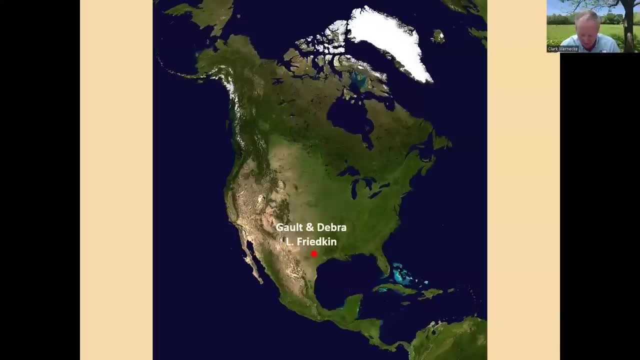 excavate the bones, but we did look at the bones. We did look at the bones and we did look at the Galt, looking for evidence of the peopling in the Americas. We were there because Dr Michael Collins is one of the leading experts on the Clovis culture and Galt has lots of Clovis. 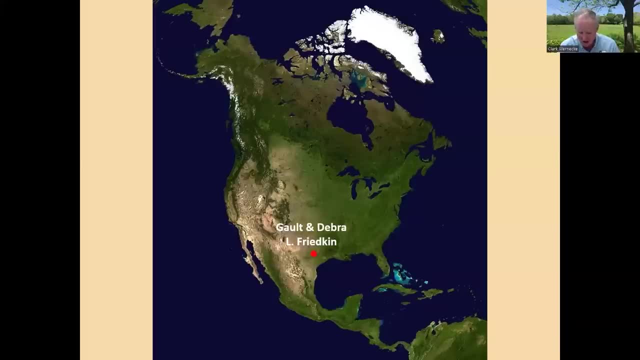 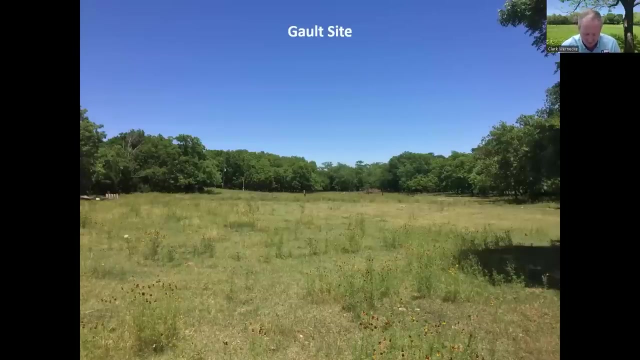 evidence more than 600,000 artifacts from that culture alone. The site's been known since 1929, and a brief test excavation was done there in 1991.. Galt is actually in the floodplain of Buttermilk Creek, a tributary of the Salado River. It's about 40 miles north of Austin and it's a 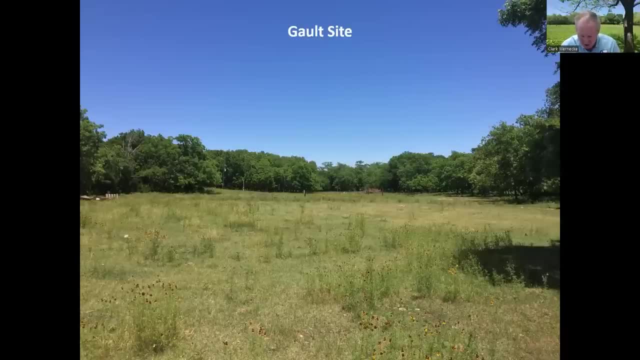 Texas. In this picture you can just see a fence in the valley. The gate's right in front of that burn pile. you can see down the valley and the Deborah Friedkin site is less than 300 meters, about 800 feet, down the street from this gate, just over the trees to the left of that burn pile. 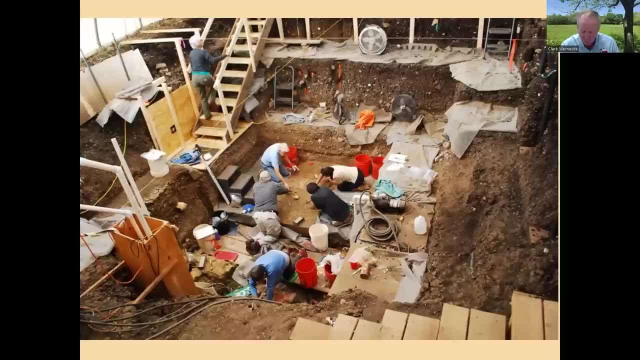 There were many excavations on the site. over a period of about 11 years We looked at an estimated three percent of the site and we discovered two percent of the site was 1.6 million artifacts from 22 cultures. Our last excavation was in response to finds deep in some. 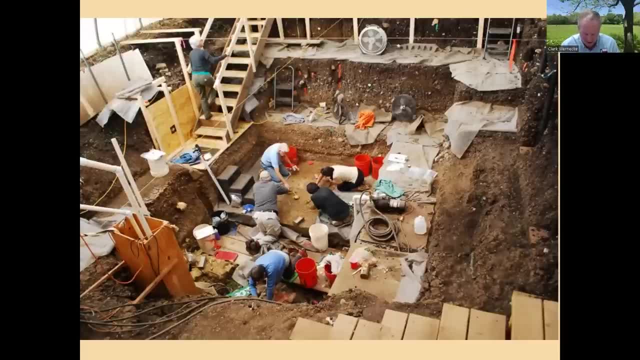 test units that we dug to show some of our colleagues the geology of the site. Above bedrock and well below Clovis, we found stone tools where they really shouldn't be. A 56 square meter unit was started in 2007.. You can see area 15 here in this picture and it was designed to step in twice. 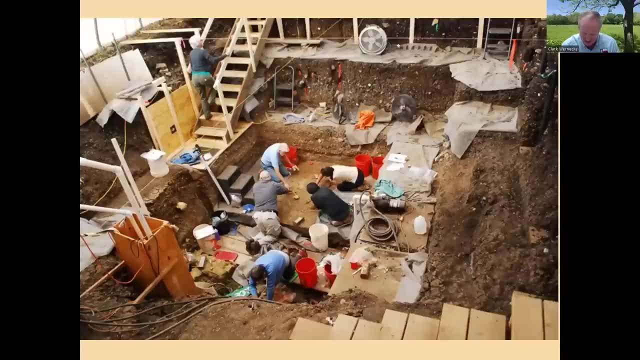 to avoid anything dropping down in the lower areas and expose an area on the underlying bedrock to see what was going on there. In doing so, we found 130,000 artifacts that predate the Clovis culture, 16 to 18,000 years old. In 2018, we published an article in Science Advances. 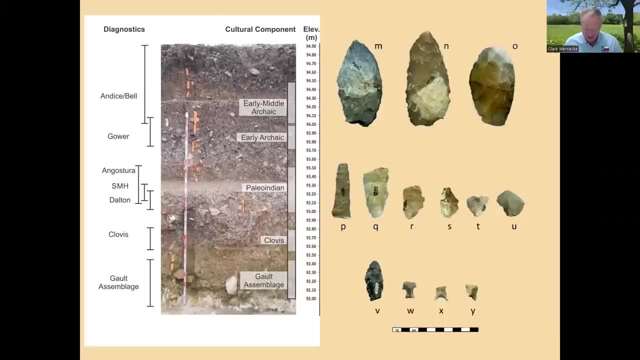 regarding the geology and dating. it called: It's open source, so you can find it online and read it. It's open source, so you can find it online and read it. It's open source, so you can find it in the article and read it. It's open source, so you can find it online and read it. It's open source. 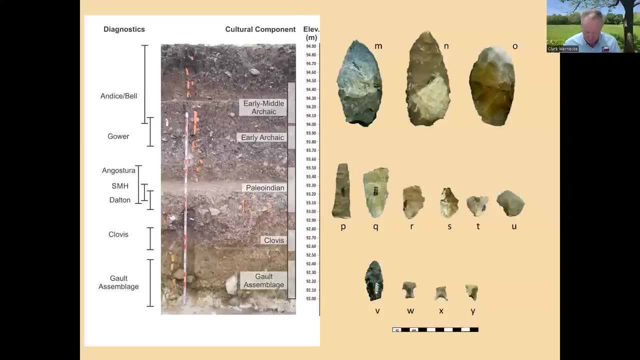 so you can find it online and read it. It's open source, so you can find it in the article. The Clovis and older components should go to the publisher this year with much more detail, so you'll probably see it in about two years, Since we do not yet have enough information to. 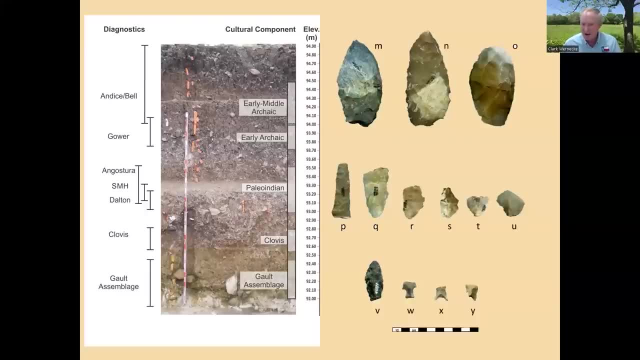 describe a culture or cultures, because cultures are patterns of human behavior. we've preliminarily called the oldest material the Galtas sandwich and it's significantly different technologically than the Clovis materials above it and nothing is moving down through all the other cultural 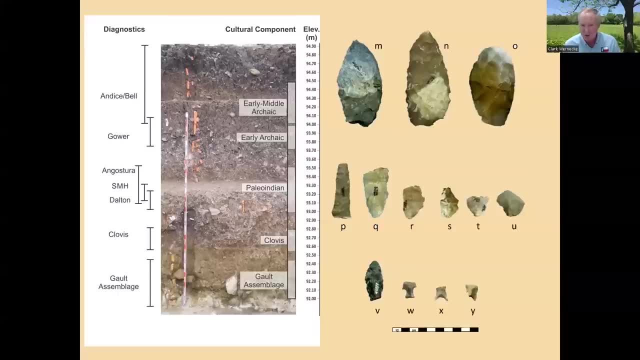 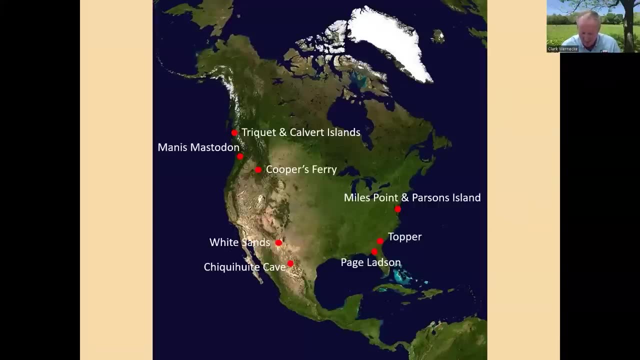 layers to get to the that depth, and we show that rather definitively in the article. It would literally take me days to go into greater detail about these sites and others like these that have data to add to the discussion. Triquet Island has good dates on Harz, 14,000 years old, while Calvert Island has 29. 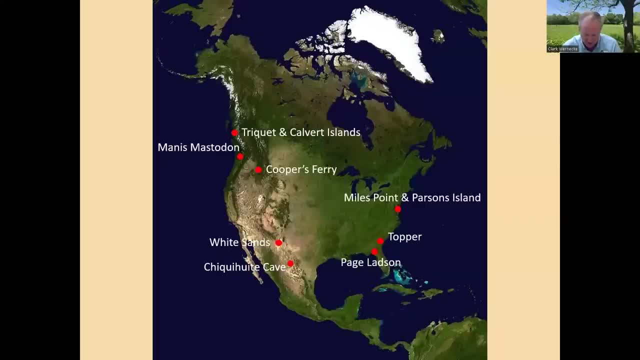 human footprints at least 13,000 years old. Recent years have seen the publication of old artifacts at Cooper's Ferry in Idaho and Chicoita Cave in Mexico. Very recently, researchers published on human footprints interspersed with Pleistocene animals at White Sands, New Mexico. 23,000 years old. Well, what about early, early man? The Cerruti Mastodon is dated at about 130,000 years old and Calico Hills, which Louis Leakey claimed was 100,000 years old, Smart scientists. 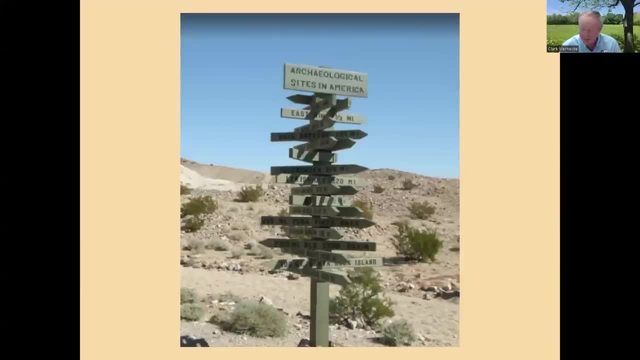 learn to date. Never say never. Today's absolute could be disproved tomorrow with new data. We do, however, have established rules of evidence and currently- well, maybe, perhaps it's like Lewis and Clark's Clovis points- there's just not enough evidence to definitively show a human presence earlier. 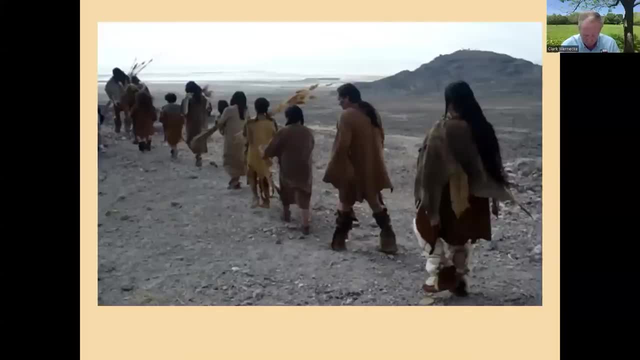 Okay, so how did they get here? Wow, okay, this is the touchiest subject. For a long time, we believed the first people to be able to see a human was a human. We believed the first people in this hemisphere walked here And no one's disputing that. later on, 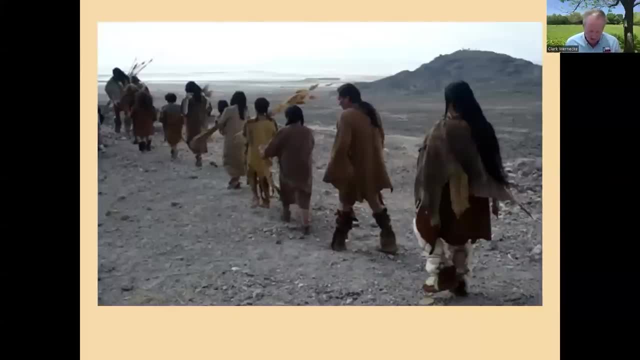 both people and animals walked both directions. But if people were here 25,000 to 30,000 years ago, they couldn't have walked here, And that's when it starts to get messy. To get here prior to that, you have to come along the coast in boats. So some of my loudest 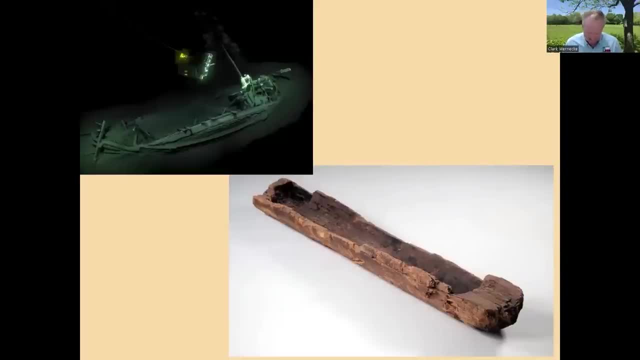 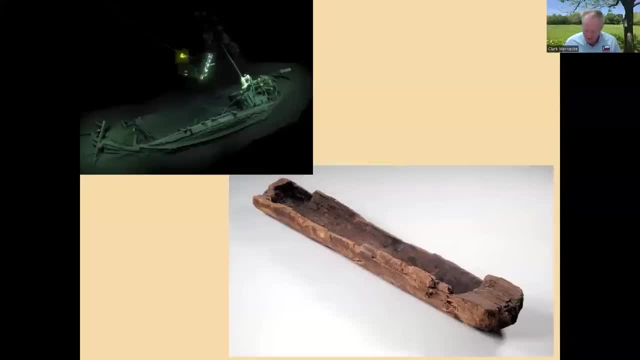 discovered the oldest known human ship, a Greek ship, 2,400 years old in 2017.. No one doubted the Greeks had ships prior to that, since there was other evidence, like trade items, to support the idea. The oldest boat in the world right now is a dugout canoe. 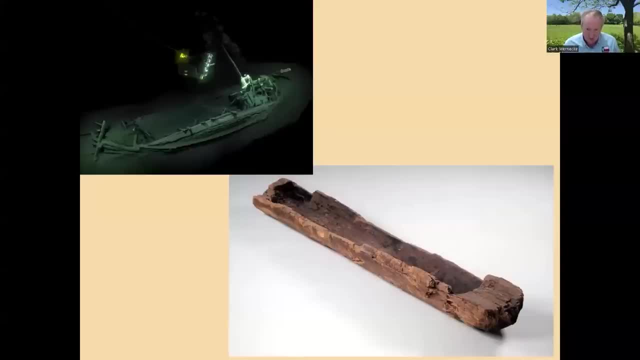 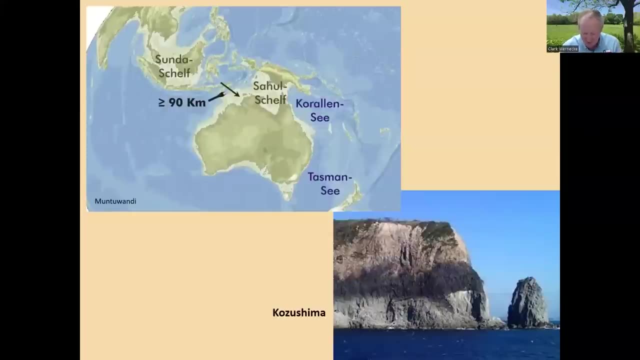 from the Netherlands around 10,000 years ago. So what other evidence is there? Well, people arrived in Australia somewhere between 50 and 65,000 years ago and they had to cross almost 60 miles of water to get there. 25,000 years ago, we found people in Japan using obsidian from Kazushima. 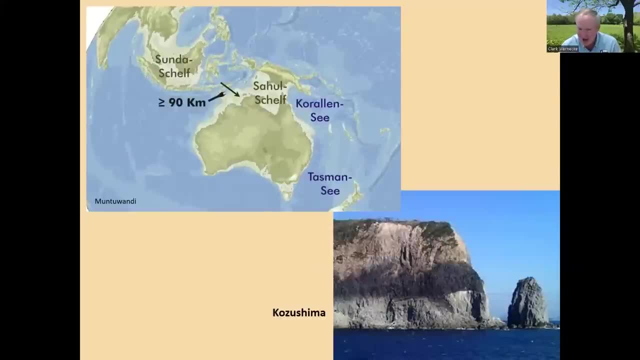 Island In that lower picture that black stripe is not a shadow, That's actually obsidian. And Kazushima Island is 30 miles from the mainland. You know, I guess we're suggesting somebody swam with a big obsidian rock under each hour People getting to the island. 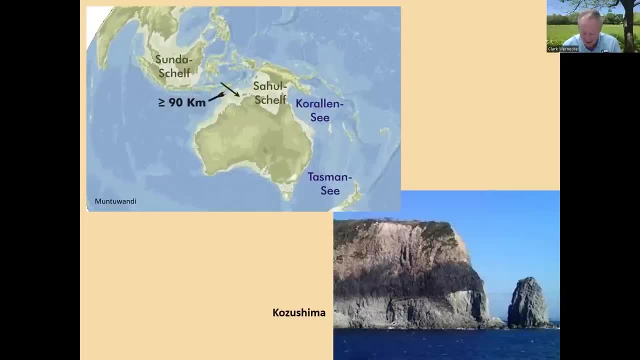 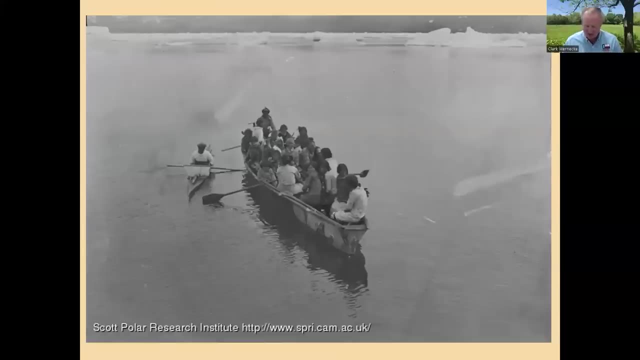 the island of Crete 130,000 years ago needed some kind of watercraft, as did the early hominids in Flores, Indonesia. Skin and bone boats still used today in the Arctic. umiaks have a tremendous capacity. This photo shows somewhere between 20 and 22 people. I lost track in the middle. It's 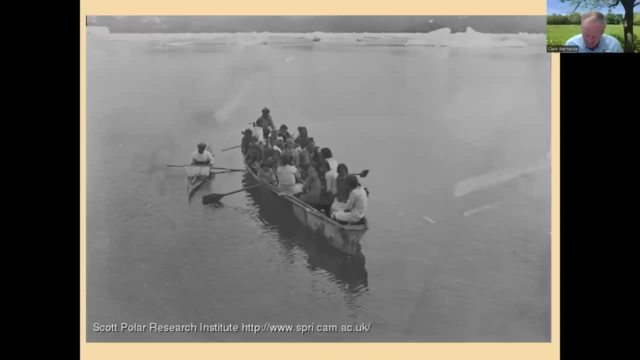 hard to distinguish And it leaves no archaeological signature. It's made of skin and bone. If the weather gets rough- modern whale and seal hunting- they're simply pulled the boat onto the ice and use it as a tent. A British journalist with two 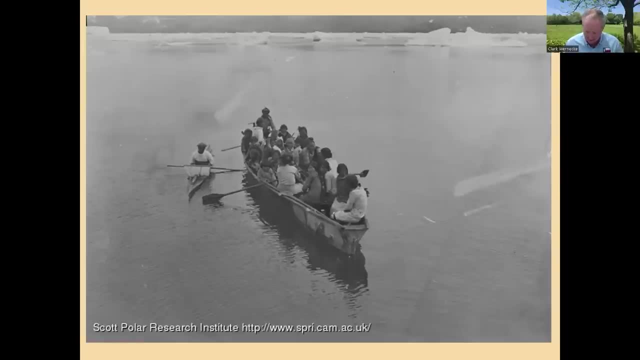 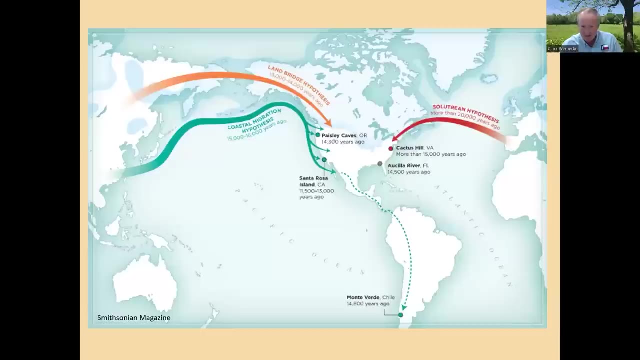 companions made a journey from Ireland, where they have a similar boat building tradition to the New World: Three guys in a skin boat. There are three major hypotheses right now: The land bridge- that's the hypothesis we were talking about before that people walked here. 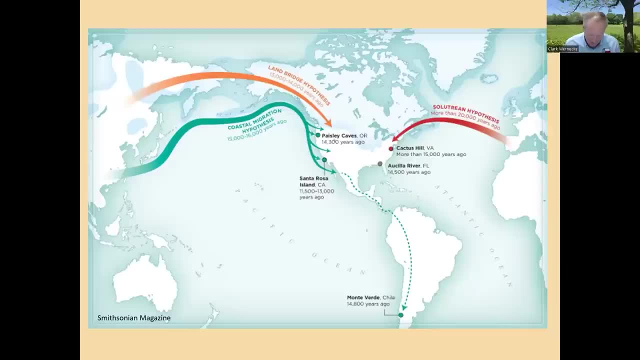 Coastal migration or the kelp highway hypothesis and the salutary hypothesis. There's no evidence of crossings through the Pacific. Much of the peopling of the Pacific Islands was about 1200 years ago. Nor is there any evidence of direct contact with Africa. 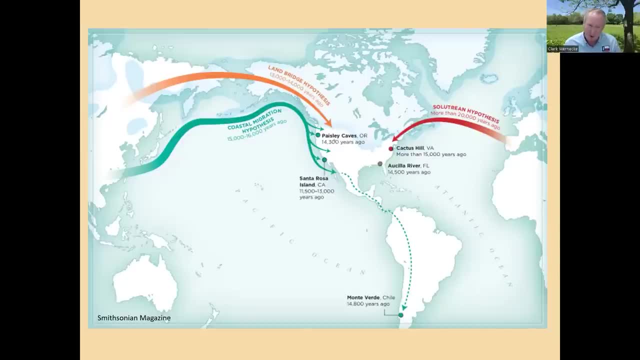 If the first peoples got to this hemisphere prior to the opening of a corridor between the Cordillera and the Laurentian ice sheets, then that leaves us with two choices: Along the Pacific or Atlantic coasts, in boats or both. This is a process and not a true-false test. 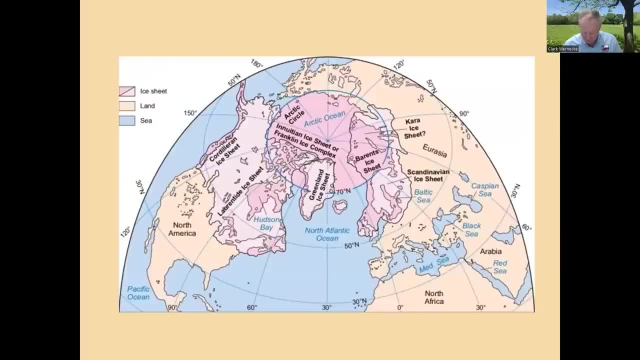 Traveling along the North Atlantic ice sheet may even be a shorter distance than the Pacific route. There are migrating birds and seals moving along this ice front, as well as the now-extinct auk, And since all of these species have to have dry land, any moderately attentive hunter 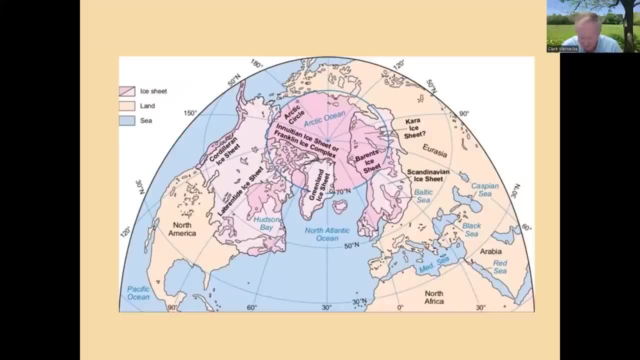 could make the connection that there was more to the west than just water and ice. It's not an especially difficult trip, despite what some people think. In addition to our British journalists, more than 156 solo rowers have done it in modern times In 1563, a group of people 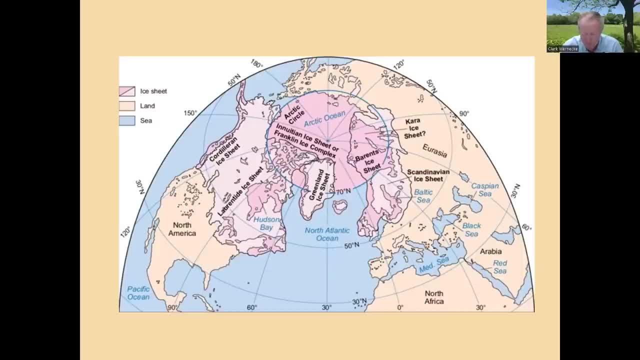 stranded in South Carolina, built a homemade boat- and most of them survived to eat. England Inuit, probably from Greenland, landed in Scotland in 1682 and in the early 18th century. So is it possible? Well, the answer is yes. People could easily have done it. 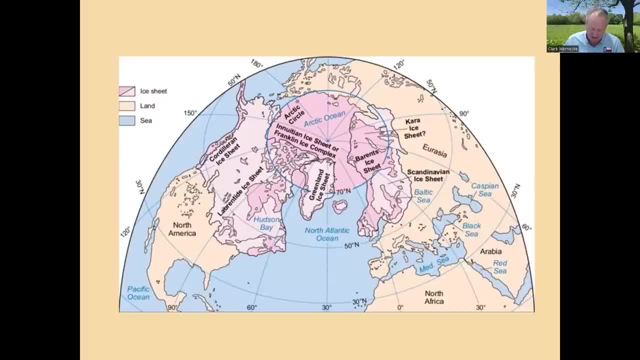 Now I'm not going to get into the details of the salutary hypothesis here, But let me say, if you quit calling it salutary and just think about possible migration from what's now Europe, there is a possibility And hypotheses should be tested, not dismissed out. 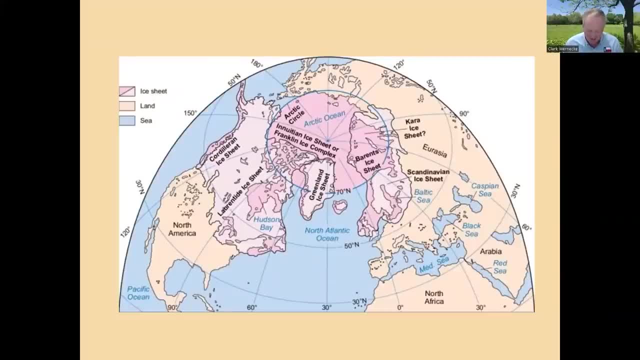 of hand. We'll talk a little bit about genetics in a minute. The biggest controversy here is that neo-Nazis hailed this as white people were here first, despite the fact that genetics for white skin is only about 9,000 years old. But that doesn't mean that we're going to be able to see. 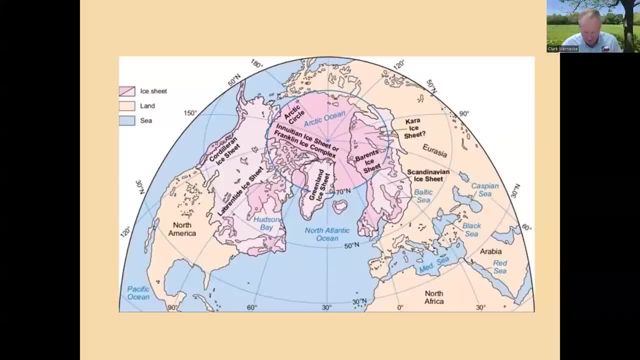 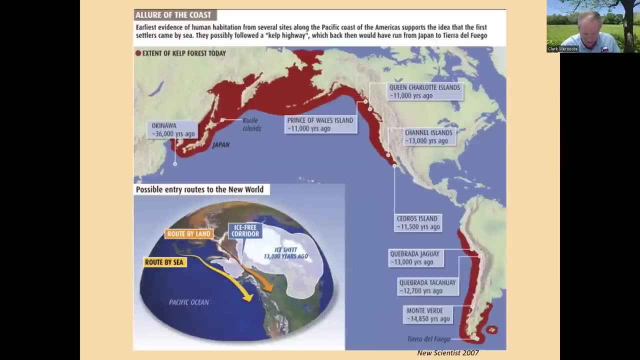 that. So the knee-jerk reaction for many people is: oh gosh, not from Europe, That's just a big can of worms. Traveling along the Pacific coast is certainly possible and relatively easy if perhaps a bit longer There would have been refugia areas free of ice along the coast We have. 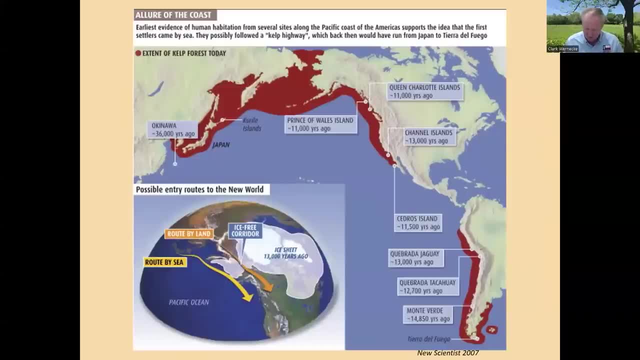 some very early occupations of the area, places like Triquet and Calvert Islands. We find the remains of bears along that route in the Pleistocene, And bears actually need a lot of food. They need a pretty good area. There's evidence for people fishing from Cedros Island, off of Baja California, 11,000 years ago. 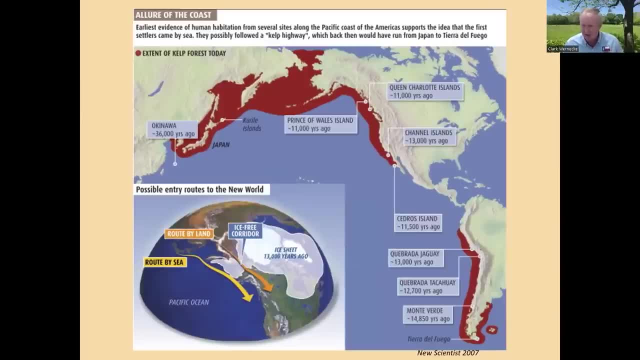 And some of the earliest human remains On Your Knees, Cave and Harlington Spring are found along the western coast. What we don't have is definitive evidence Archaeological sites that would be located on the Atlantic or Pacific coast in the Pleistocene. 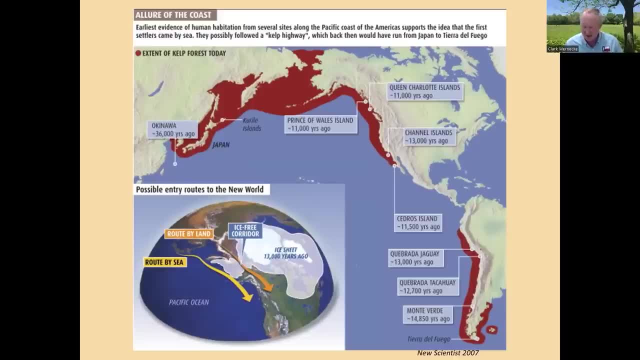 would be underwater today. One argument against any migration from the east is based on lithic analysis. There are major disagreements here, but suffice it to say not everyone sees similarities. Well, we have the same problem when we look at the west: The technologies in Alaska and Siberia. 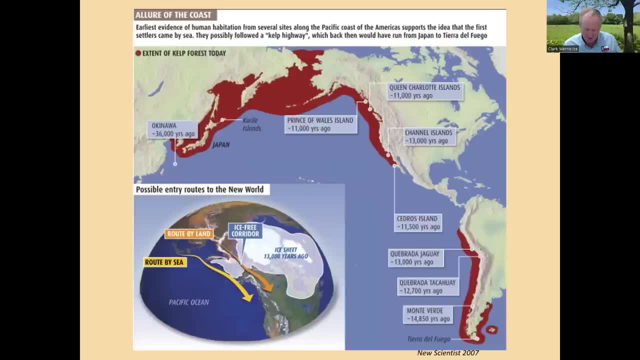 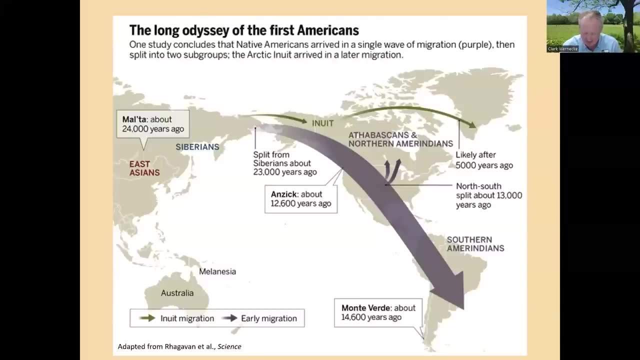 look nothing like those that appear later in the rest of the Americas. Yes, OK, you say that We get that, But didn't they figure it all out with DNA? The short answer is no. No, they haven't, And here's some of the reasons why We see a lot of graphics. 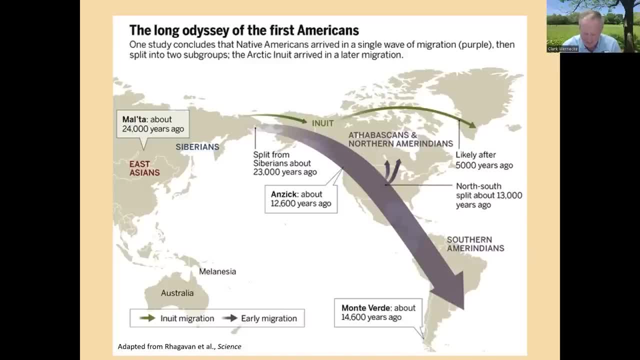 on. they make it seem pretty obvious, but they leave off all the bits that might get in the way. For instance, there was an early migration all the way to Greenland around 4,500 years ago and a later migration by people not genetically related. This graphic simplifies it by ignoring. 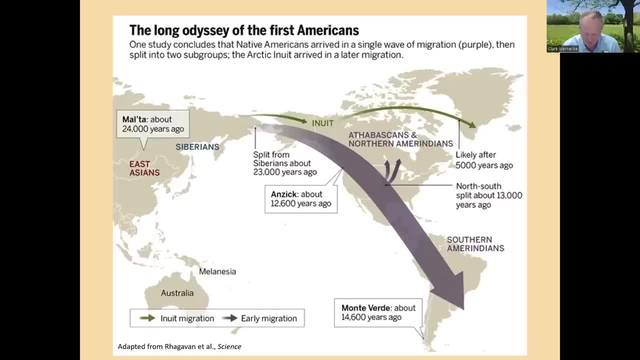 that and making it one migration. It's important to remember that the peopling of the new world again was a process, not an event, And as a process it's likely to be complex. One of the problems we run into is that genetically dating something is filled with. 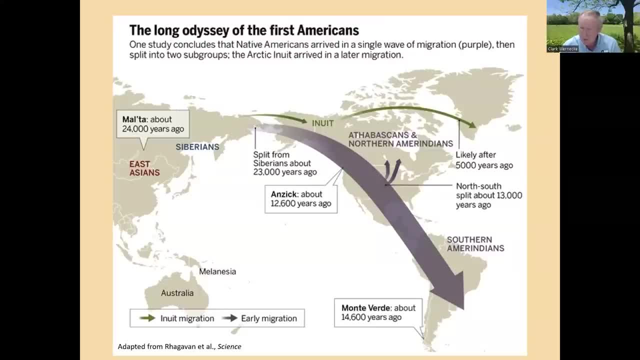 assumptions, How long a generation is, what the mutation rate was, and that makes it a horrible yardstick. So the best thing to do for geneticists is to combine it with a culture you already know the dates of, to give you some markers along the way. Commonly they throw in the child burial. 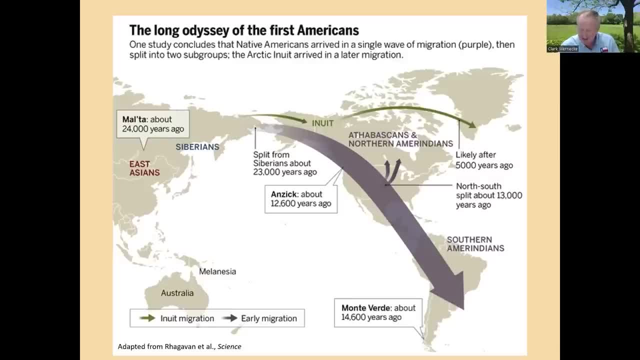 at Anzac, as they do here, and say that they're not genetically related. That burial was found with Clovis artifacts and therefore Anzac is representative of Clovis. Unfortunately, the first archaeologist to visit the Anzac site Dee Taylor, a professor at the. 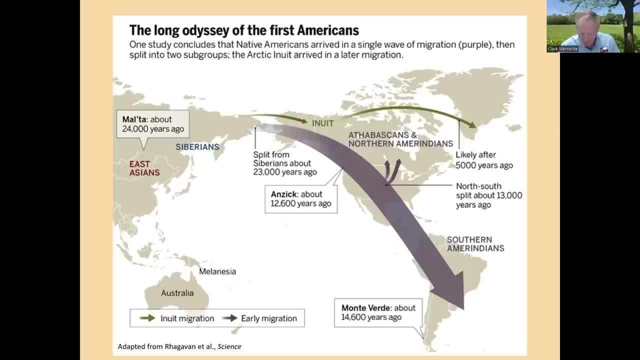 University of Montana wrote of the site. quote: the material was unearthed in such a way that data from several levels could have become thoroughly mixed. Now we can never actually prove that artifacts and bones were definitely associated together in this site. The geneticists who have been using this just took later archaeologists' assurances that they 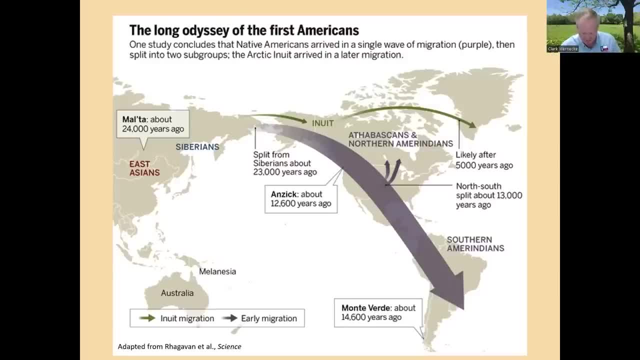 were associated, And there are some dating problems at the Anzac site as well that you could read up on your own. So Anzac is not demonstrably Clovis, And I'm sure we could all agree that one person's DNA is representative of everyone who lived at the time right. 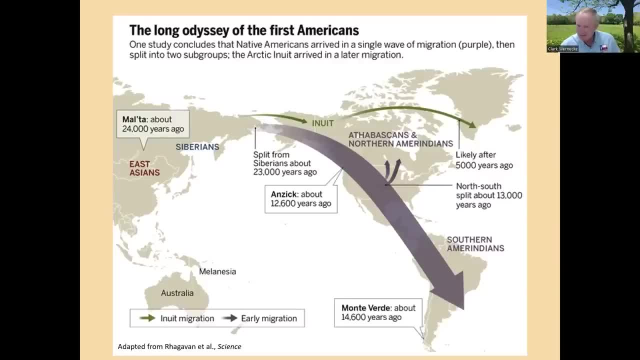 Wait, what Now? that doesn't make sense. I got my DNA done and sure as heck doesn't tell me where my neighbor's from, does it? Well, what about Clovis? This technology we have assumed represented the First Peoples and the Americans. 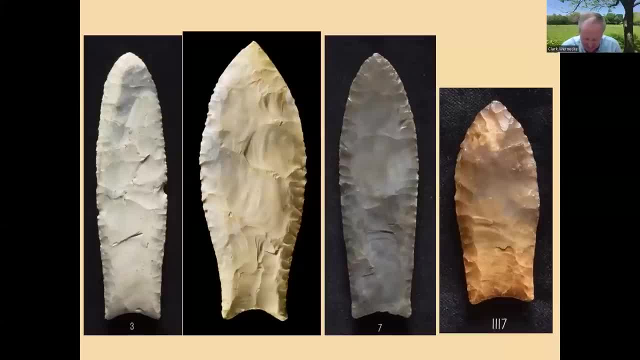 Anthropologically, the Clovis culture doesn't make a lot of sense. So we're saying there are all these little regional cultures in the old world, no matter where you think immigrants came from. And then there's this monolithic culture from Canada to Venezuela for a time, And then 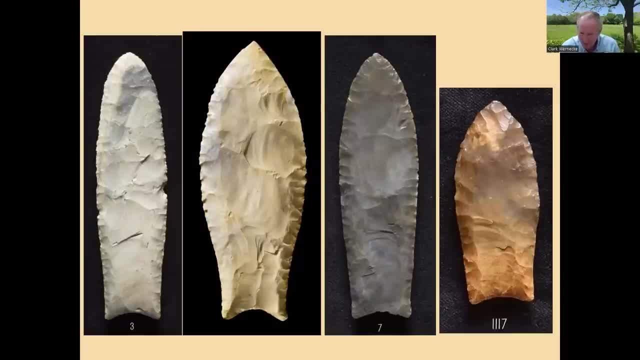 we're back to a bunch of localities, And then we're back to a bunch of localities, And then we're back to a bunch of little regional cultures. We've also long recognized, but not spoken about much, the regional variations that we see both in the assemblages from this time, as well as the 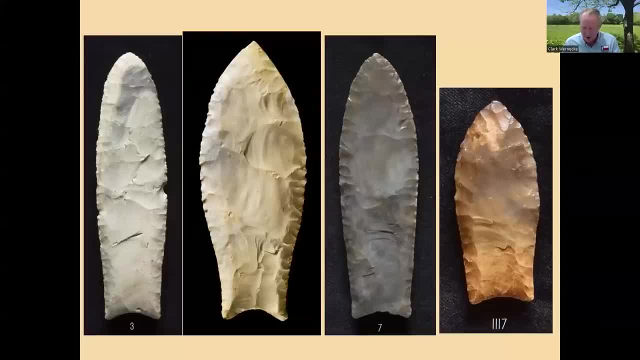 supposedly diagnostic points. We've long talked about Western fluted points and the Eastern fluted tradition that certainly have some general technological and morphological similarities, but they're not the same. These pictured here are all Clovis points from Texas And they certainly look quite different and they're actually made differently. 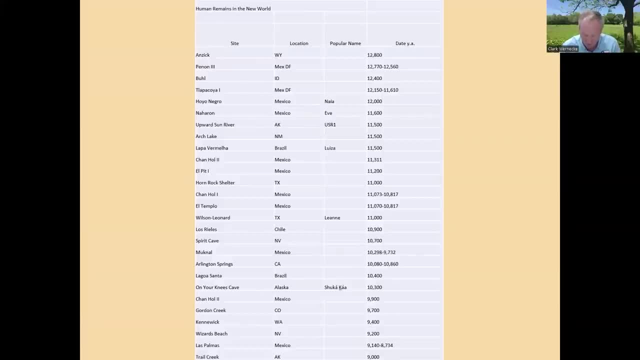 We also don't have much genetic material to work with. I'm sure I missed some here, but here are 27 sets of remains older than 9,000 years, And the oldest are probably 10 to 15,000 years younger than the first immigrants. There are estimates as high as 40 million deaths in 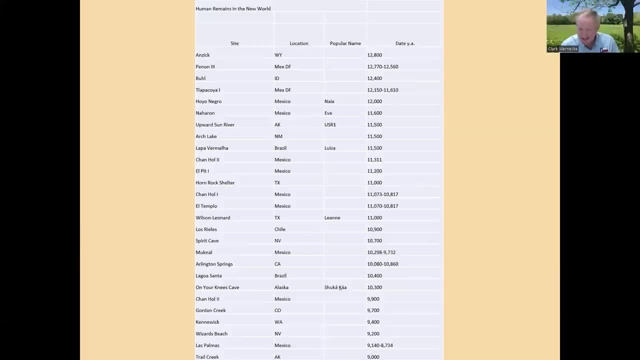 the new world after the arrival of the Spanish. That's a lot of misguidance And we do have a lot of data on how the population over the centuries has evolved. over the last and even 20 years- The first of these studies- we don't have as much data on the population. 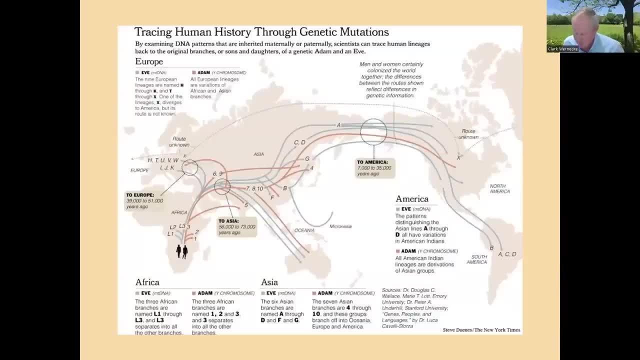 in the 1840s as we do in the early 1850s. but this is indeed a lot of information. The last one is the question of how much population we have. today. farms of a variety of species are present in all of our communities, And then you can compete with. 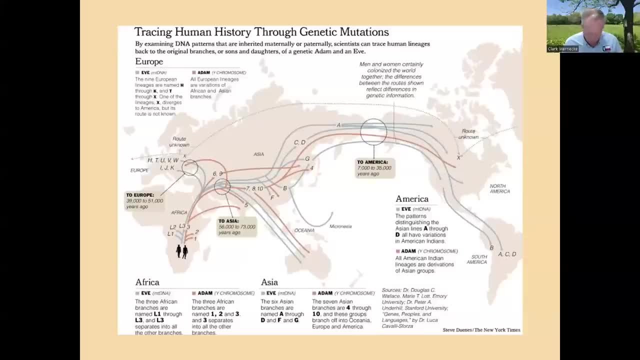 any thing other than animals, even ants. We can also see that in even animals, So we can get an idea in this map. This is the X haplogroup which is found most frequently in Europe and Eastern North America. Some years ago there were publications saying: oh, we fixed this. X and the First Peoples of 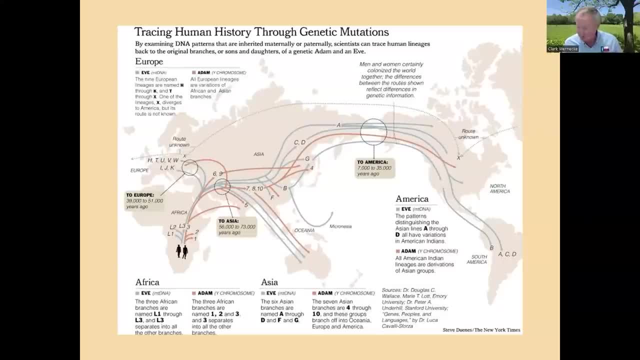 the Americas came from the area of the Altai Mountains, northwestern Mongolia, and we find it in populations there. The problem is is that the X haplogroup in the Altai is only about 9,000 years old and Mongolia is still a long ways from the New World. Here's a recent publication. 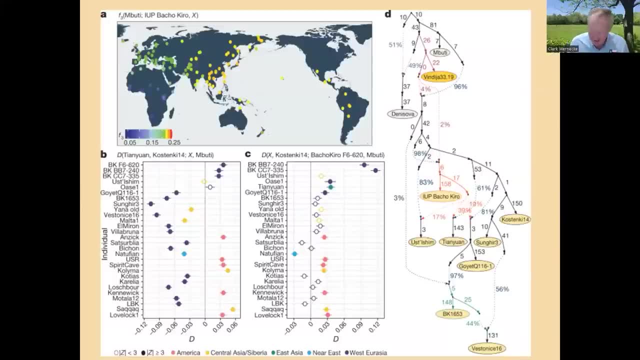 looking at a different aspect of DNA shared alleles In three skeletons 42,000 to 45,000 years old in Bulgaria. The warmer the color on the map, the more shared genetic drift. Some of these skeletons in Bulgaria are closer to Native Americans than they are to individuals. 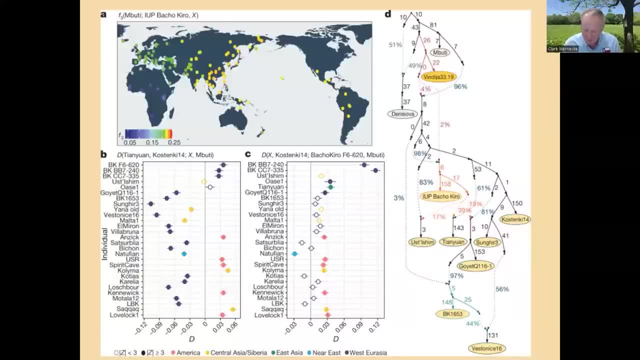 from Central Asia. By the way, the population of Europe has been replaced at least three times in the last 14,000 years, so there's a lot of problems, not just in the Altai Mountains, with comparing modern to ancient populations. We only mapped the human genome in 2003, and great strides have been made. 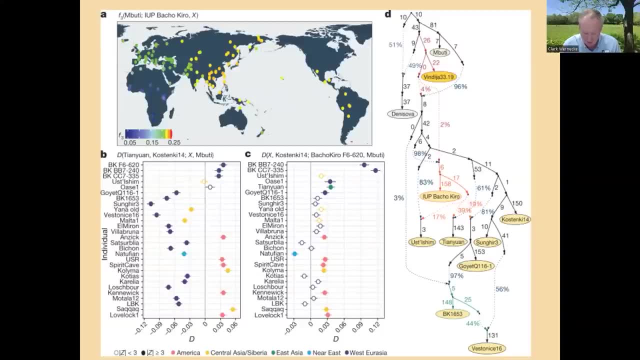 in understanding it, but there's still a lot of things we don't know. There's some really great people sequencing ancient samples, but we have a limited sample of ancient DNA. Molecular divergence can precede population divergence. We're missing a lot of lineages. 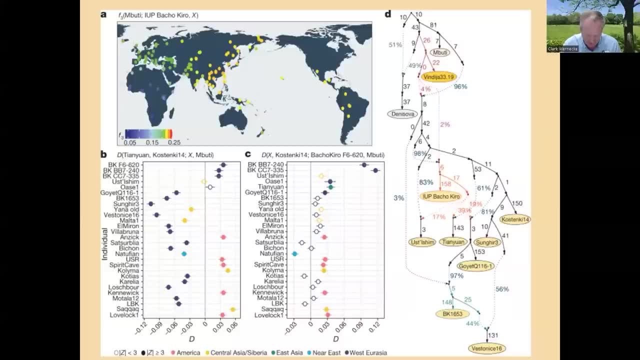 We're assuming genetically distinctive source populations. We're assuming that individuals are representative of a population. We're assuming that instantaneous change happens with no subsequent gene flow. Mutation rates are based on little data. The average generational age is based on little data Recombination, And then we also need to understand that there's a lot of data that's. 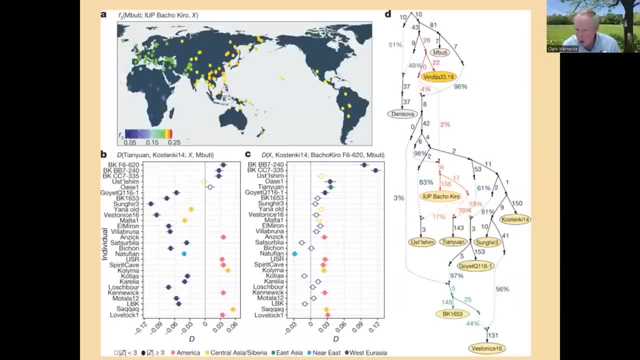 going on. We also need to assume that populations are panmictic, meaning that all individual pairs are equally likely to mate. In other words, there's still a lot to sort out. I'm sure perhaps in my lifetime they'll get a lot better data. 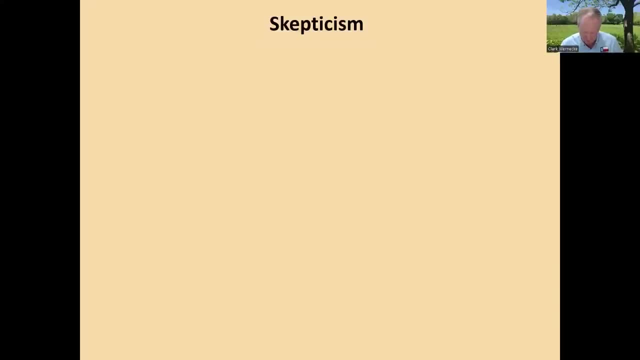 Most importantly, what you should take home from today's talk is heightened skepticism. Skepticism is healthy and it's part of science. Watch the language. There are code words that should wave large red flags in your head, and the following examples are all from recent publication. 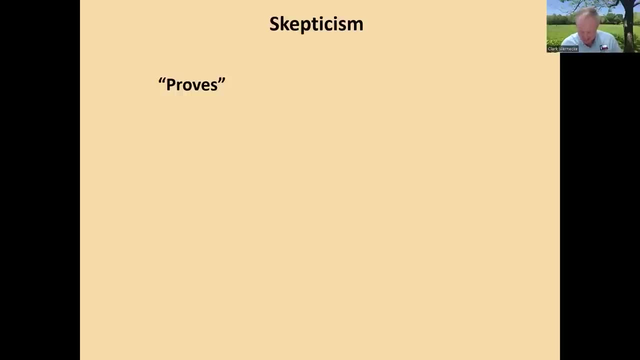 I like this one. This study proves or we prove. the scientific method does not prove things. We try to disprove them and then, even if much of our data might suggest that something is otherwise, prove is a very good idea, definitive word. I really like this one. Conclusively shows Really Beyond a shadow. 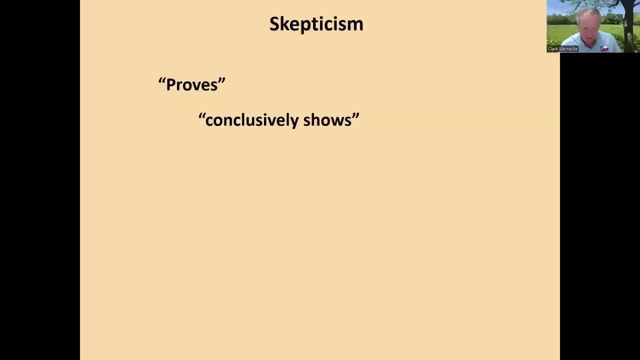 of a doubt Conclusively shows Does not support Okay. on the surface this might seem okay, but it's a real weasel phrase here. Lots of things don't support a hypothesis. The dirt on my shoe does not support the hypothesis that the ozone layer of our atmosphere has been depleted. Nope. 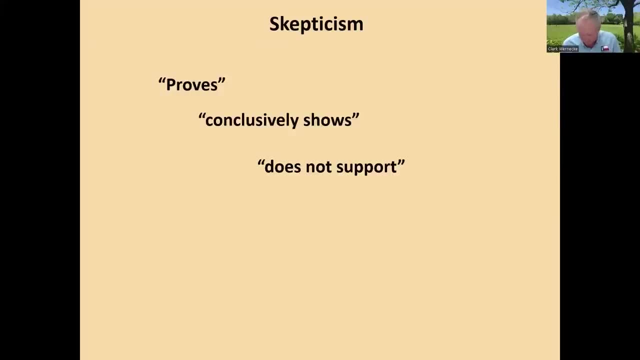 You know it does not, but so what? There's a lot of things that don't support things. Refutes the possibility. Oh, this is reserved for when you have a real ax to grind with a colleague. This is not only wrong. it's impossible for it to ever be right When you see phrases like this. 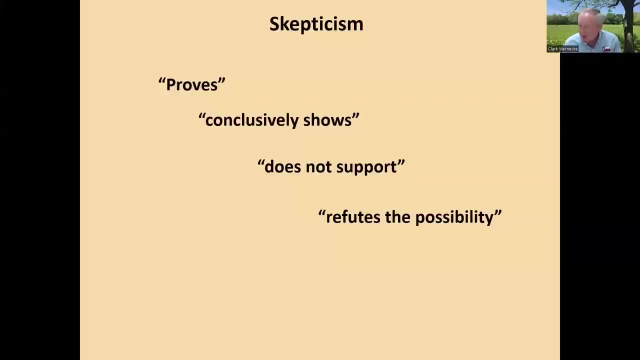 I want you to think of me using my most sarcastic tone and going really Really. So read these things and then start thinking about it. What we have now is enough data to say: there seems to be an awful lot of smoke, so we really ought to watch out for the fire. 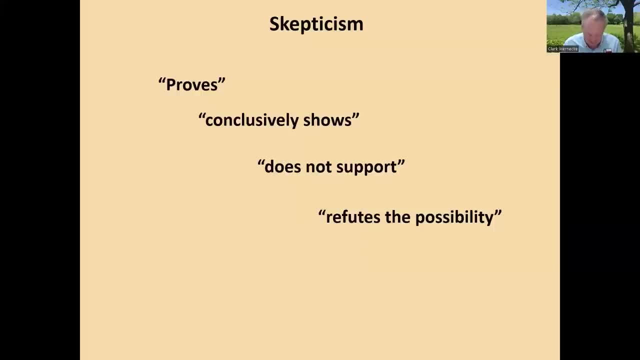 I'm sure my listeners in the West know that that one's a really important one. We have no definitive answers right now, but we have lots of indications that the old hypotheses don't work. Just like we rejected people being here only 4,000 years ago, it's time to let go of 13,500 years ago as well. 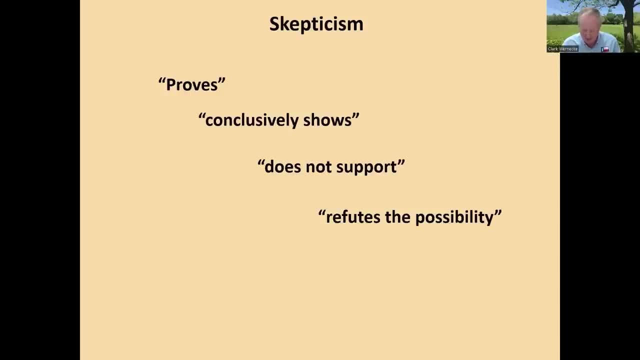 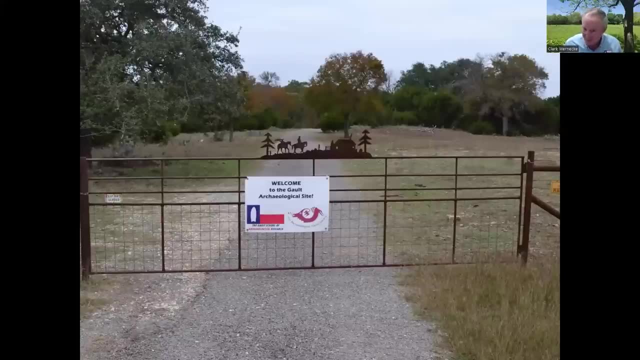 and look for more data and test new hypotheses. So again with that, my thanks to the Conservancy for inviting me back and for all of you for joining me tonight. I'm going to try to answer some of your questions to the best of my ability. 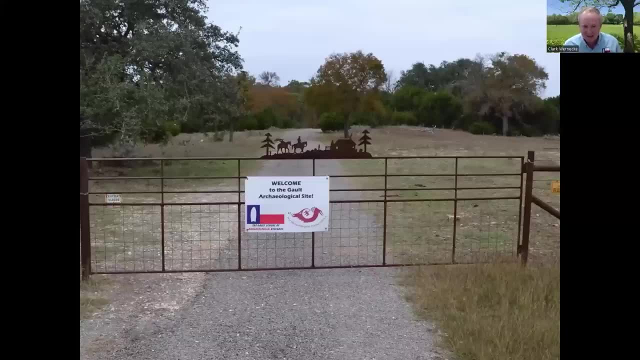 but I'm going to remind you again, I'm an idiot. So give it your best shot and we'll see you next time And we'll see if we can answer some of these. That was great, Clark, Thank you. There's your graduate seminar, minus some stuff. 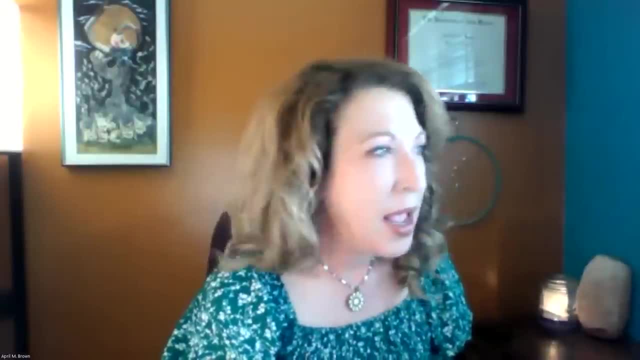 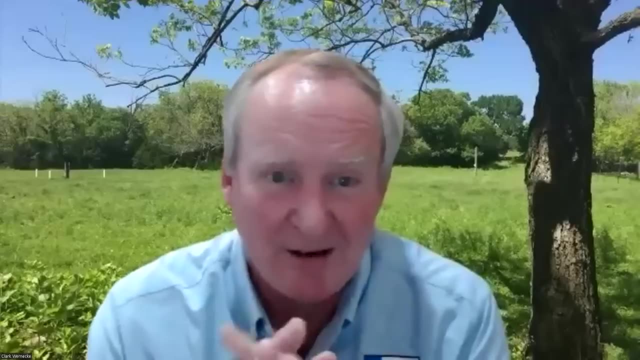 Okay, we have a handful of questions, Just a handful, Just a handful. right now We'll see how that goes, But we have like five, 10 minutes tops anyway. so, All right, We went a long time. That's good stuff. 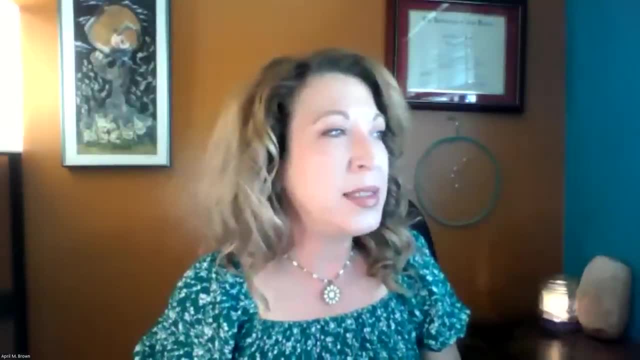 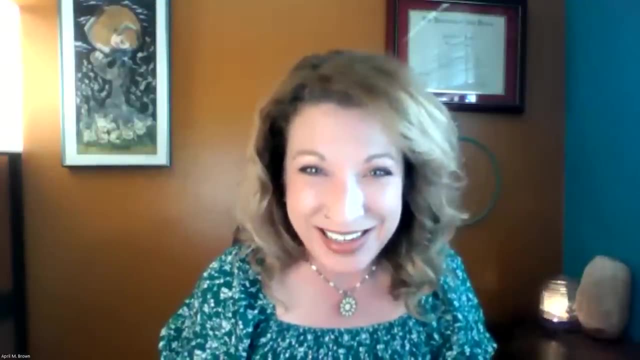 No, it was fantastic. So one of the questions was: someone asked: how can you, how can you, establish that an artifact is unquestionably human made? Oh boy, That's something I almost have to show you rather than tell you. 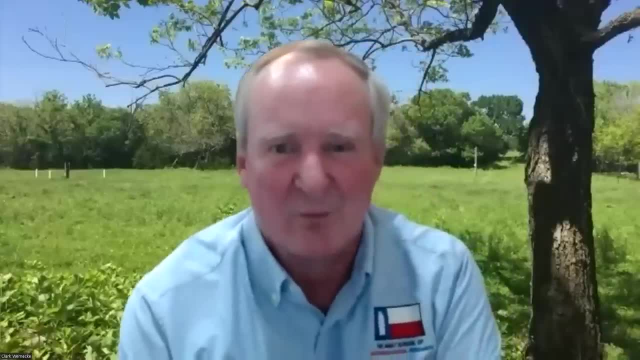 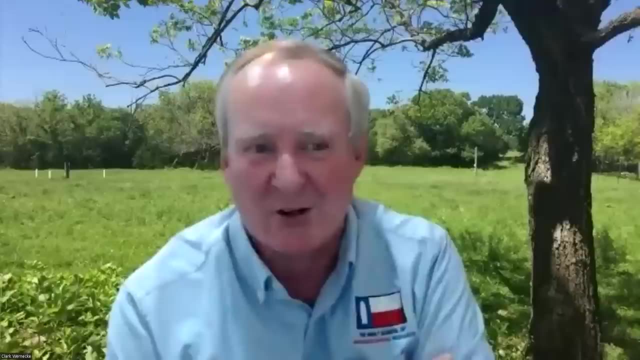 You know, when you find a sharpened stake with rope tied on it, I think we can agree that's human made. Most stone tools. we can actually show you, through lithic analysis, exactly how it was made And you know they're. they're more complex, They're more complex, They're more. 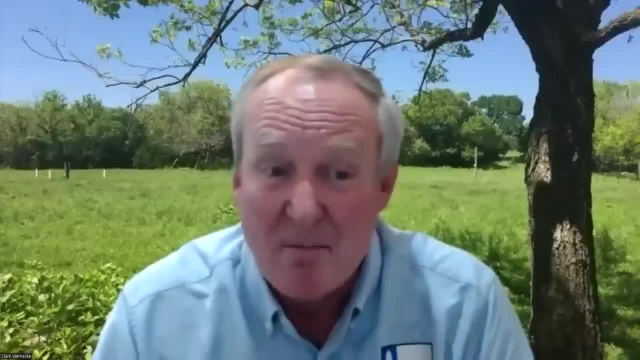 complex than can happen other ways. I mean, nature can mimic some stone tools sometimes, but you find a whole lot of them. they're human made. There's a lot of things like that that you really have to look at the stuff in the lab to be able to definitively tell you why. 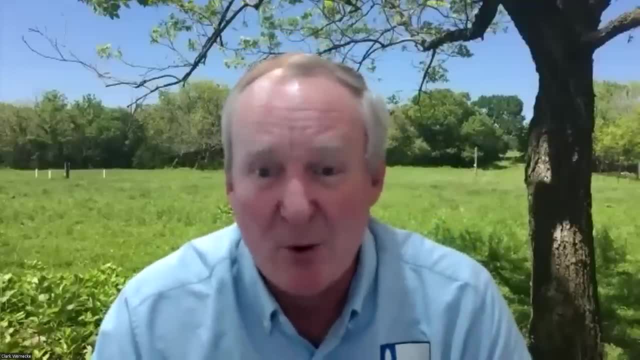 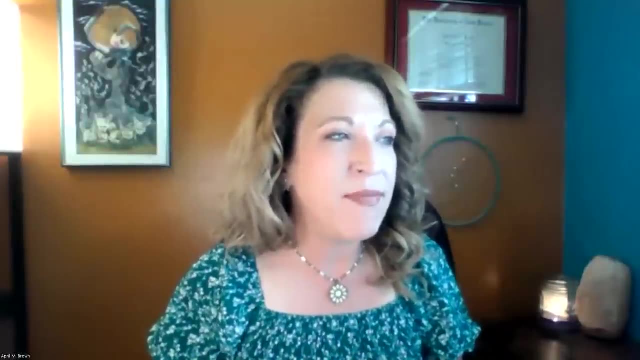 we think they're human made, But a lot of them are pretty obvious to most of us, Okay. Another question is: how is it determined that phosphates identified at Meadowcrofts are not Okay? I don't know. I don't know. 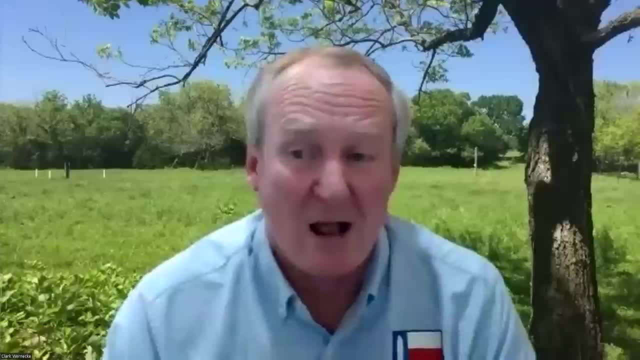 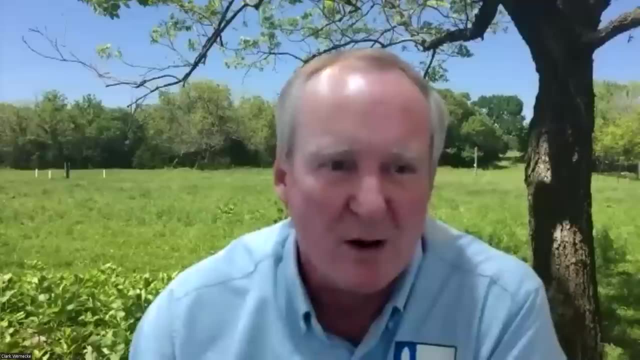 Okay, I don't know, I don't know other mammal. Well, as I understand it, the phosphates and phosphorus and stuff basically come from human activity areas. I may be wrong in that. Again, I have a soil scientist that I'm. 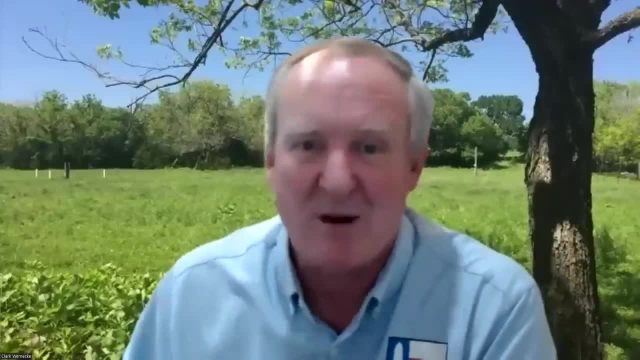 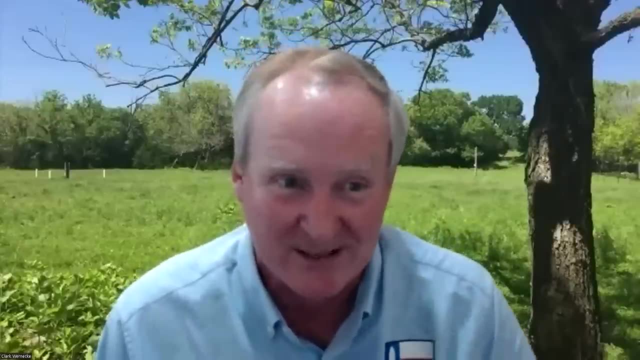 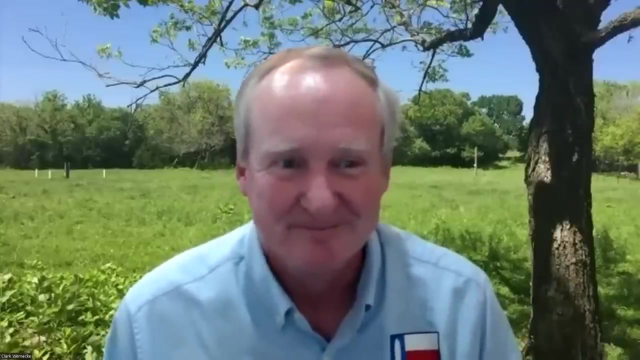 working with right now. I knew of about three of the tests that I wanted done on soil samples. He sent me a list of 23, and I have no idea what the other ones do, So I have to sit down with him and go through it. It's not a question I can answer. well, I'm an idiot. 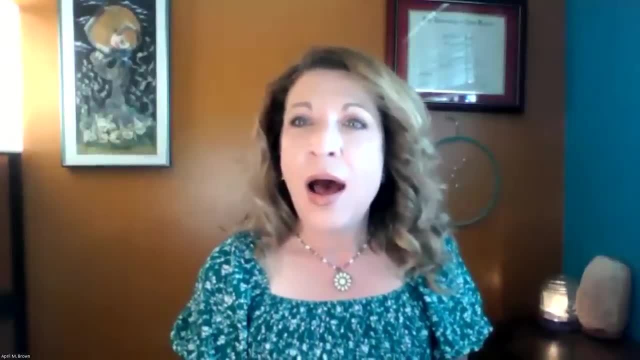 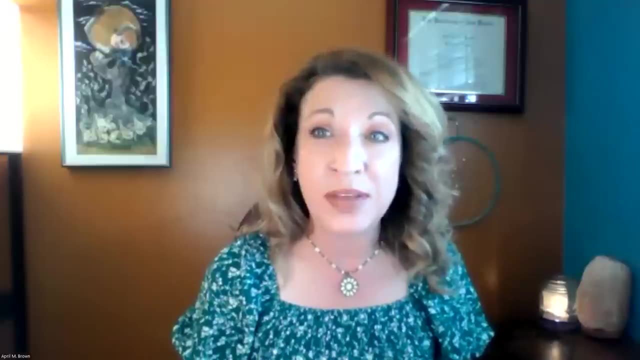 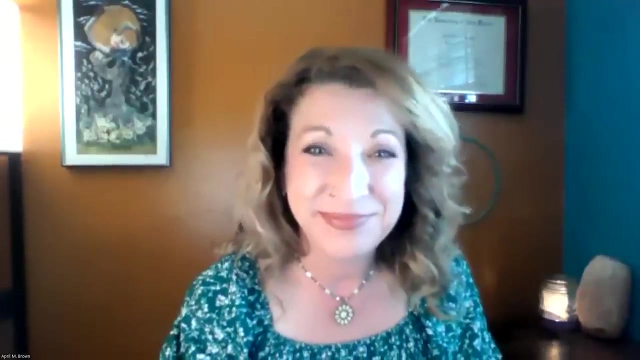 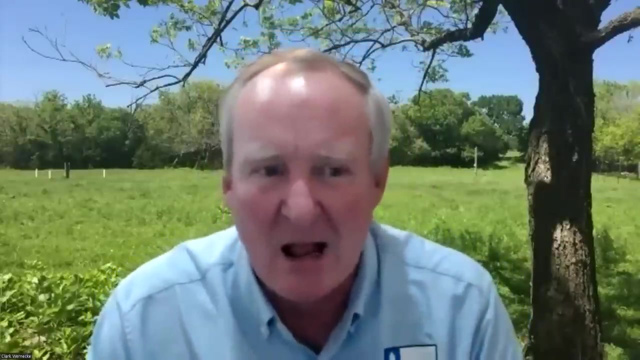 Okay, Let's see here The next question. Patricia says she read an article a while back proposing that the diversity of indigenous languages along the Pacific coast supports the theory of migration along the West Coast. What do you think? Ah, it can support one hypothesis. Yeah, Although it depends on how you look at that diversity. 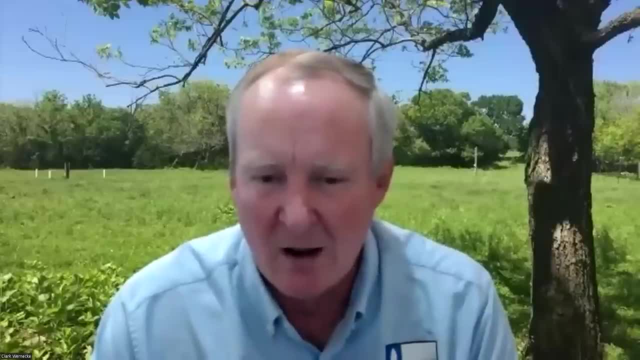 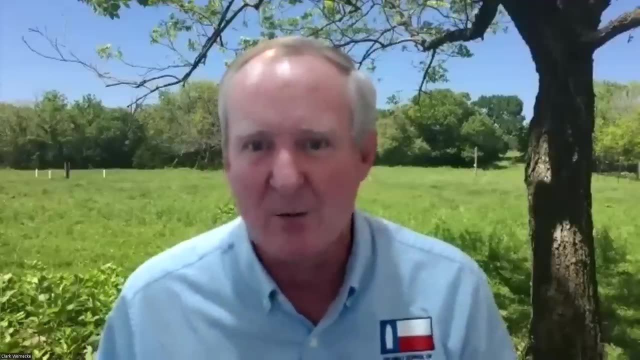 Again, linguistics is not my field, but when you look at that stuff, there's a lot of discussions about how to examine diversity in languages And I don't know that actually there's a definitive answer there. even in their field, Linguists don't all agree on that. 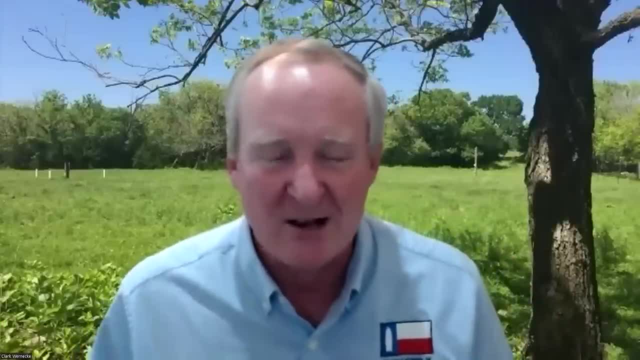 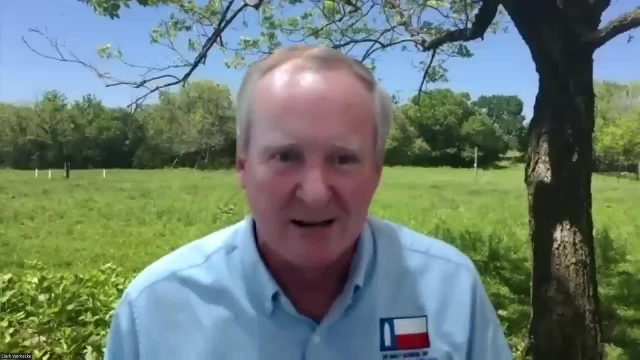 The old linguistic evidence that everybody thought, oh, that's going to support the Clovis thing. And for years people have been punching holes in that and saying, well, this doesn't work and this doesn't work And it was poorly done. So I'm not sure that we have a definitive way. 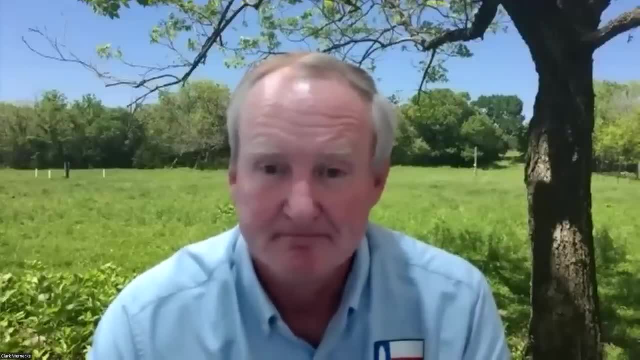 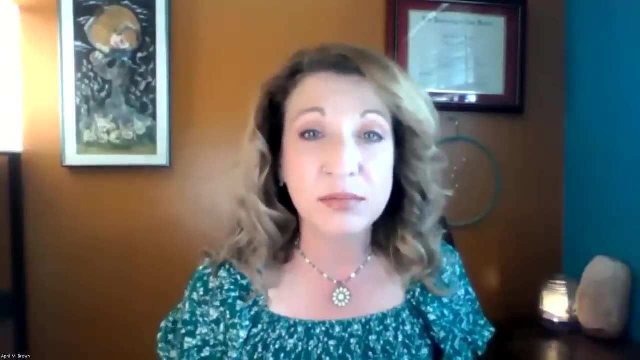 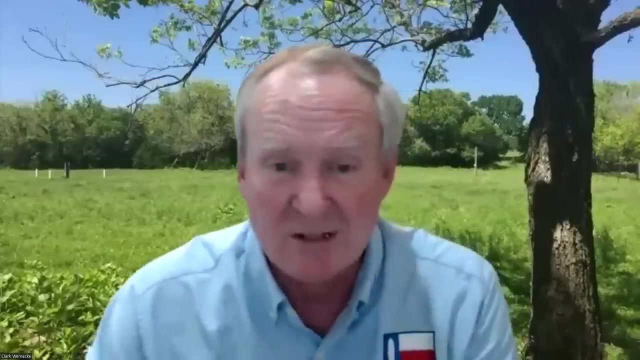 of saying that with linguistics. We have another person who asked what is the oldest secure date from the Galt site so far. The oldest secure date? Well, human date is around 18,000.. You can see our Science Advances article. It's open source. So if you go to Science Advances, 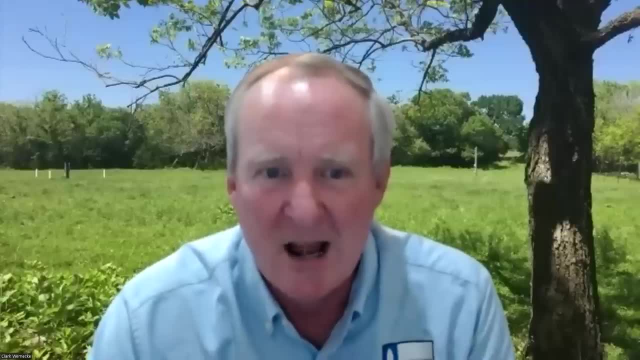 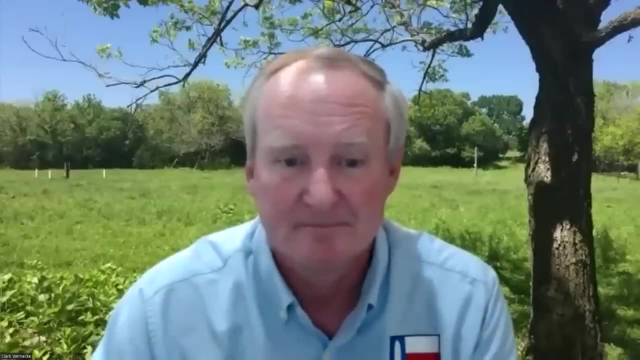 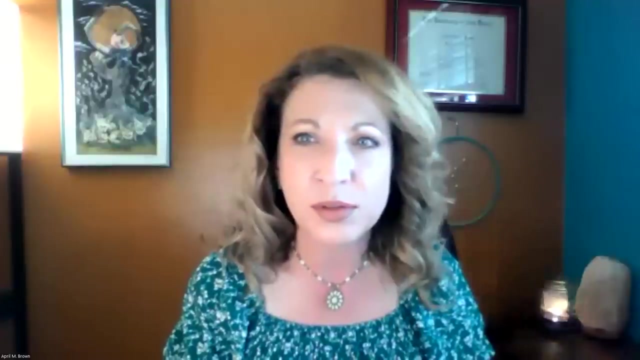 and just put Galt in the search thing, it'll come up and you can read the information about the dating of the site. Okay, Someone asked: has there been any research that attributes typology of pre-Clovis tools? Will you repeat that again? 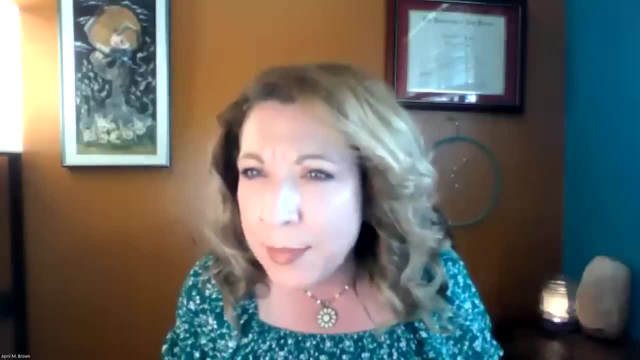 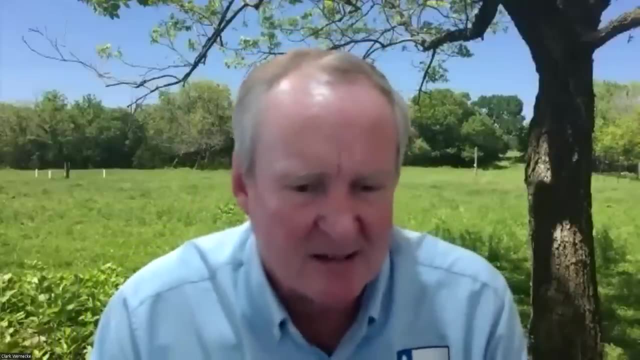 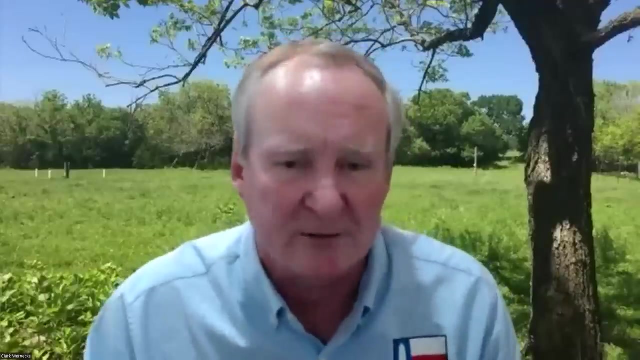 Any research that attributes typology of pre-Clovis tools. I mean, we're researching the technology of these things, But when you're talking typology again you're talking about patterns And I can't compare, say, stuff from Galt to Monteverde. 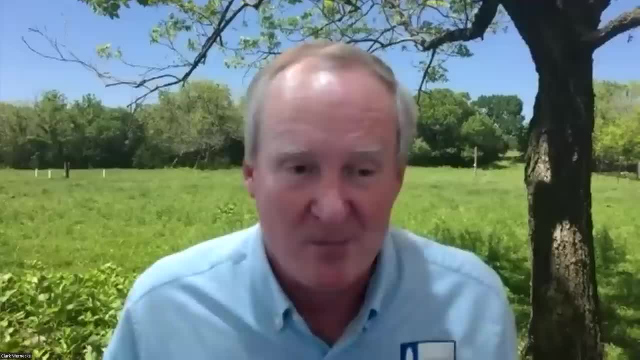 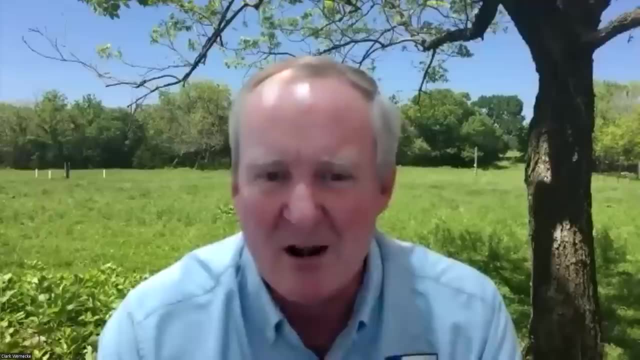 They're thousands of years apart. They're thousands of years, thousands of miles apart. Trying to compare those things is not a good idea. You need things that are nearby And that's why I noted those millipedes, And I think that's one of the similar points. It's intriguing. It's not yet definitive, But at least. 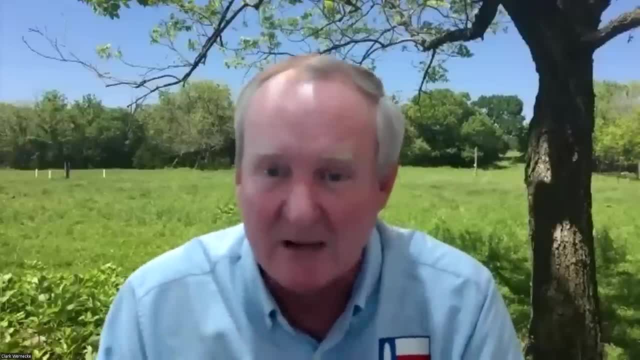 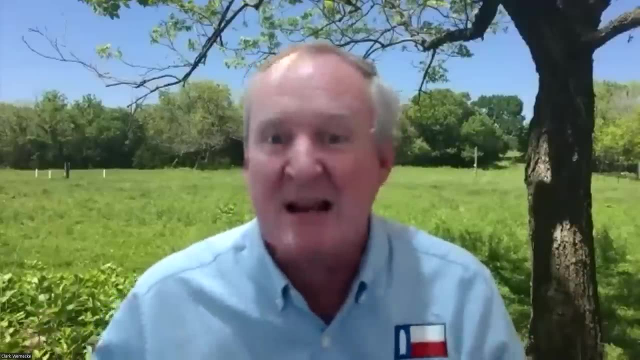 those are closer together. We're talking Delaware, Virginia, Pennsylvania. Maybe there's something there, And as we find more stuff, maybe we'll find out that we do have a typology. Maybe there is something there that we can say: hey, there's this culture and this culture, I know we got called. 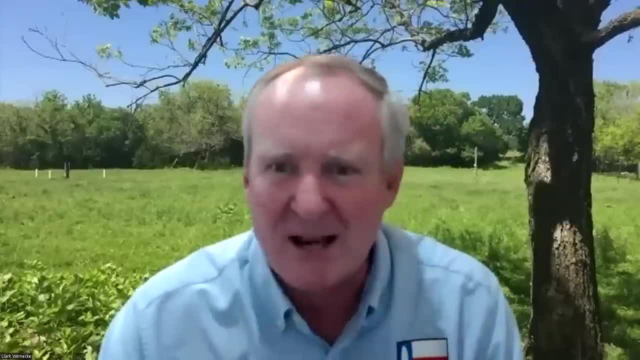 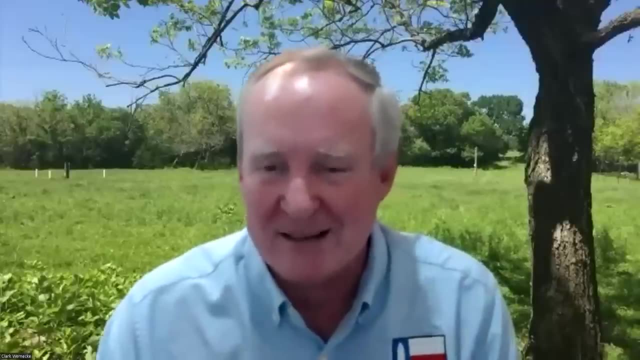 on the carpet by one person not long ago who said, in our arrogance, we're calling this the Galt assemblage. And I tried to make it really clear. We're only calling it the Galt assemblage internally because we don't have a cultural 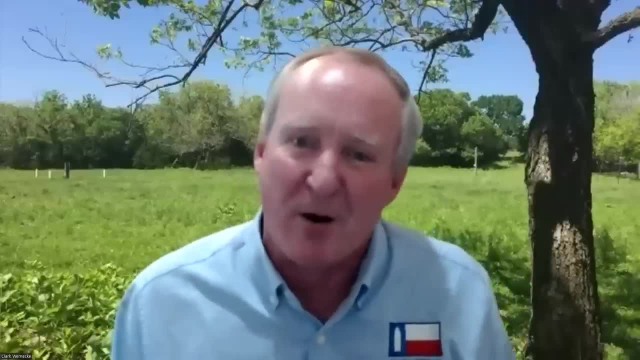 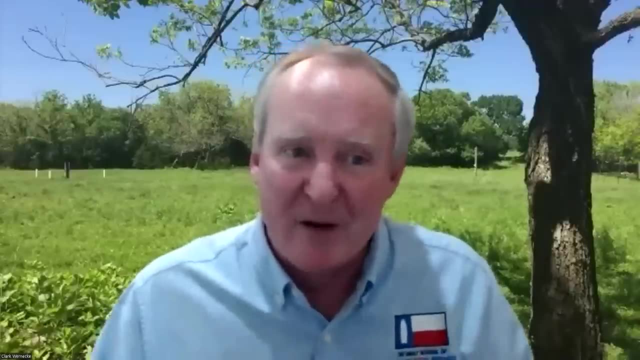 name for it And I don't have other sites in Texas to compare it to. We actually excavate 10 to 15 sites here in Texas every year looking for that comparable material, And if I can find other sites with similar dates, similar geology, similar tools, then I can start talking about. 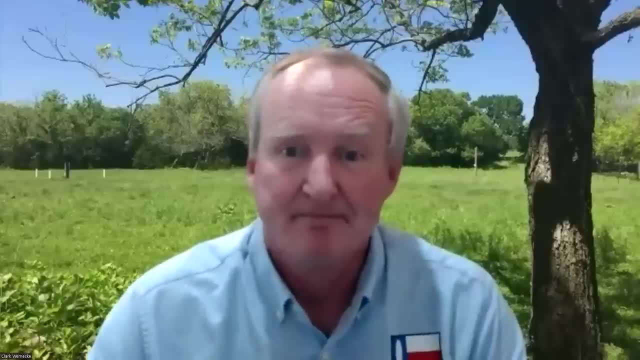 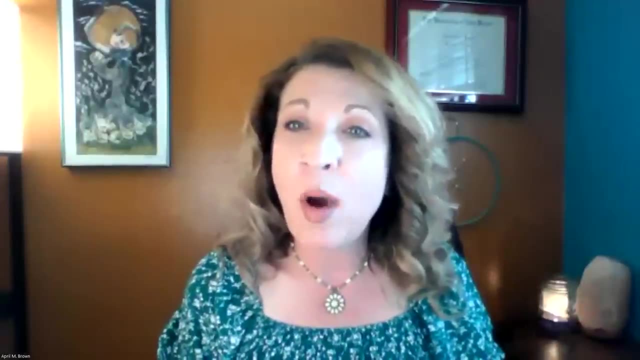 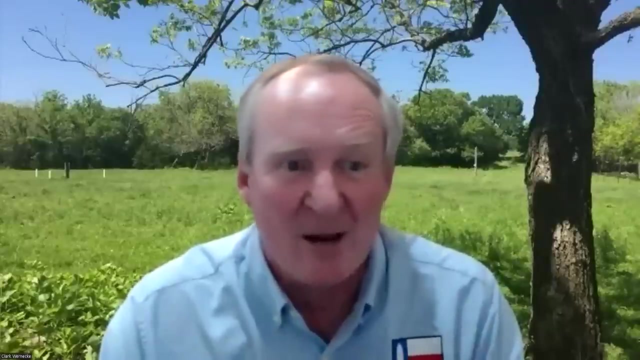 patterns And maybe we can start getting into typology. It's a good question. We have another person who asked: why do projectile plants change styles over time? Why did your appliances in your kitchen change over time? Why does your phone change every year? 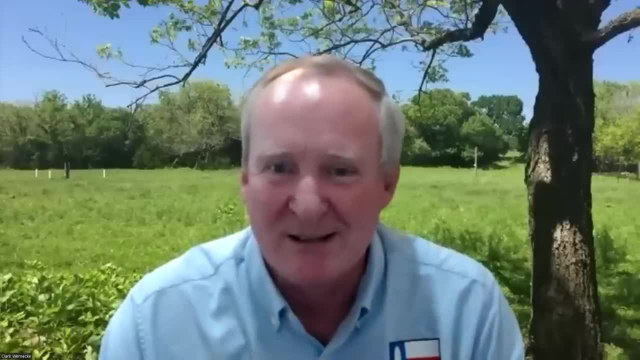 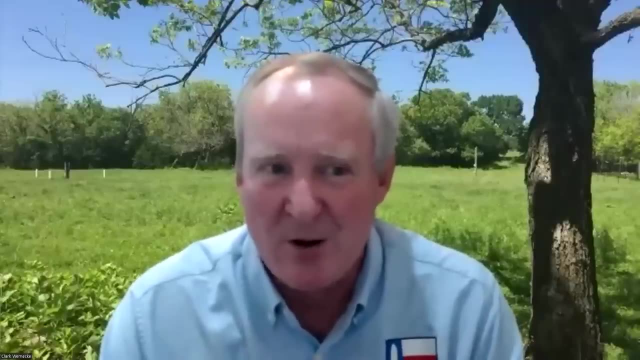 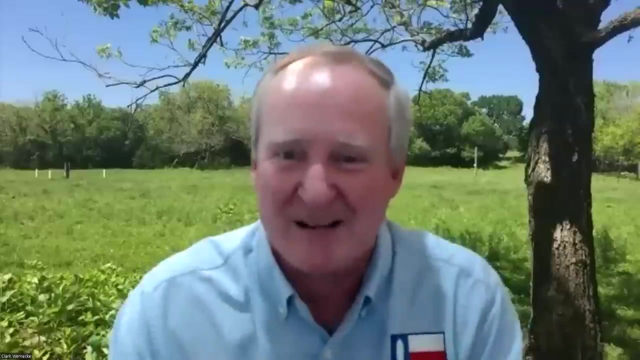 now, That's just humans being humans. The Harvest Gold dishwasher didn't work much better than the Avocado dishwasher. They were only like two years apart. There weren't vast technological changes. But suddenly we decided: eh, Avocado's out, We need Harvest Gold. And you just replace those. 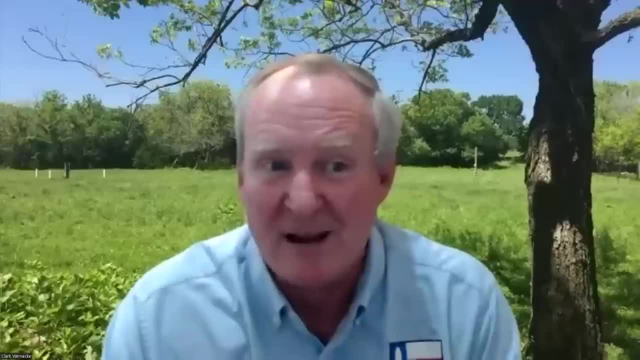 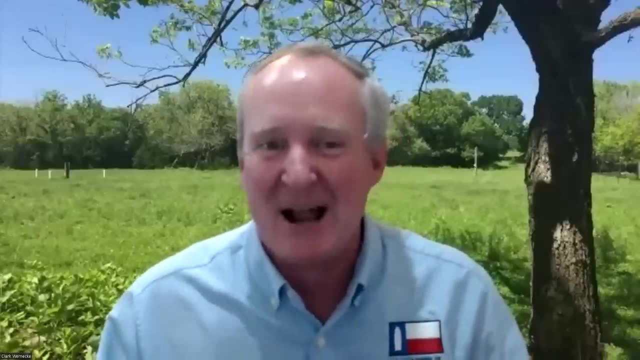 appliances. Now, nowadays it happens very, very quickly. We have instantaneous communication worldwide and trends can come and go in a week. But in the past it's a lot slower. People see something from another culture- perhaps it's traded to them or something- and go. 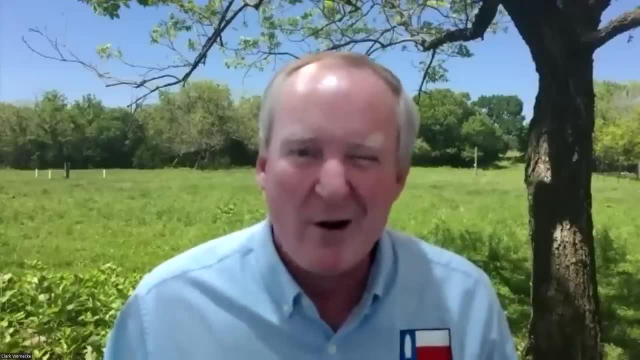 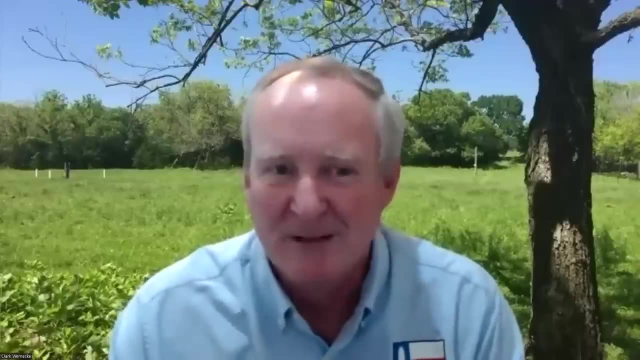 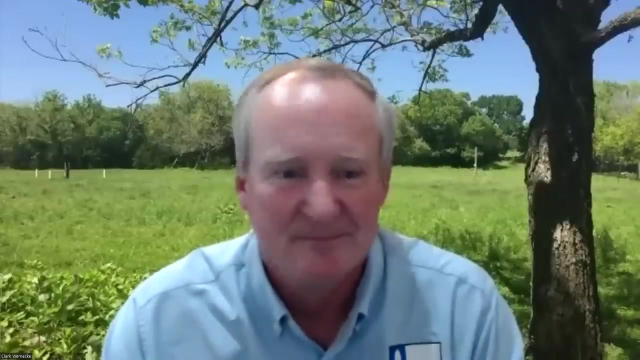 that's the coolest thing I've ever seen. I wonder how I could make one of those and start adapting something else Later on. people just start adapting different things to differentiate themselves from the other guys over the ridge. Do you have any thoughts on rock art evidence related to this time period? 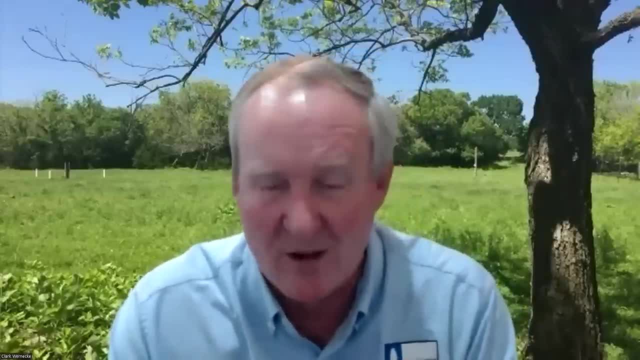 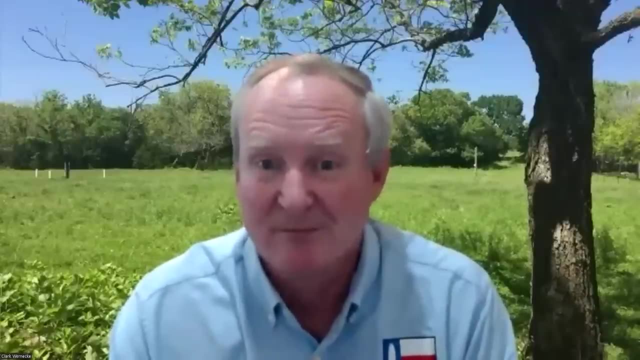 Well, Galt has incised stones, the oldest ones of which are of Clovis age, with geometric designs on it, And those are representative of the first art in the Americas. I am of the opinion that if you don't look for them, you won't find them. 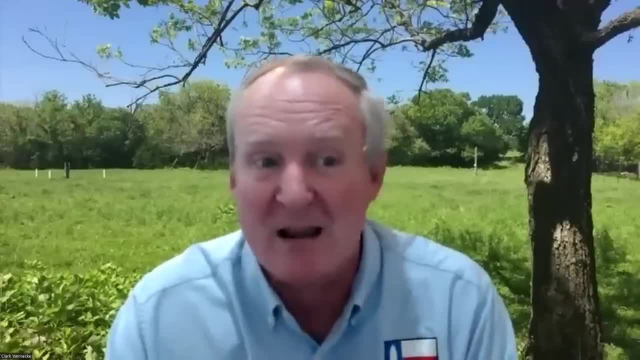 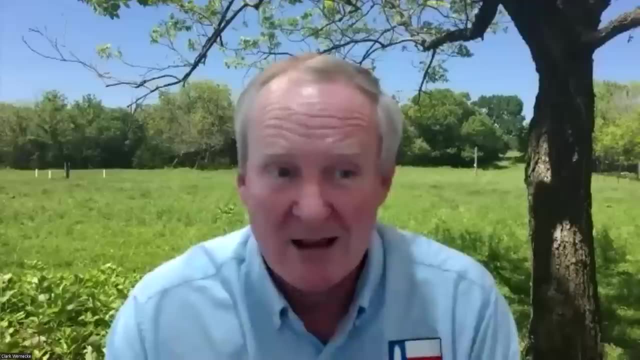 And we're finding that to be more and more true as people start finding them elsewhere, Not only in old collections. when they go back and look, we have stuff here in Texas from Kincaid Rock, Shelter of Clovis age and Wilson Leonard of Clovis age- The folks that are working. 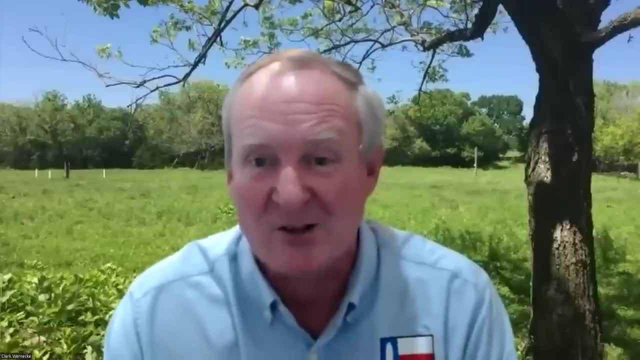 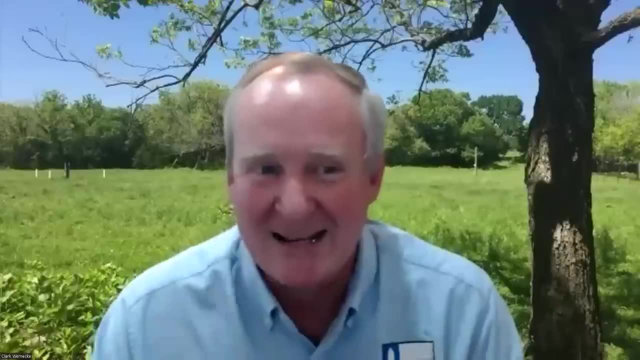 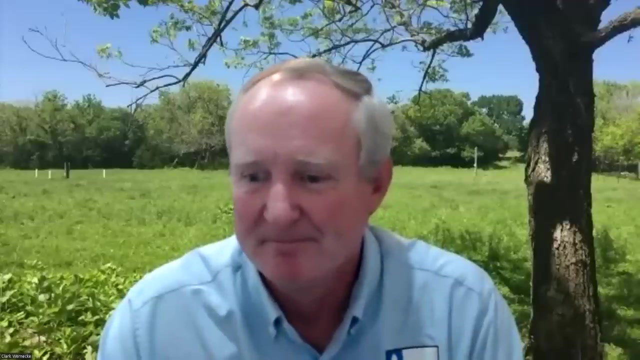 in Trinil, Indonesia, on stuff 450,000 years old, actually quoted the article we did in American Antiquity about incised stones and said, as Lemke and Wernicke said, if you don't look for it, you're not going to find it. I'm convinced we'll find even more. 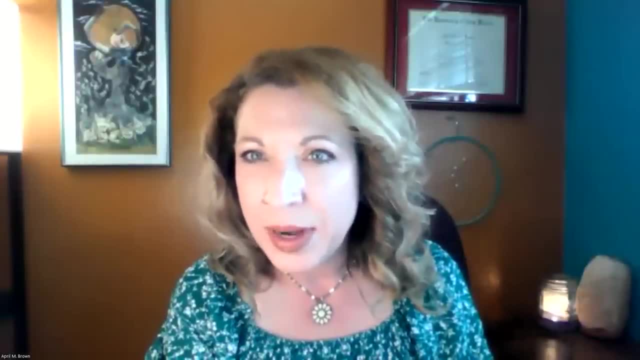 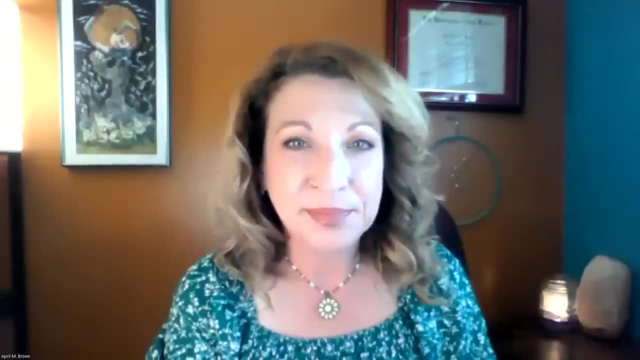 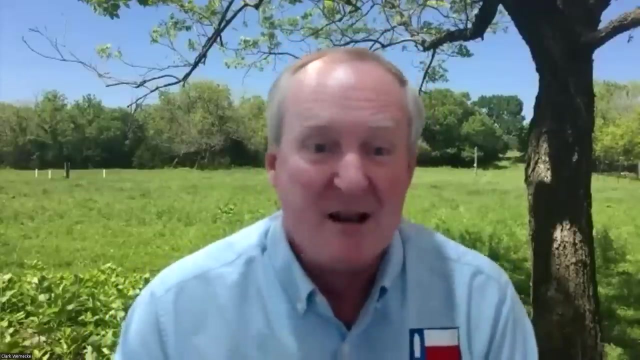 Okay, So this might be a loaded question, but I'm going to ask it. They're all loaded questions. Why did you dismiss migrations from Africa? Because we have absolutely no evidence for them whatsoever: Nothing genetically, nothing artifact, wise, nothing. Now I told you that we never say never. 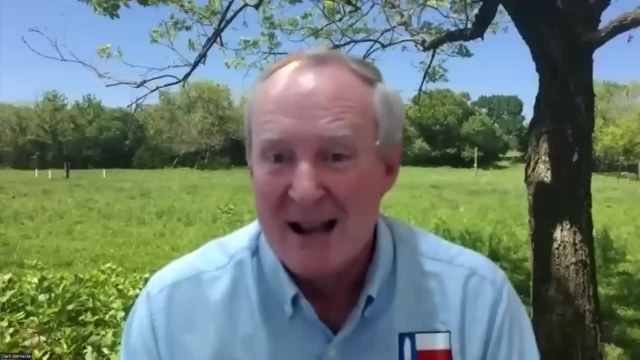 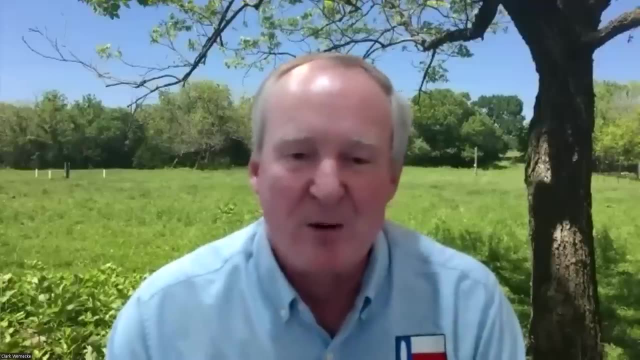 So maybe someday- I mean, there's an awful lot of archeology going on in South America- and maybe someday in Brazil they find something and go, wow, this is weird, Although you have to remember. remember, too, that you need a bunch of people. 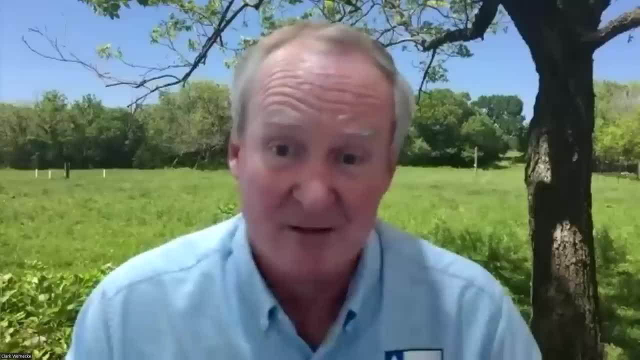 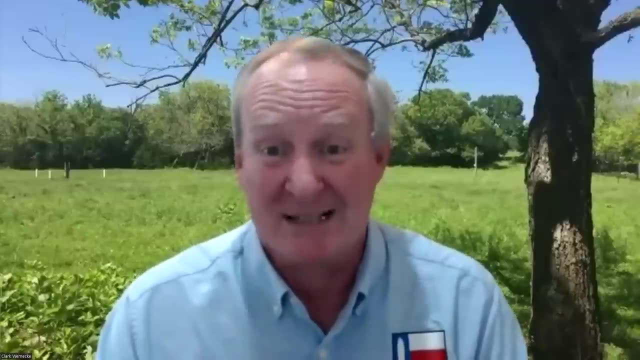 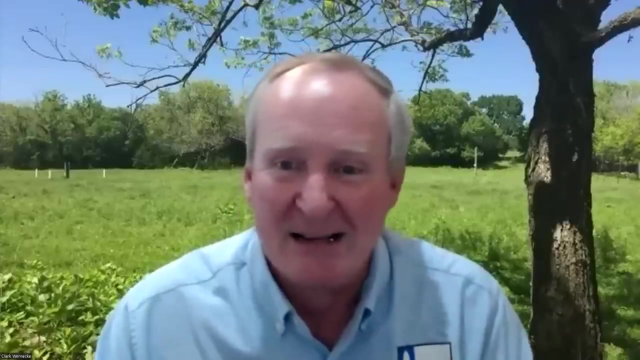 to do a migration and to have a viable population, And the fact is is that we know historically of lots of people that ended up in the new world by mistake, People that were shipwrecked here, people that were driven off course and everything. There are two guys that were shipwrecked in the 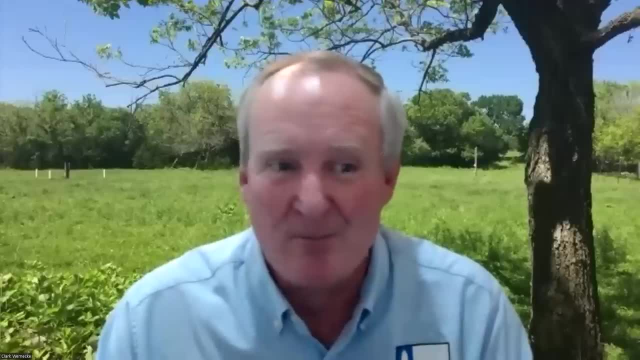 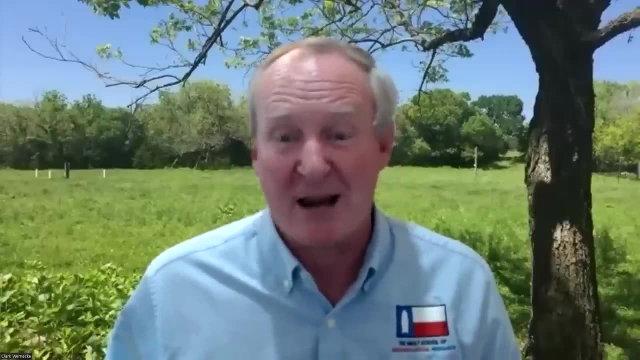 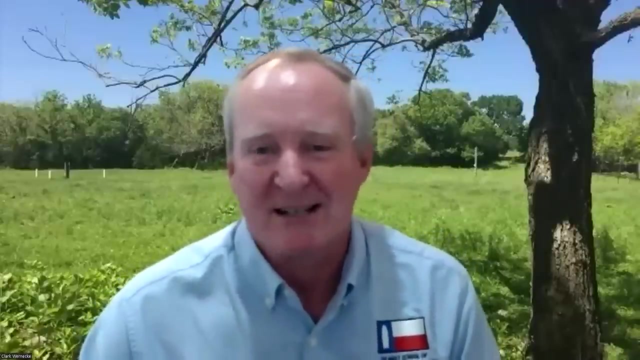 Yucatan and they were Spanish. Dave, Madison And the Maya didn't become Spanish. Those two Spanish guys became pretty Maya. One of them married the chief's daughter and became a war chief in the particular city he lived in. So yeah, you need a bunch of people and we're just not seeing any evidence. 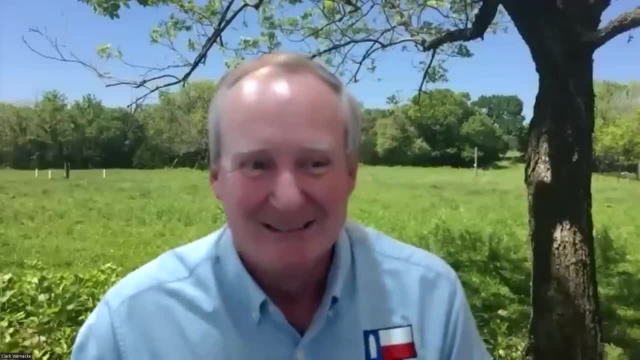 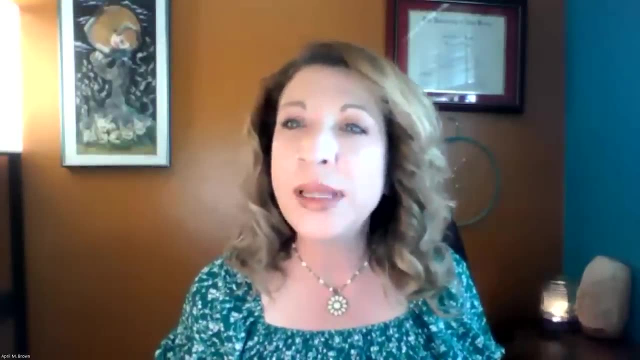 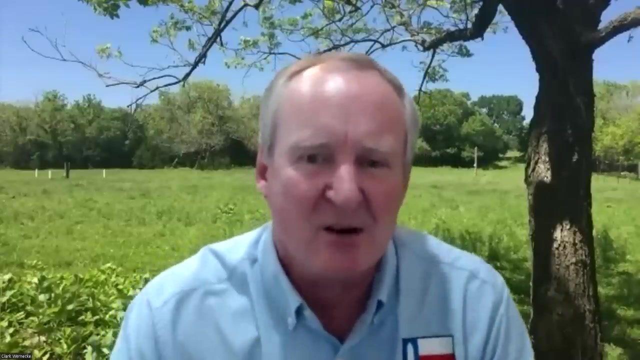 So I dismiss it now. Does the Friedkin site- I might be saying that improperly- have any comparable early material to Galt? Yes, they do. The Friedkin site has stuff that's 15,000 years old. They've also published articles on it. 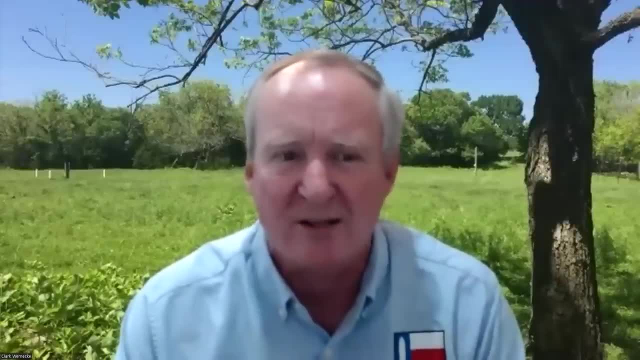 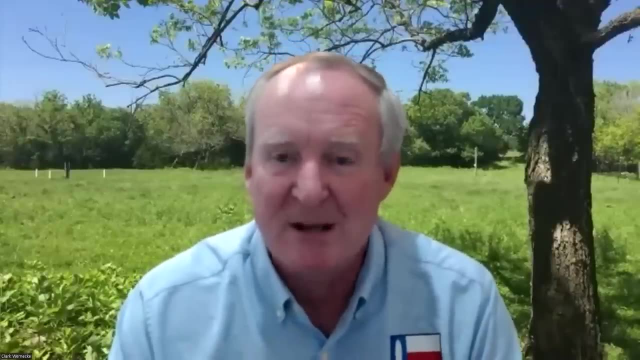 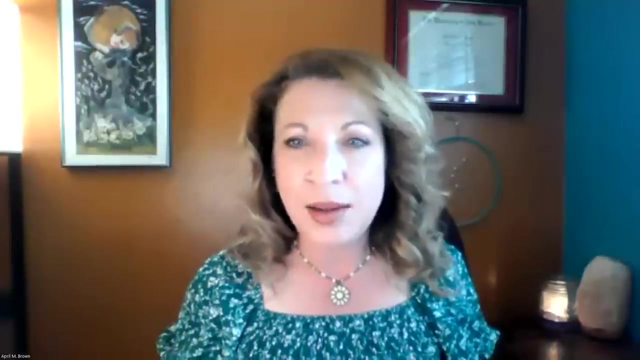 It was excavated by a group from Texas A&M who worked with us at Galt for two years and got an opportunity to work downstream from us, And they have similar stratigraphy, similar artifacts below Clovis. Okay, I think we still have a few questions, but I actually think I'm going to have to cut it off at some point. 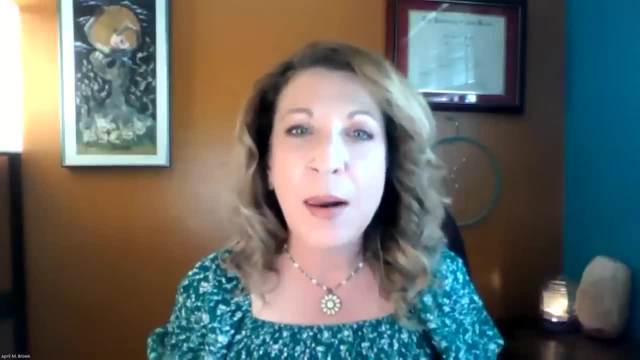 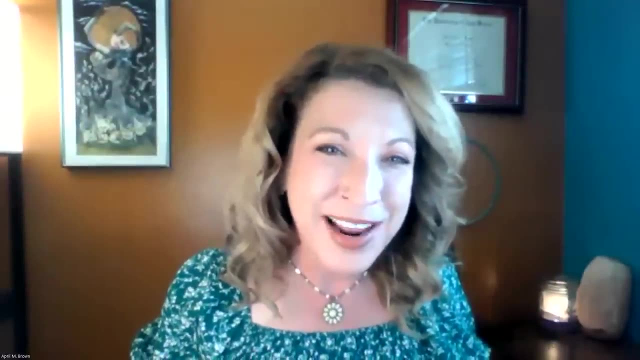 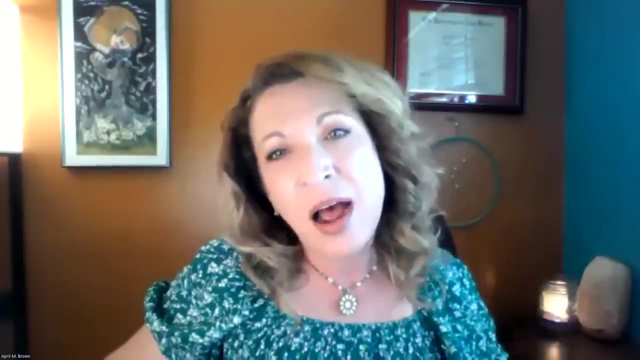 We're going over a little time here, But I'm going to somebody first of all. someone asked if you give talks on a regular basis because they love your the way you think. That was another question. And finally, the last question I'll let you cover is whether you're doing tours at the Galt site.